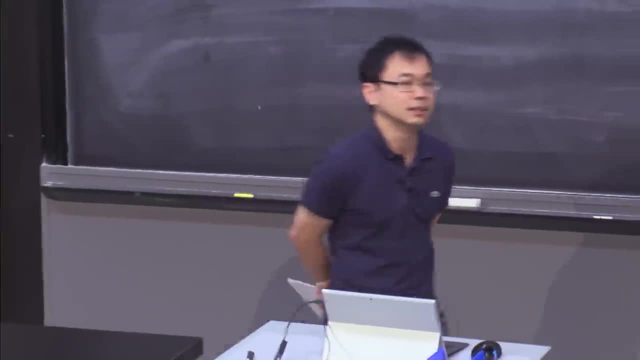 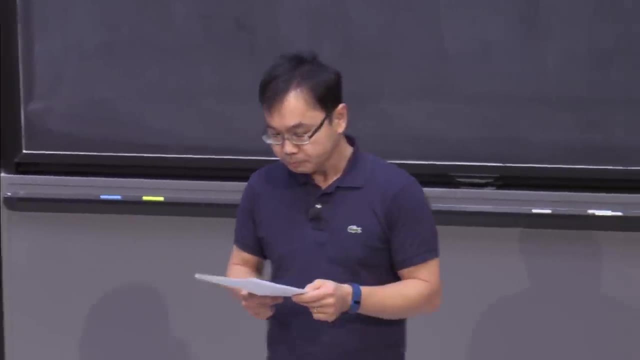 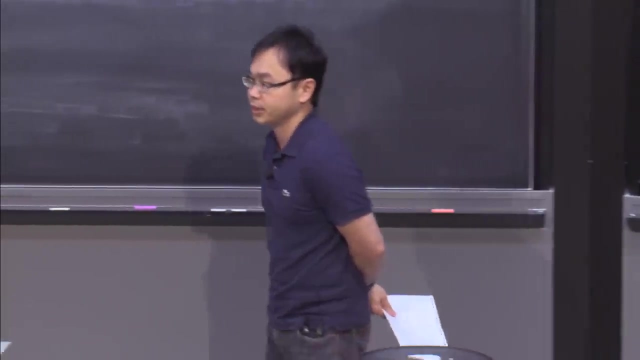 that there are three different kinds of different kinds of systems we discussed in the lecture or in the textbook. The first one is actually a string, a very long string system with constant tension and mass on this string And the behavior of this string obey wave equation. 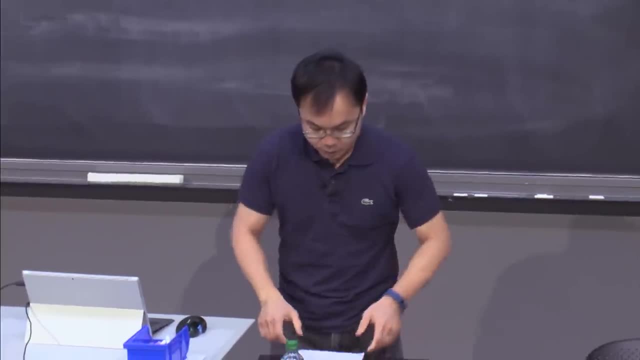 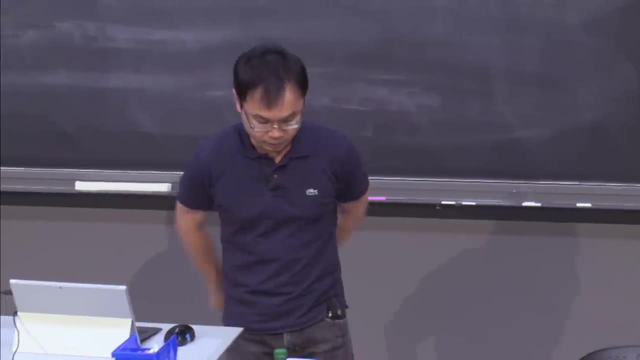 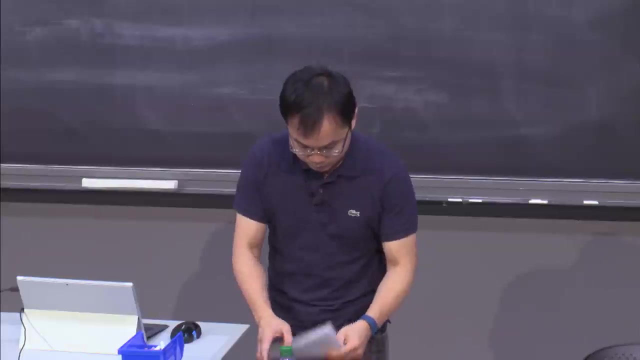 can be described by a wave equation. We also can produce a density wave with a spring And basically the wave is a string and the density wave of a spring can also be described by wave equations. So that's actually described in the textbook. 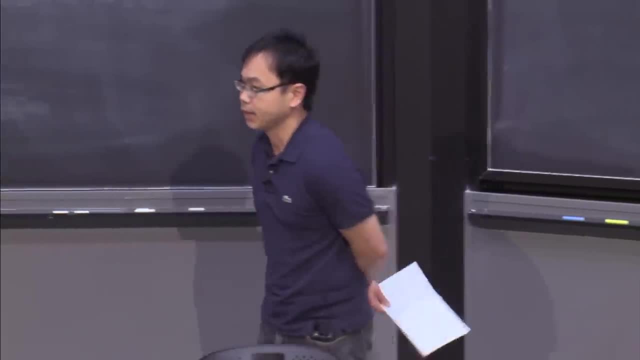 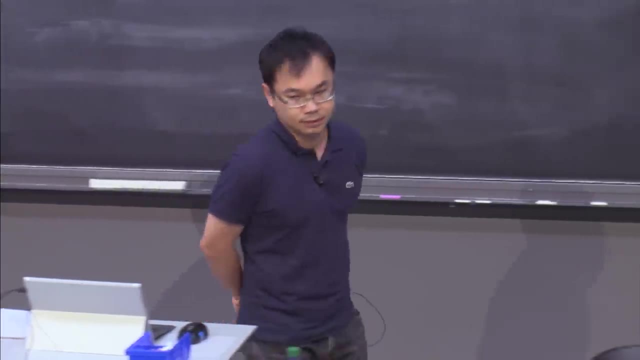 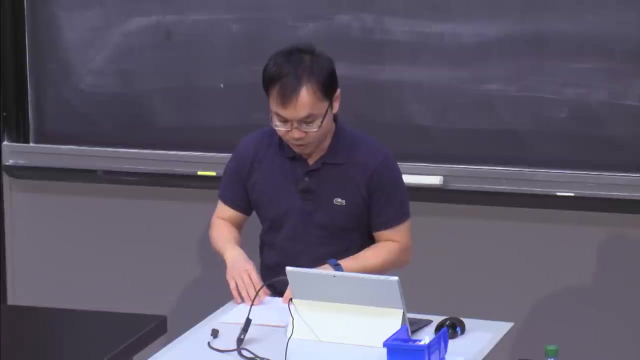 Finally, last time we actually discussed sound waves, We have open pipe and we can have air inside the pipe, And the behavior of the air or the molecules inside the organ pipe can be described by wave equations. So what we are going to do today is: 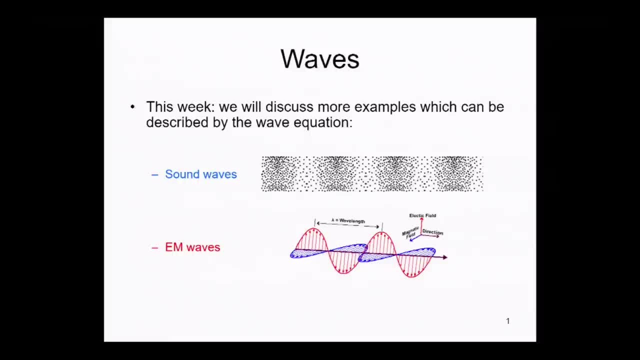 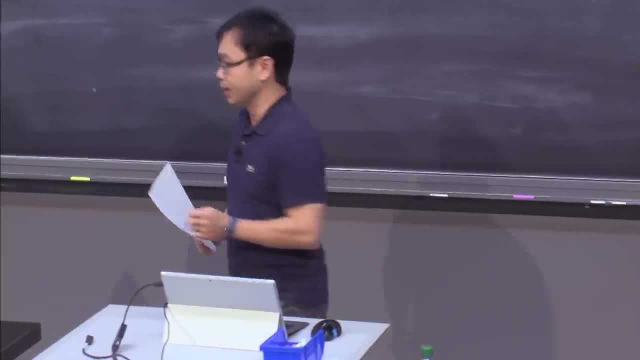 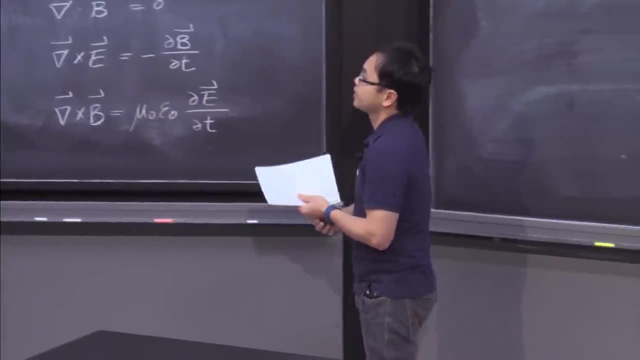 to discuss with you a special kind of wave, which is electromagnetic waves, And that's actually slightly different from what we have learned in the last few lectures, And we will see what is the difference today in the lecture. All right, so this is a reminder of Maxwell's equations. 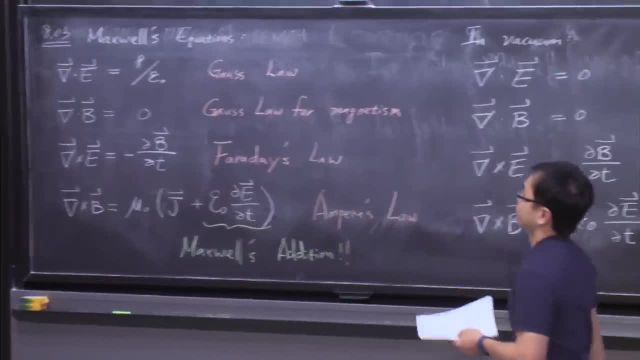 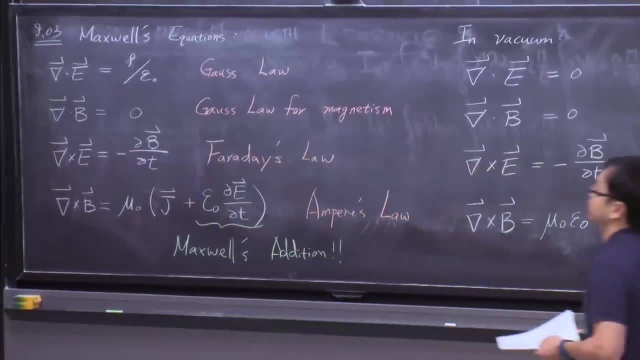 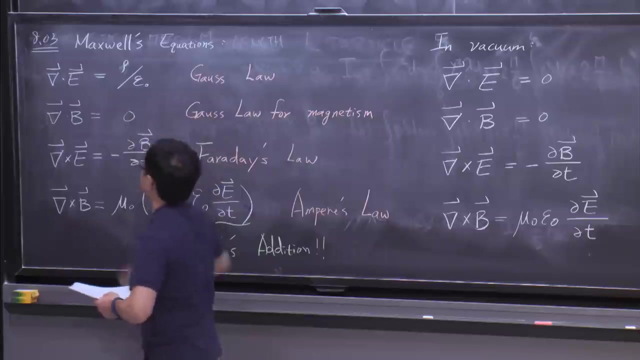 So basically, what is written here are the differential form of Maxwell's equations. OK, so the first law is Gauss' law. It says: should the divergence of E, the electric field is equal to rho, which is the charge density. 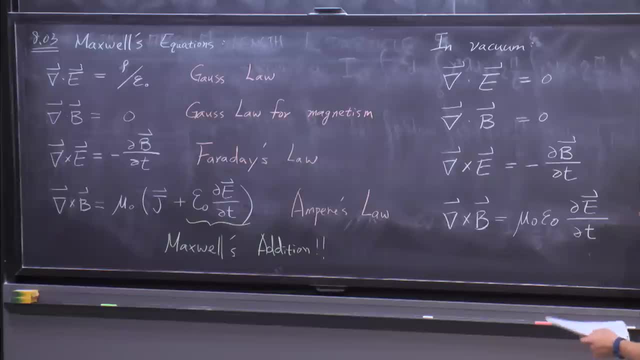 as a specific point, divided by epsilon 0, which is essentially a constant. We'll call it permittivity, this constant which actually relates the divergence of E And then the density wave and the density of the charge at the specific point. 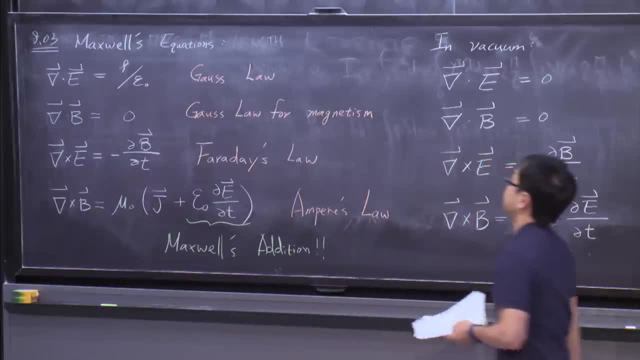 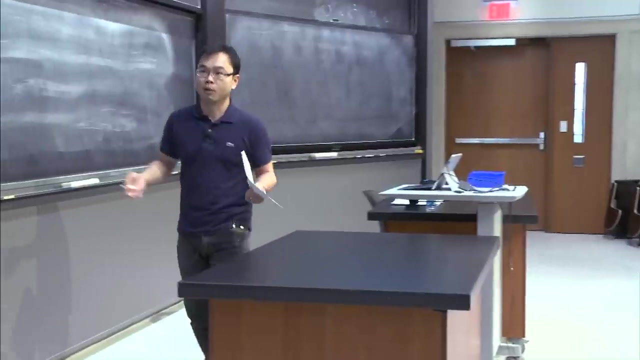 And the second law is actually Gauss' law. for magnetism, This is actually divergence of B equal to 0. So divergence of B is always equal to 0, because we don't have yet discovered the magnetic monopole yet, right? 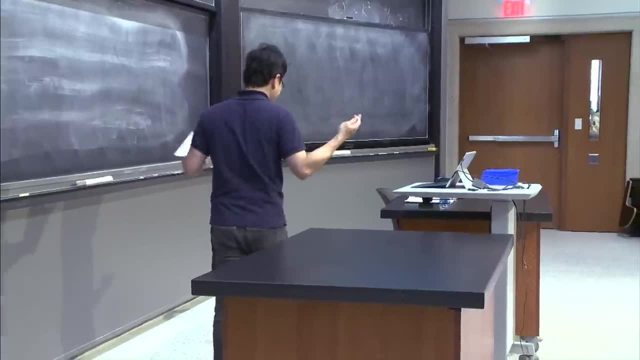 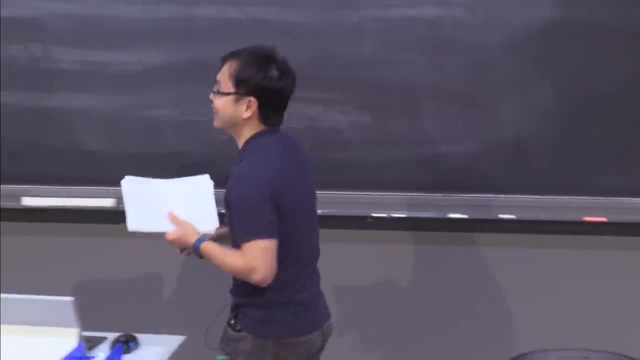 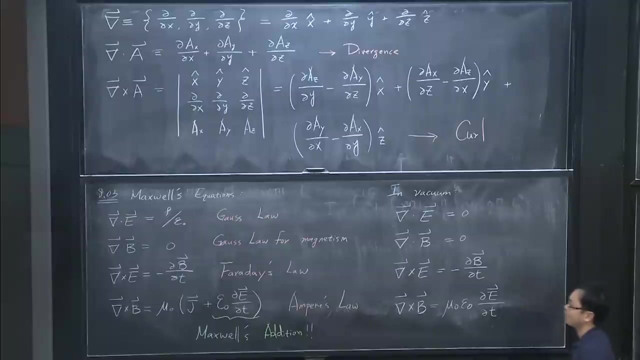 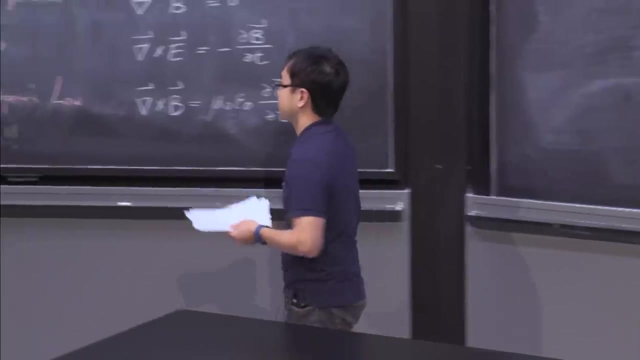 So maybe you have discovered it one time, at some time in your experiment, And please let me know. I want to be the first who knows the result. All right, so promise me. The third one is Faraday's law. It's a curl of E equal to minus partial B, partial t. 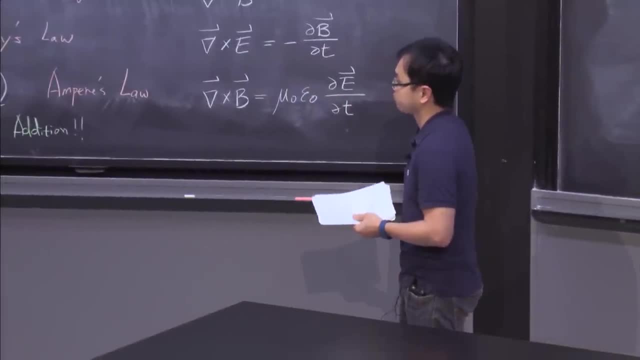 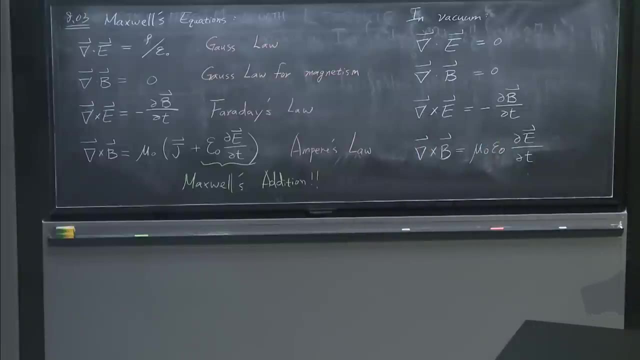 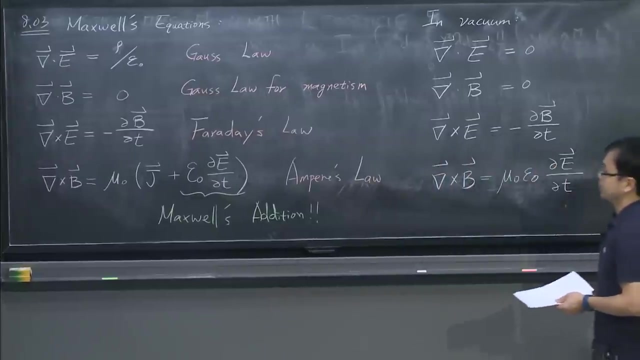 And the B, as a reminder, is a magnetic field vector And the last law is actually Ampere's law. It's actually a curl of B equal to mu 0.. Mu 0 is actually a constant permittivity and which relates the current and displacement current. 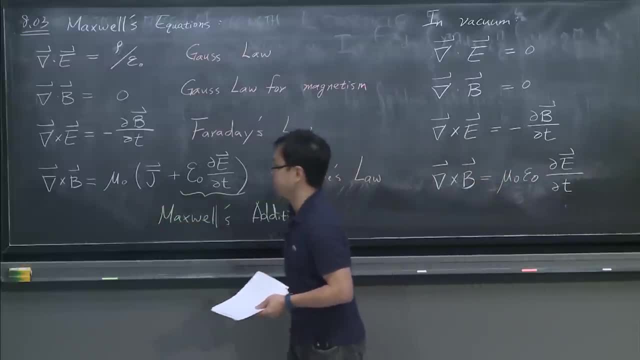 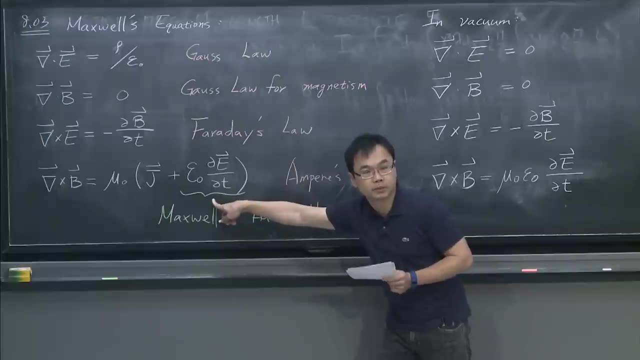 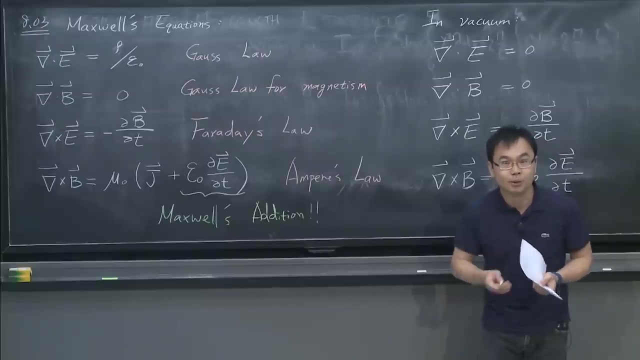 epsilon 0, partial E, partial t to the curl of B, And I would like to draw your attention that this term, this very important term, is actually Maxwell's addition. OK, So if I have a collision, there will be no electromagnetic wave. 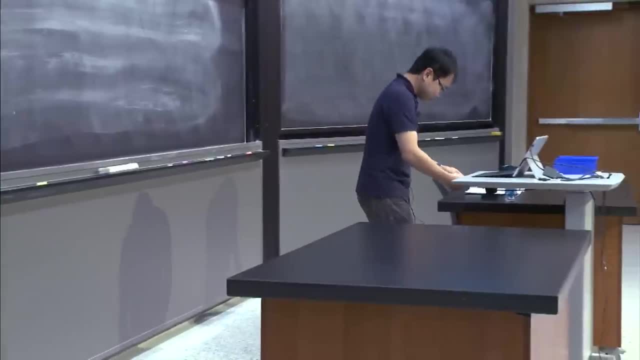 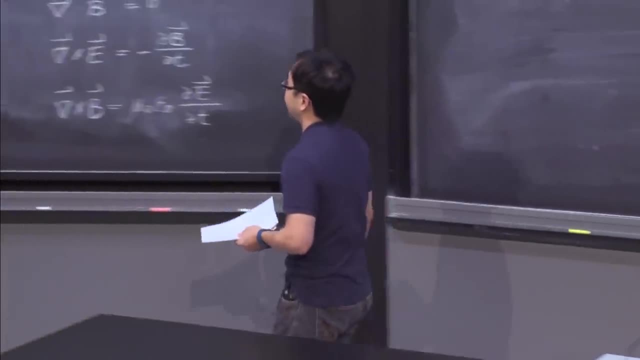 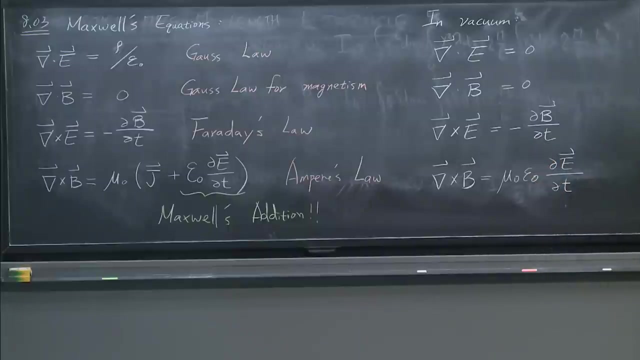 Then you cannot see me, OK, All right. So what we are going to discuss today is a simpler case at the beginning. So what will happen if we go to vacuum? OK, Go to vacuum means there will be no material charges floating around. 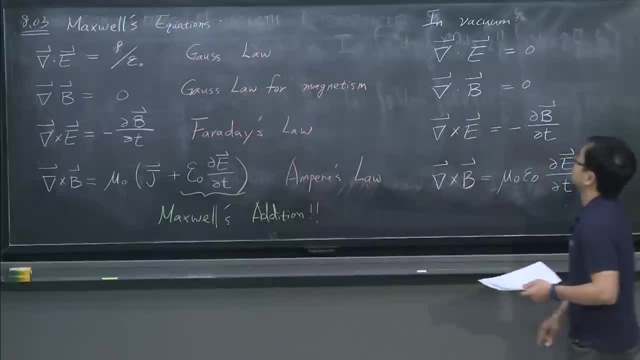 OK, So that means rho will be equal to 0.. Therefore, the divergence of E will be equal to 0.. And also, in the last equation, Ampere's law J, which is the current density, will be equal to 0. 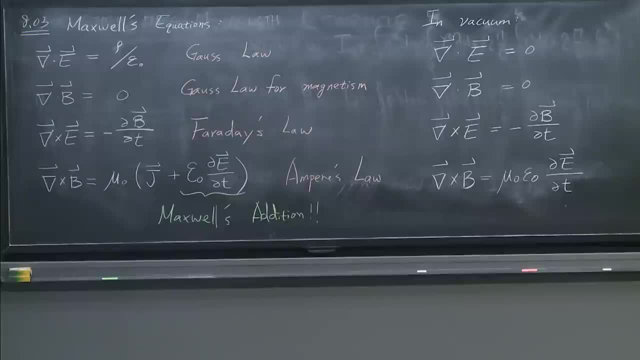 Therefore, the function of form becomes a curl of B equal to mu 0, epsilon 0, partial E, partial t. OK, So Before, Before, Before we go into the discussion of Maxwell's equation and its implication, I would like to remind you about some mathematics which 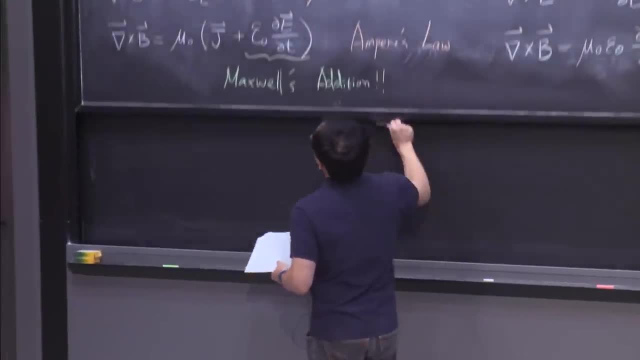 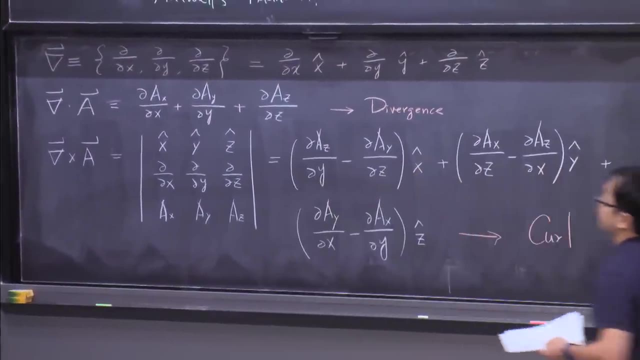 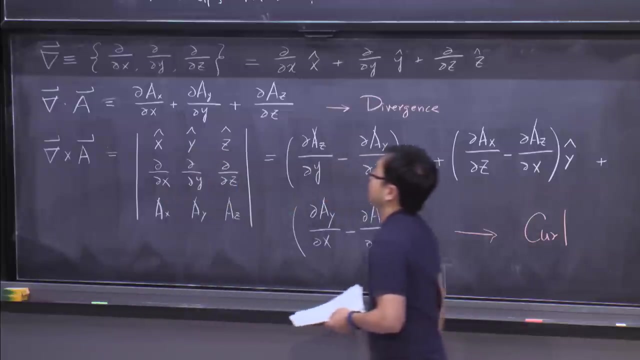 will be used, which will be used in this lecture- I hope you have seen this in other course- or AO2.. So, as you can see, we use del here, which is a vector, And this vector is defined as partial x, partial y. 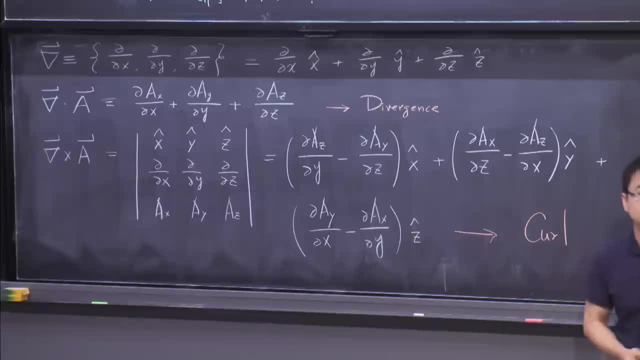 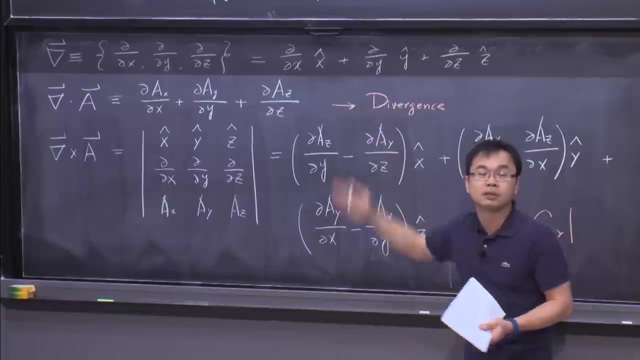 and partial z in the x, y and z direction. OK, So this is actually some kind of operator, operator which you will see that again, a lot more of operators in AO4.. And we make this definition because I'm lazy, right. 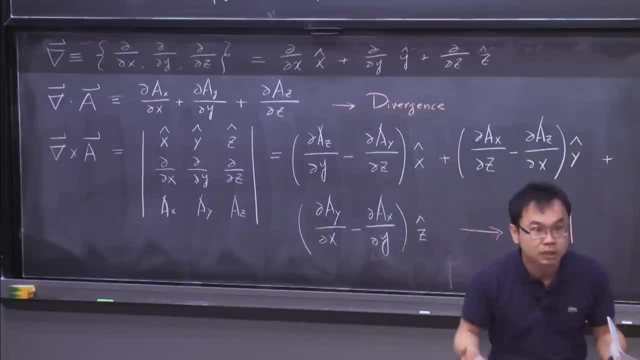 Because I don't want to write so many partial partial x, partial partial y, And I don't want to write so many partial x, partial z again and again. Right. Therefore, we define del, which is like this: It looks really crazy, but it really. 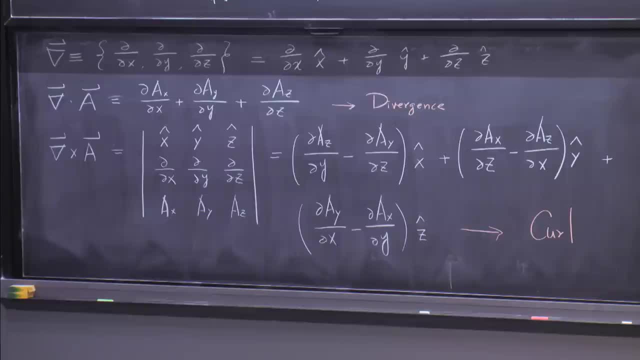 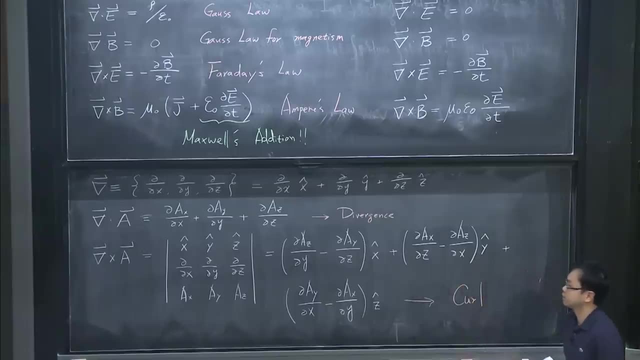 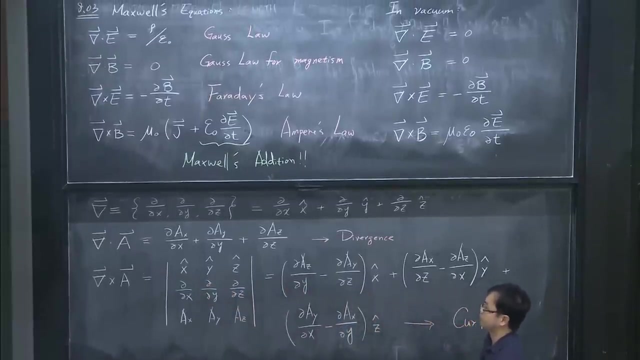 makes our life much easier. OK, So that's the whole reason. OK, As a physicist, And as we discussed before, we have divergence, which is defined here: Del times A. both of them are vectors, One is operator vector. 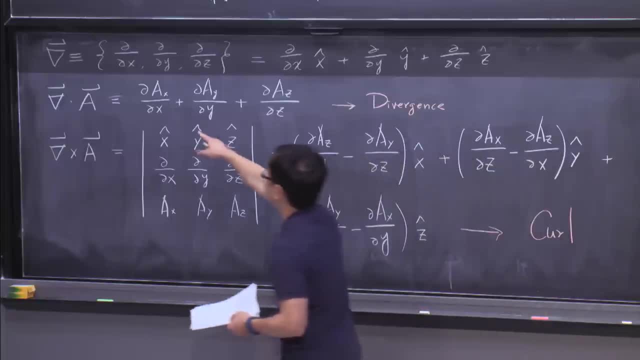 And the other is actually really a vector. You basically get partial A x, partial x plus partial A y, partial y plus partial A z, partial z. So basically you just multiply them like normal operation And you can actually get this equation. 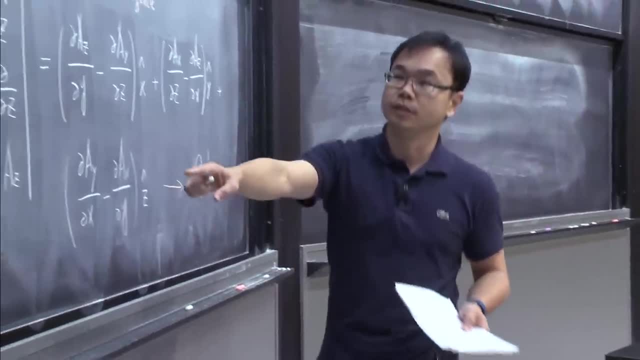 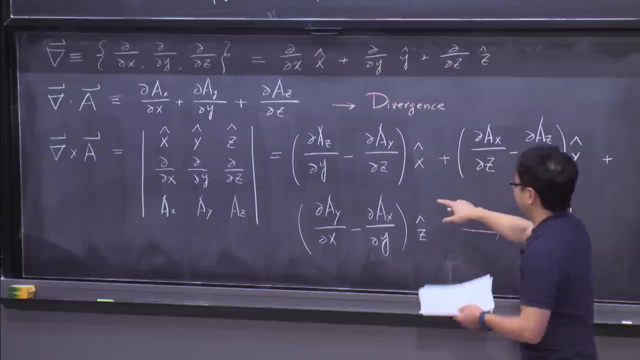 OK. Then finally there's curl. Curl is actually like this: It's actually del cross A. OK. So basically, maybe in the past you see this complicated formula. You have, maybe no meaning to you, And one easy way to remember this curl. 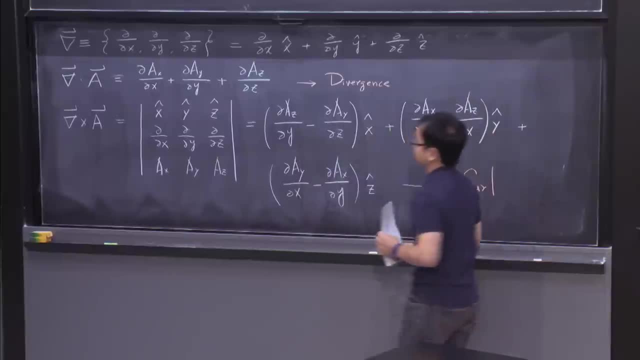 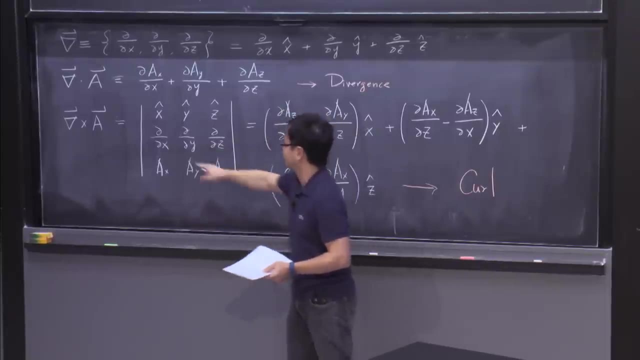 is to not care about this. Don't look at the right-hand side part, But just remember that you can actually construct this curl by a determinant of a matrix, The matrix. I can fill the first row by x, y and z. 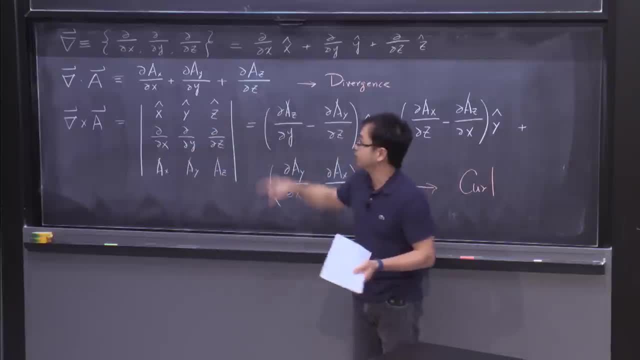 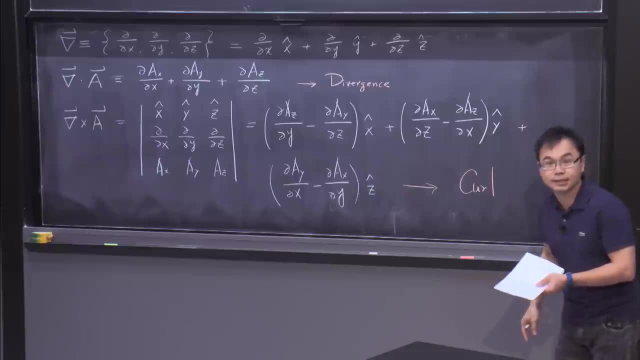 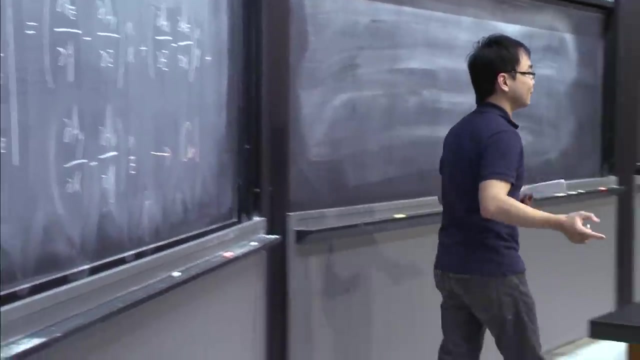 and the second row. I filled it with the content of del. Finally, I filled the content of the matrix with A vector. Then you will be able to calculate the determinant of this matrix. Then you naturally will get this very longish formula. 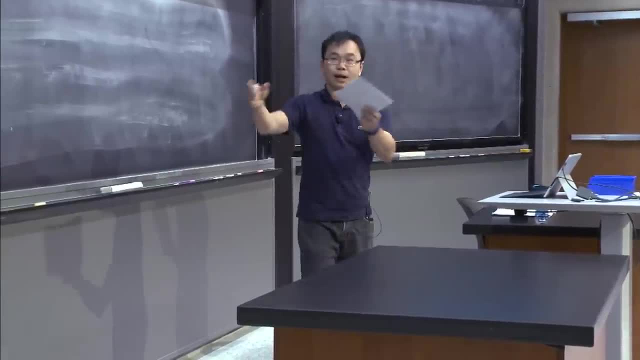 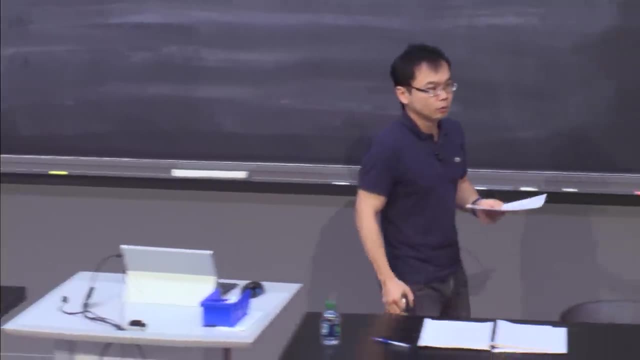 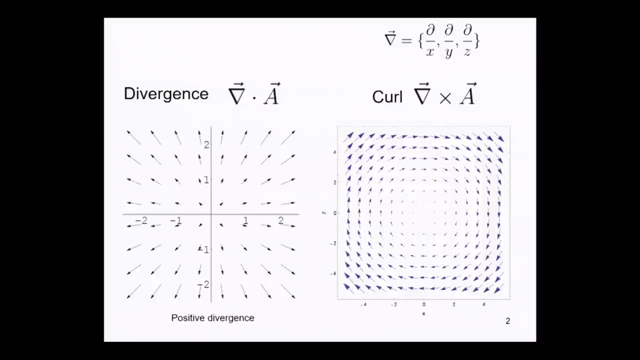 So you don't really need to remember the formula, But you will be able to know how to calculate that really easily, OK, OK, So we talk about divergence, We talk about curl. We have. what does that mean? Right, Divergence, curl, what does that mean? 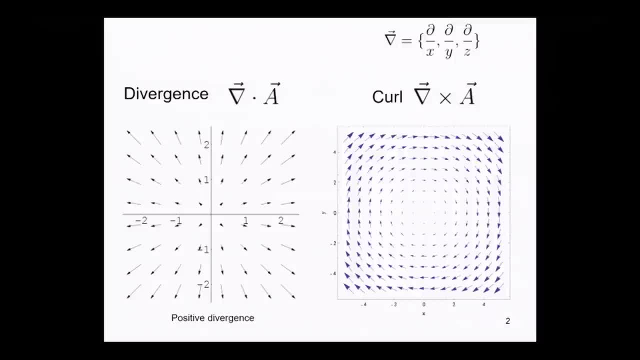 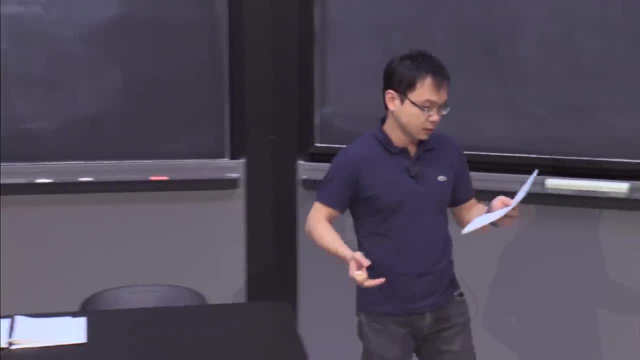 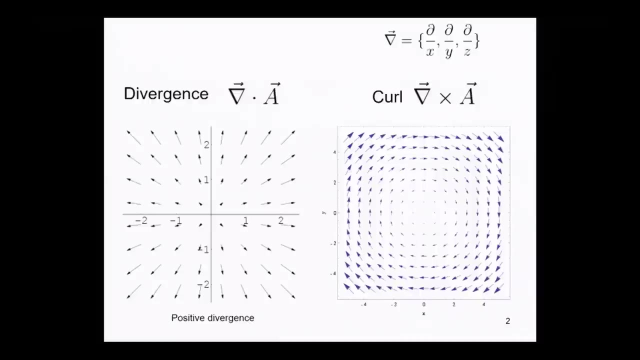 OK. So divergence is actually some kind of measure which measure how much the vector v OK spreads out or diverges from a point of interest, Right? So in this example there is a vector fill. Vector fill means at any point in the space. 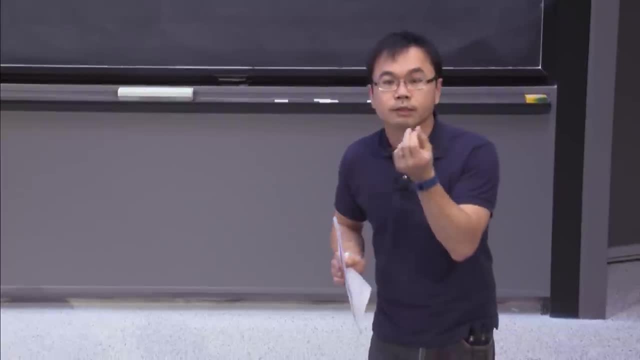 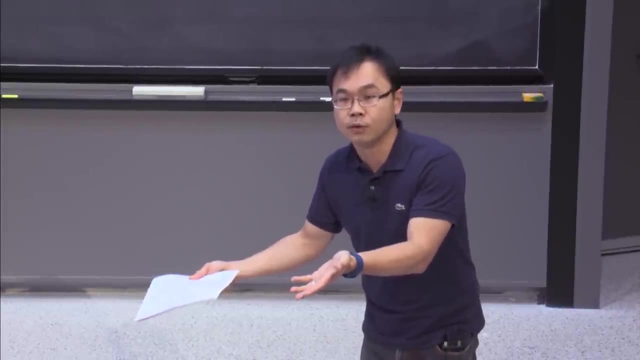 in any point in the space OK which I am discussing, there is a vector associated with that And I call it vector fill. We know scalar fill very much right. For example, the temperature as a function of position is a scalar fill right. 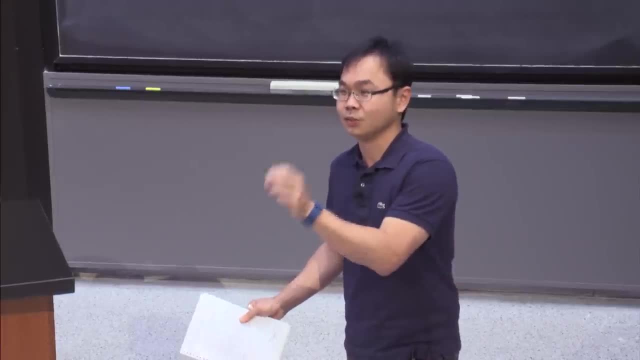 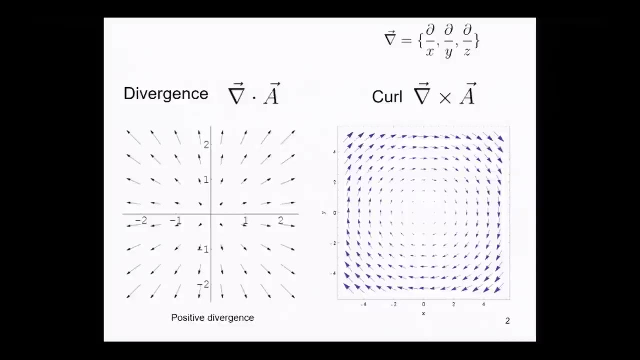 So every point You have a scalar corresponding to that point And in the case of vector fill, every point you have a vector connected to that point. OK, And if I arrange the vector fill like that, each arrow is actually a three-dimensional vector. 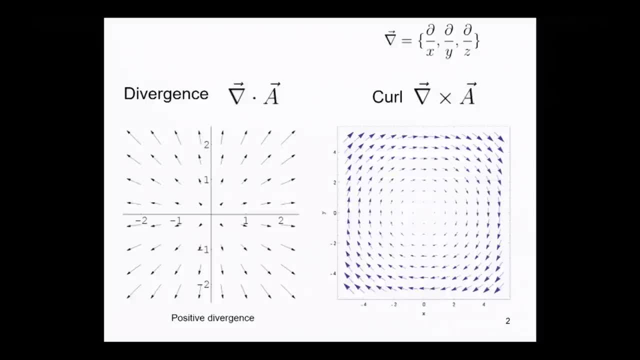 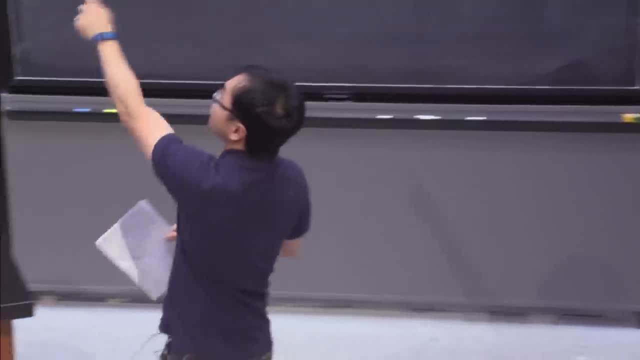 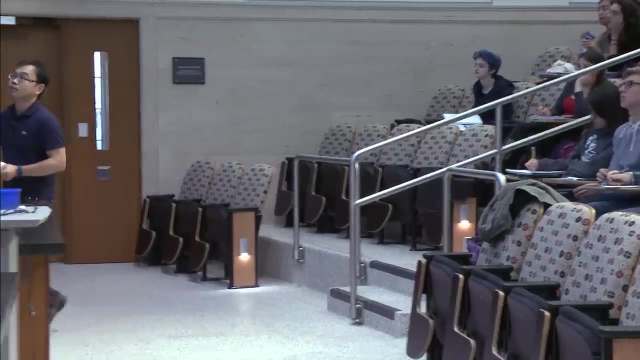 OK, Then if I evaluate the divergence and you see the heart, it looks like something is really spreading out from the center to the right And that will give you positive divergence. OK, So that's the physical meaning of this formula. And second formula which we discussed is the curl. 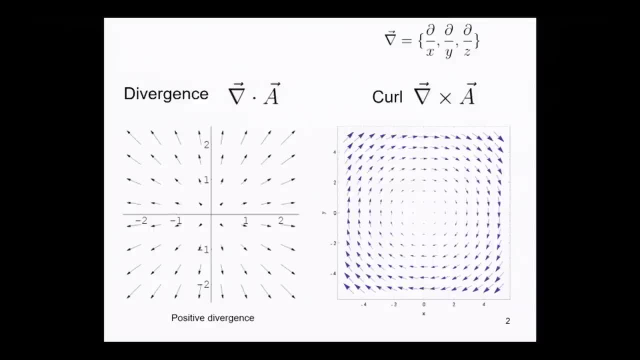 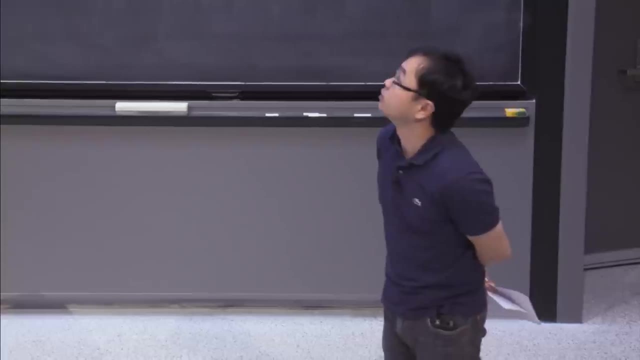 Right, So curl is actually the del cross A It's a measurement of how things are curling around, a point of interest. OK, So you can see that if I arrange my vectors in a space like that, then you will see that really. 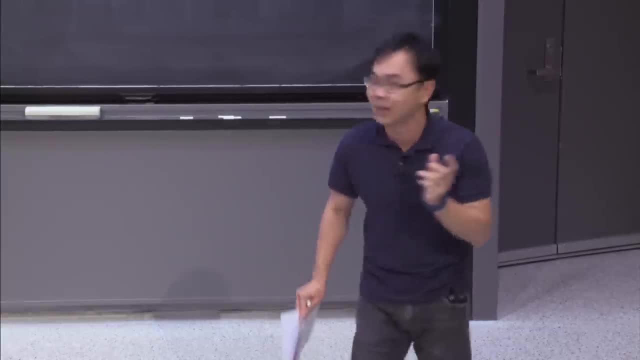 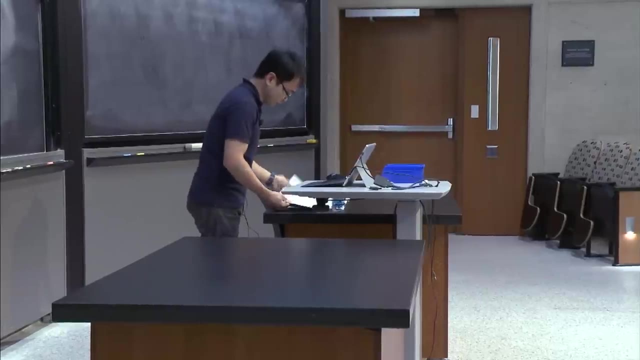 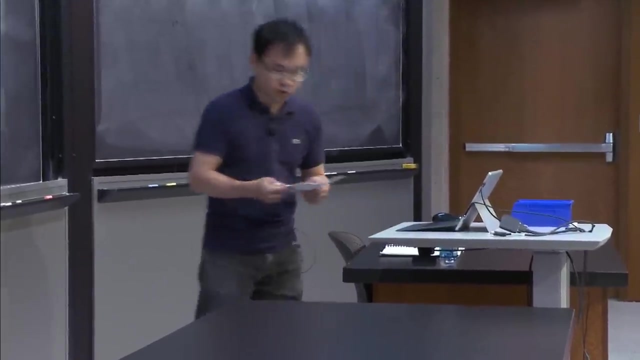 it's like something is really rotating around that specific point. Therefore, if we evaluate the curl, you will get the non-zero value. OK, So that's actually the physics intuition which we can, or say the mathematics intuition which we can actually get when we discuss. 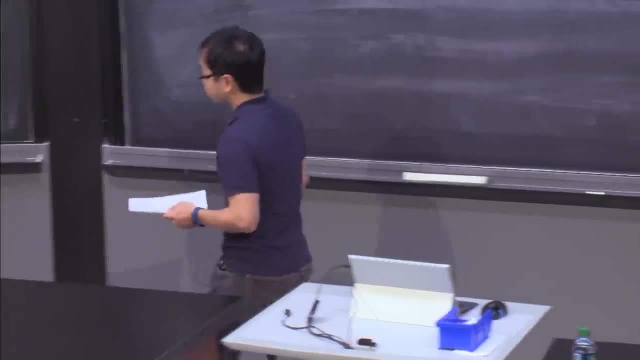 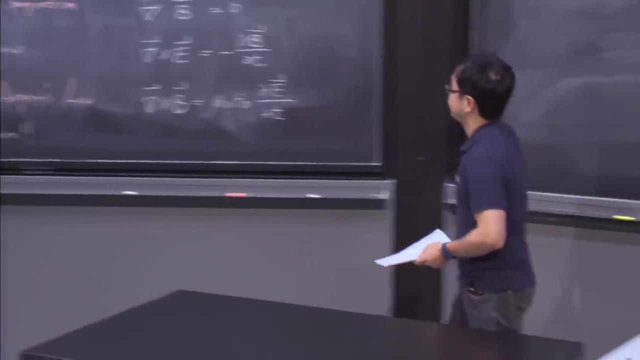 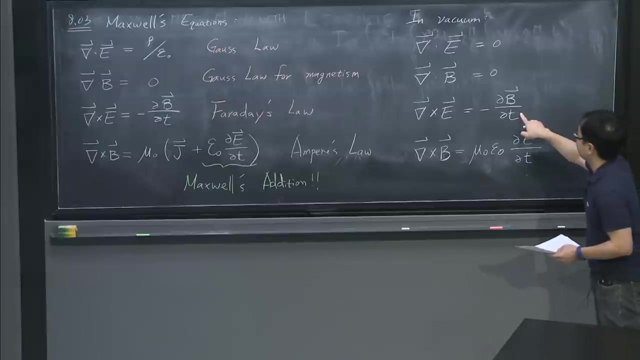 before the discussion of the Maxwell's equation: OK, So if you accept those ideas and let's take a look at what we have here, especially in the vacuum case, OK, So in the vacuum case you have a curl of E equal to minus, partial B, partial T. 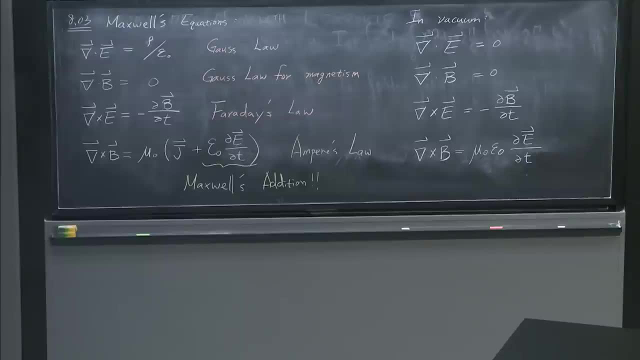 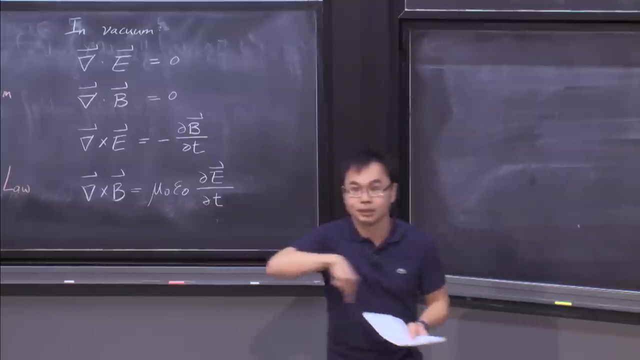 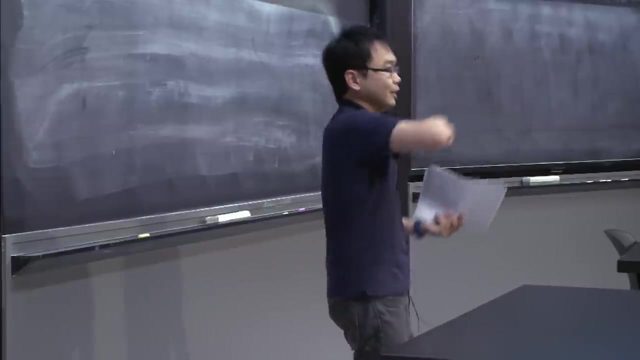 OK, What does that mean? That means if you change the magnitude of the vector field, magnetic field. if you change the magnitude of the magnetic field, OK, that will introduce a curling around thing in the E field. OK, So if you change the size of the B field? 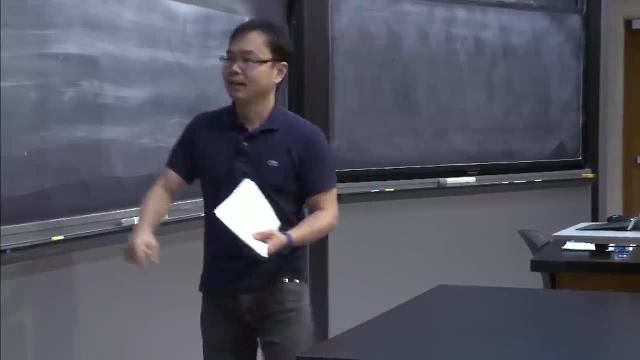 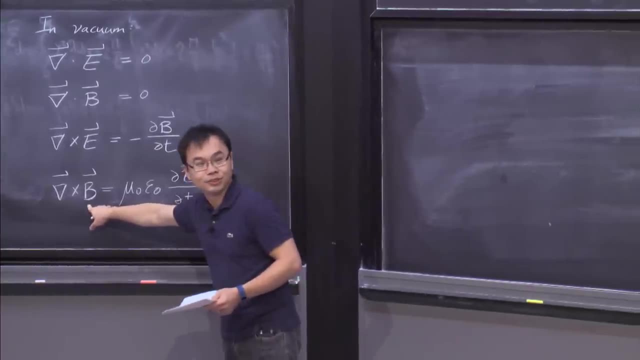 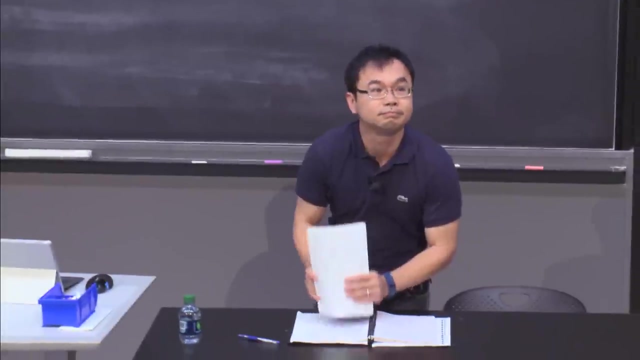 then the E field will start to curl around, doing this. OK, And on the other hand, if you change the electric field, that will produce something which is curling around in the B field. OK, All right. So do you have any questions? 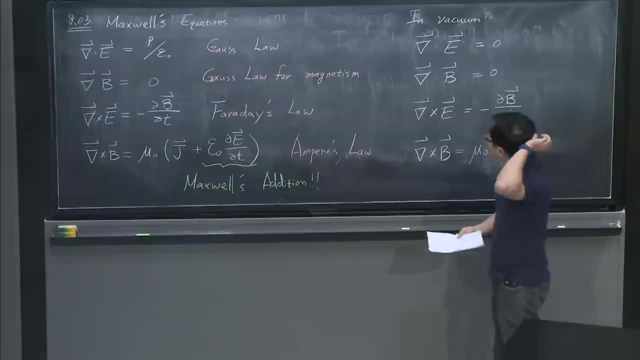 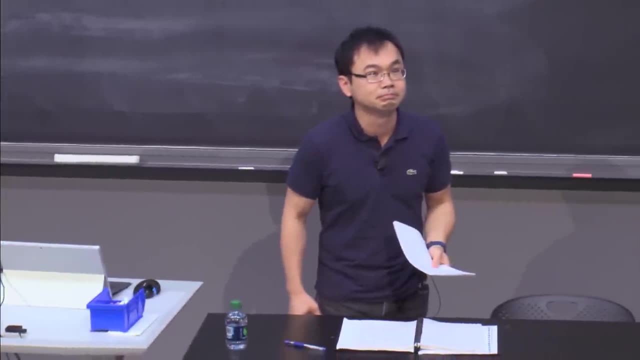 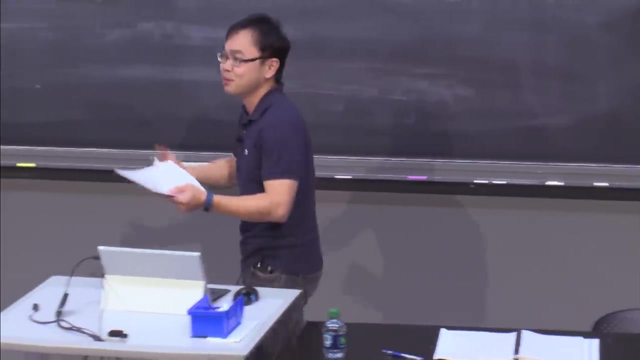 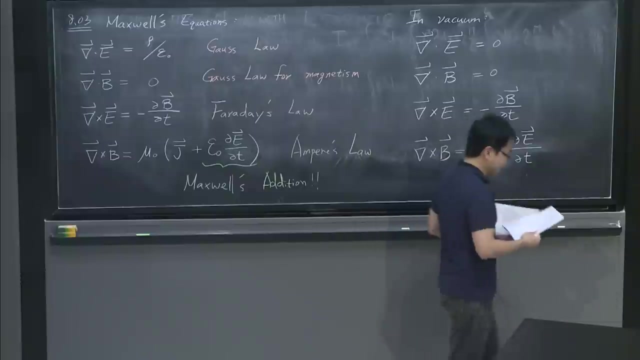 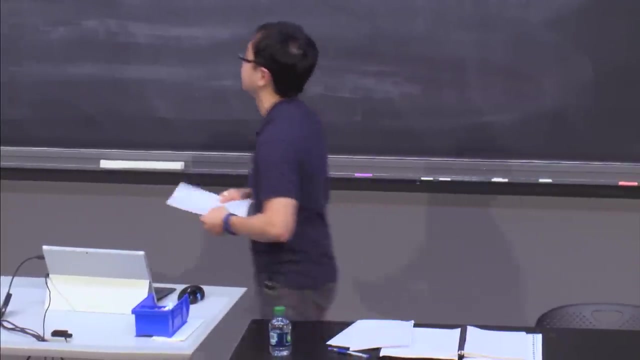 I hope everybody is familiar with this notation. So from here, actually, Maxwell, see the light. Can you see it? Maybe not yet. Maybe we are slightly slower than Maxwell, But we will see that together in this lecture. OK, For that I will need, as usual, the help. 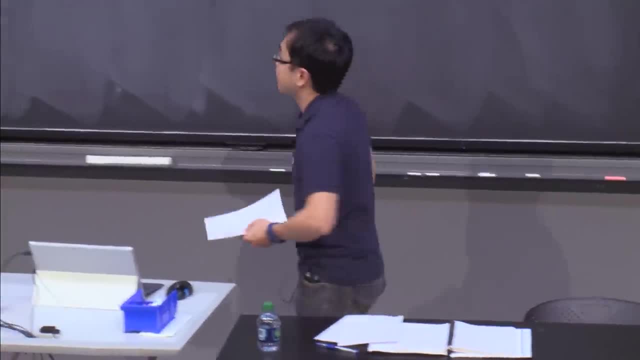 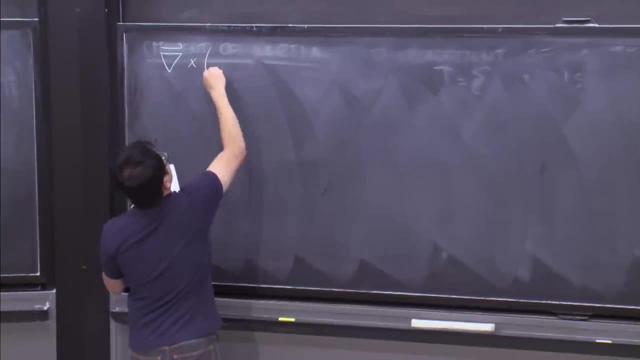 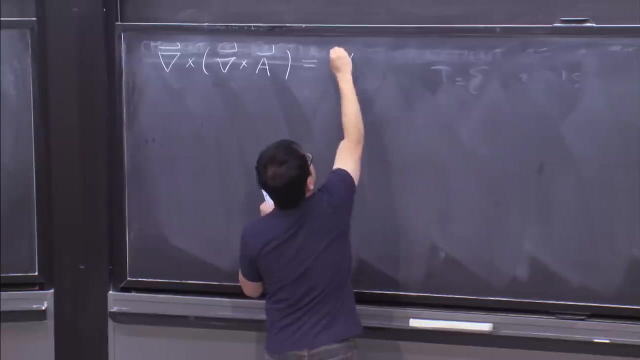 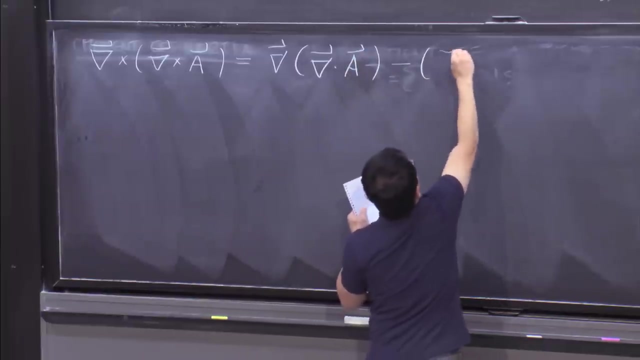 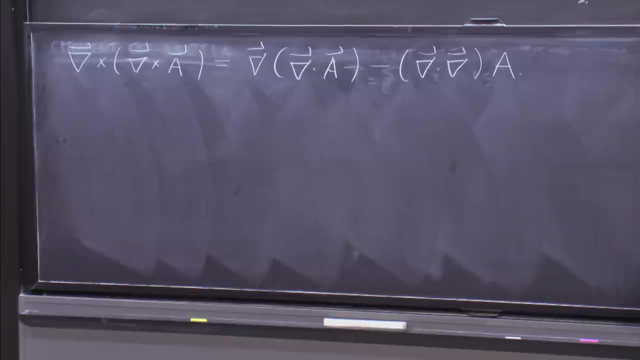 from the math department. Right, So we are going to use this identity. This identity is curl of A, And curl of A will be equal to del divergence of A minus del dot del A. OK, So this is an identity which we learned. 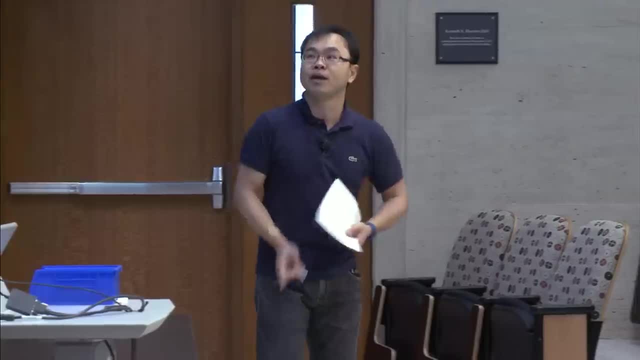 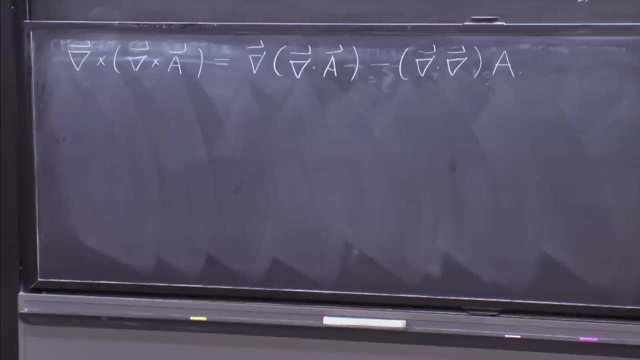 from the math department And, of course, if you are patient enough, you can actually expand all those terms and you will see the left-hand side of the formula and right-hand side of the formula And you will see that really, this works. 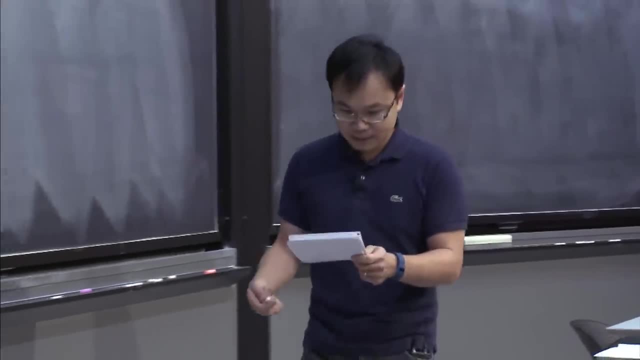 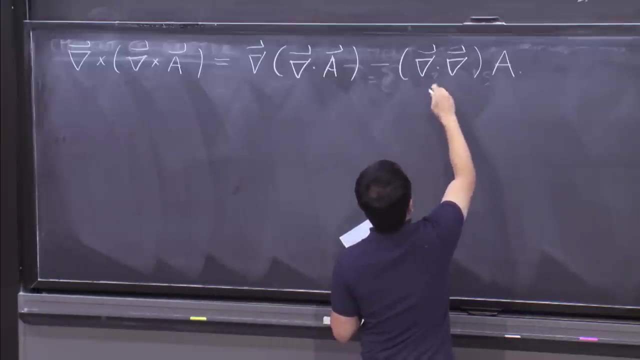 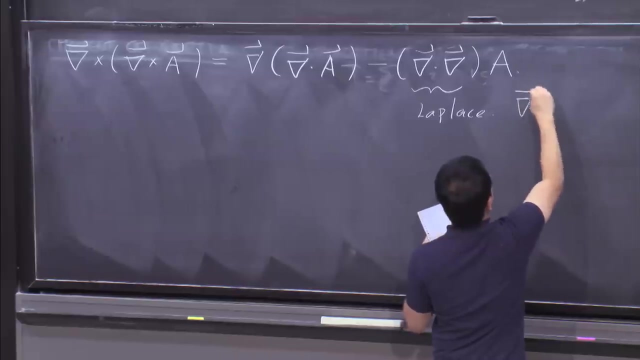 OK, So I'm not going to do that here in front of you. So, if you accept, this is an identity And usually when we have del times del, we call it Laplace And usually we write it as del squared. 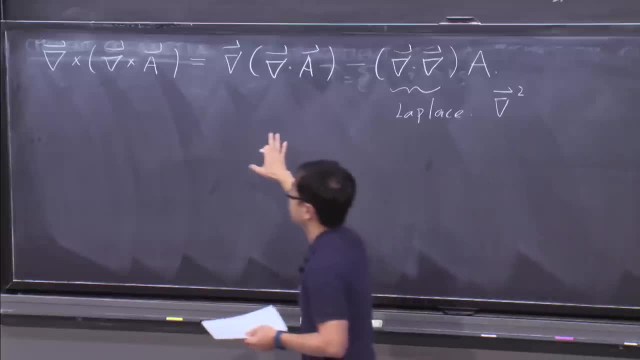 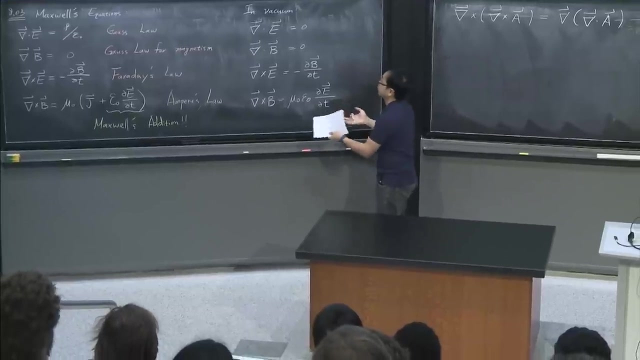 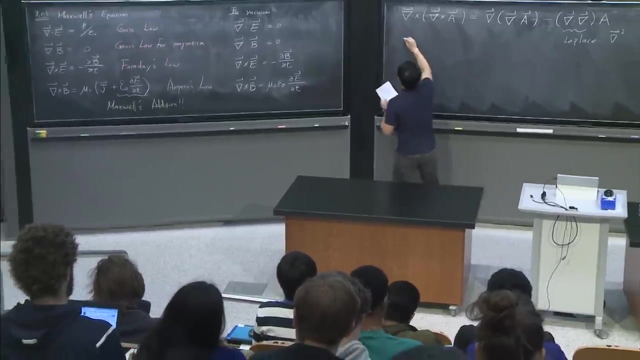 OK. So with this formula I can now put in my electric field into this formula, Right? So if I put in the OK, assuming that I am working in a situation of vacuum, OK, and I plug in my electric field into that formula. 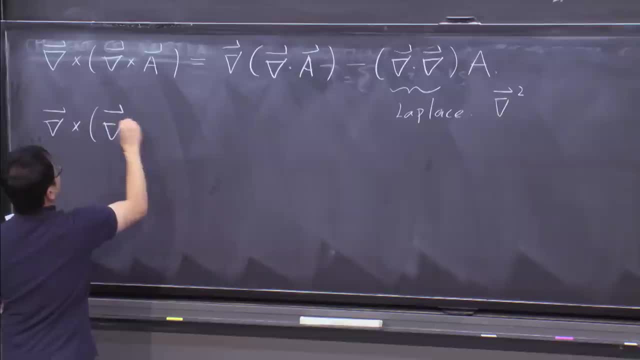 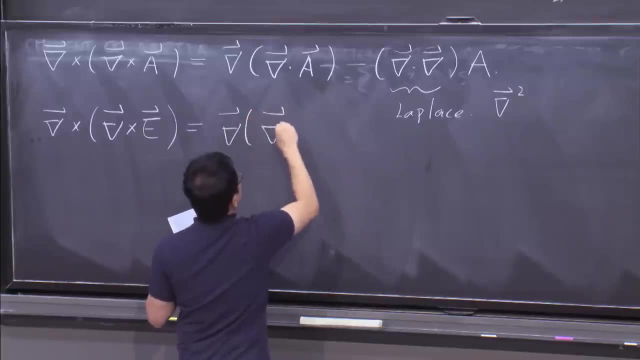 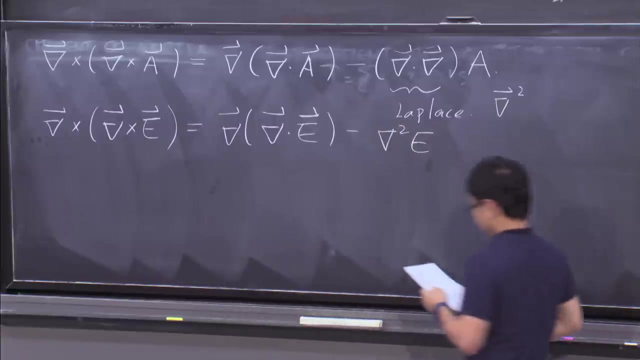 then this is actually what I'm going to get- Curl of E, And this will be equal to del divergence of E minus del squared E. OK, And based on the four Maxwell's equations, we can immediately recognize that divergence of E is equal to 0, right. 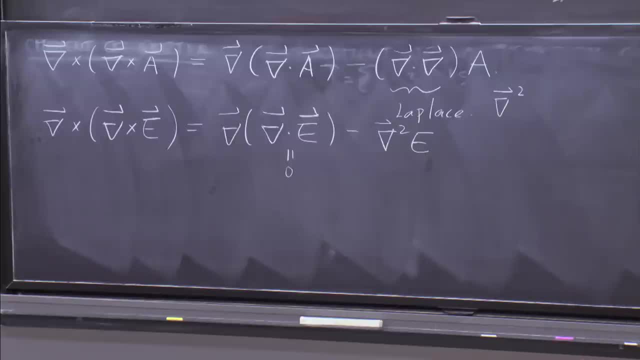 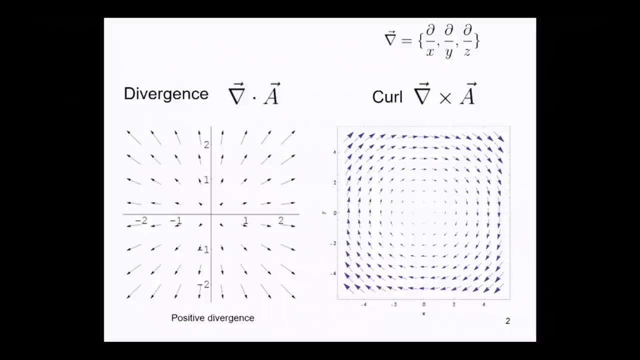 Because I don't have charges around. Therefore, you cannot introduce a gradient or a divergent. OK, You cannot introduce positive divergence in the electric field. Therefore, when you evaluate the divergence of the electric field, that is equal to 0.. 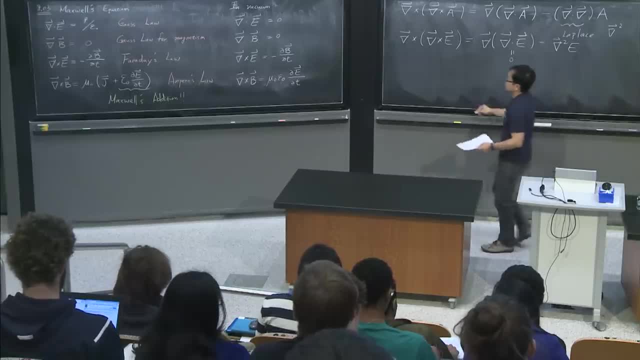 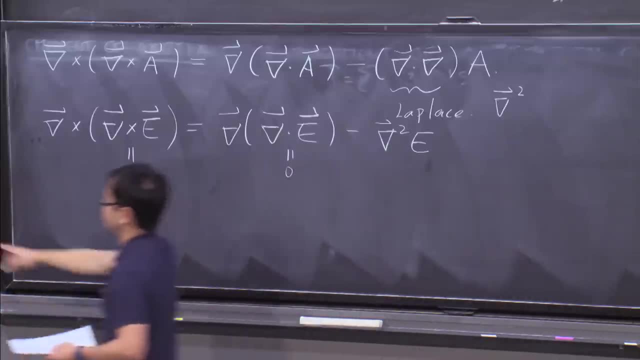 OK, According to that formula, the Gauss law, And you can also take a look at here- So we have curl of E according to this formula. OK, Basically you can actually conclude that this will be equal to partial B minus partial B. 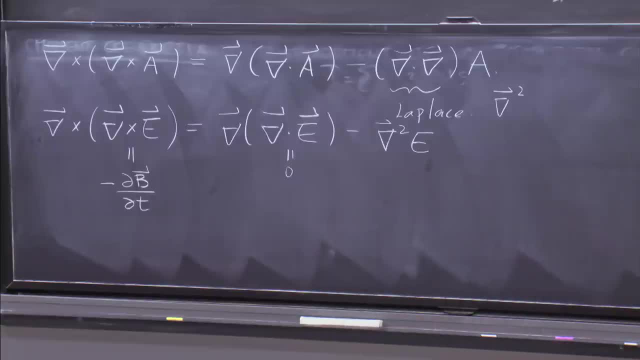 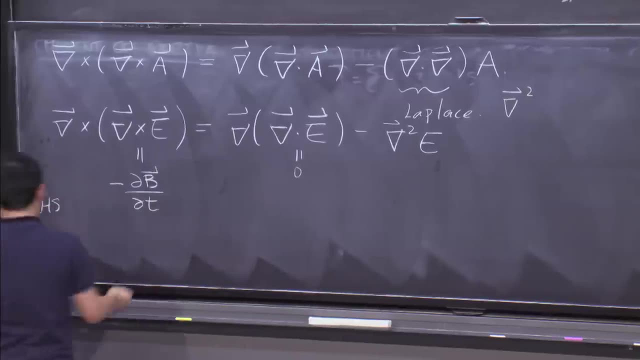 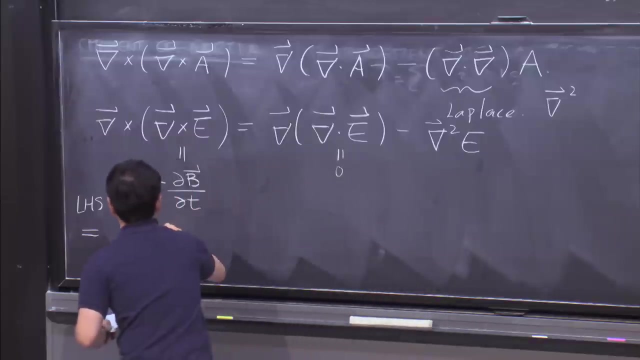 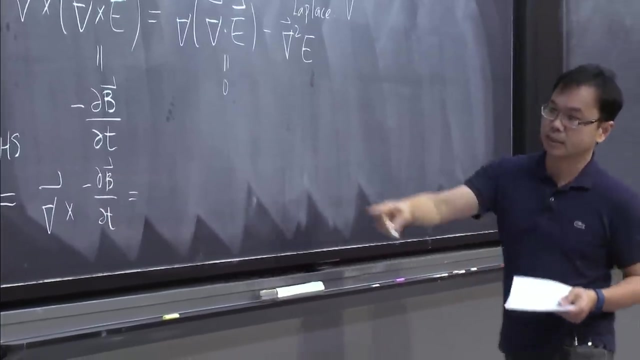 partial t according to Faraday's law. OK, So if I look at the left-hand side, OK, that will be equal to a curl of E And this will be a curl of minus partial B, partial t, And this will be equal to, basically I: 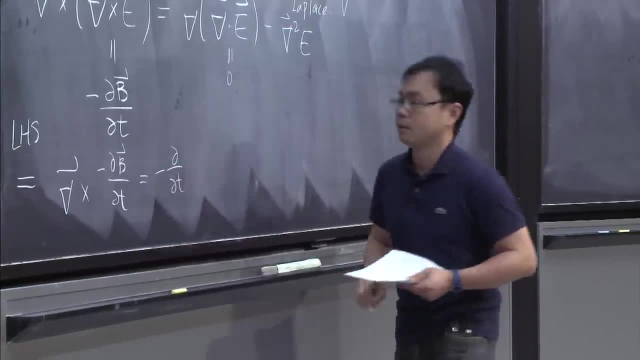 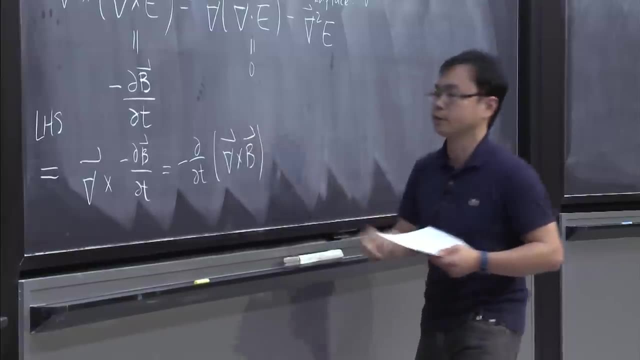 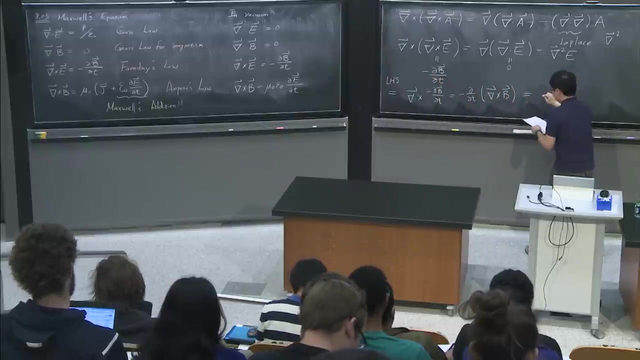 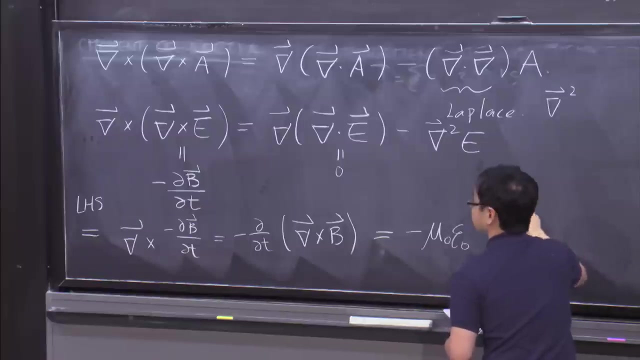 can take the minus sign out and take the partial partial t out And basically you have curl of B right And according to Ampere's law this is equal to minus mu, 0, epsilon 0. partial square E, partial t. OK, 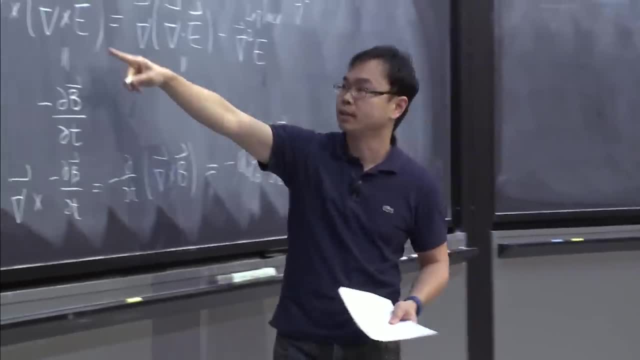 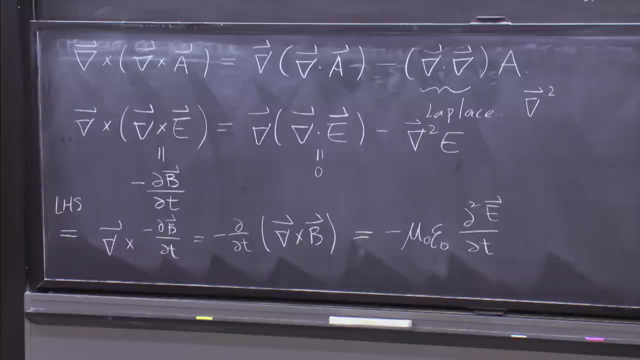 Everybody is following Right. So basically what I have been doing is copy the left-hand side and make use of the Ampere's law And basically you get minus mu, 0, epsilon 0, partial square, E, partial t squared. OK, 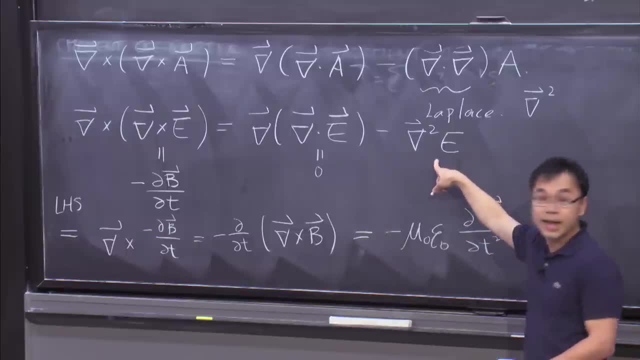 And this thing: the left-hand side is equal to the right-hand side. right, OK, The right-hand side. what is left? This is equal to 0.. So this is gone, And what is actually the remaining part is actually minus. 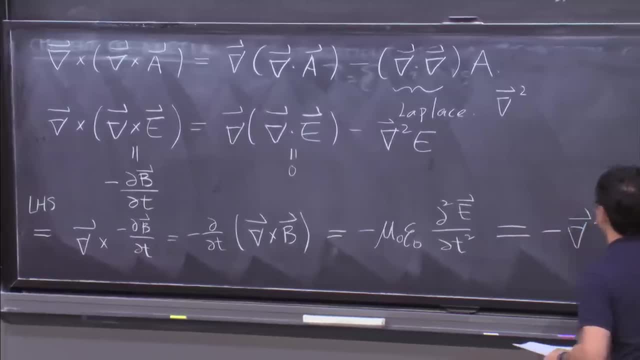 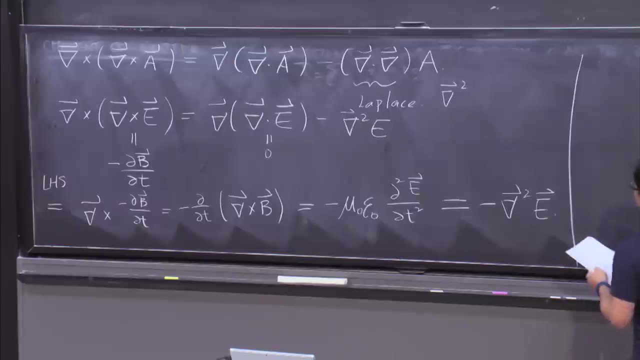 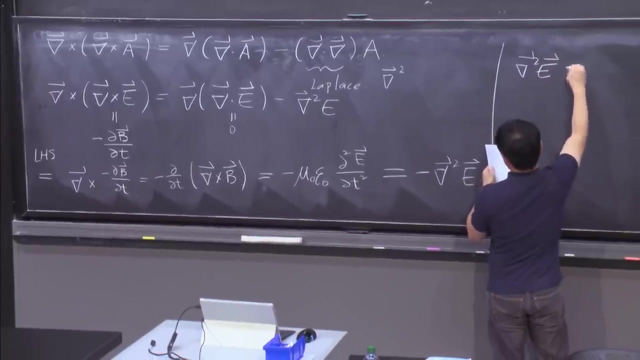 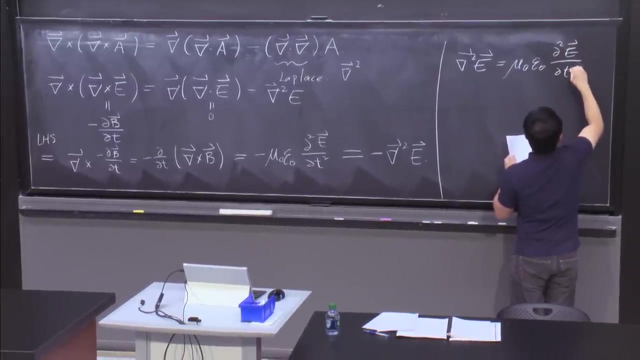 This is equal to minus del squared E. I can actually cancel the minus sign And then basically, what I am going to get is del squared E, And this will be equal to mu 0. epsilon 0. partial squared E. partial t squared. 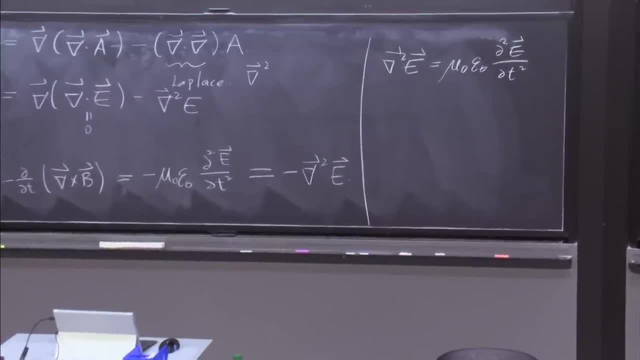 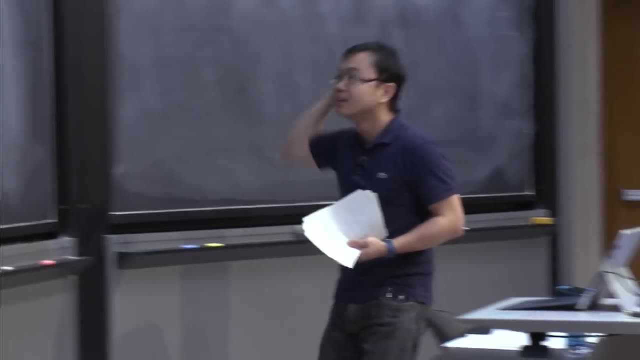 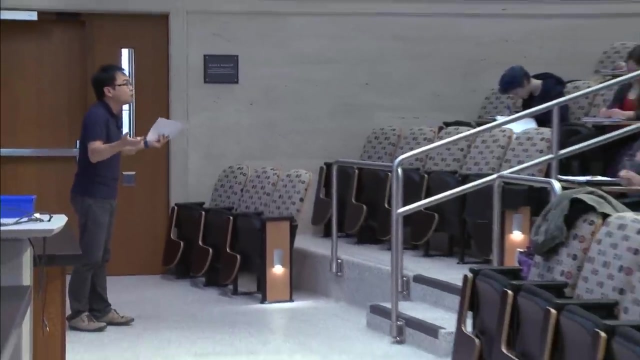 OK, Wow, this is what This looks like. what Wave equation again? Oh my god. But there's some difference, right? This is different from what we see before. right Before, the wave equation is only having partial square. 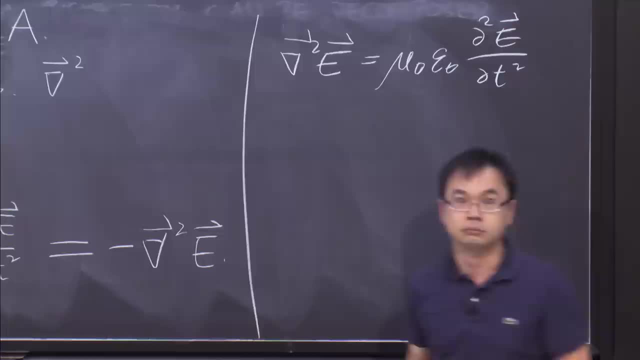 partial x squared. This time you have this del squared, Very strange, right. So what is this? Del squared is actually partial square, partial x squared plus partial square, partial y squared plus partial square, partial z squared. So this is an operator which you have three components. 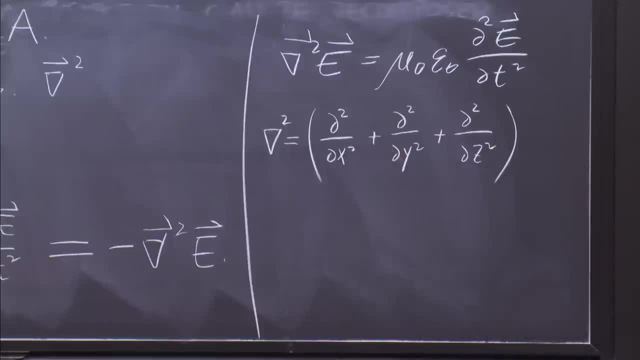 And, basically, if you do this calculation, you are going to have how many turns? How many turns will you have? If you do this del squared E, how many turns will you have? You will have how many? Anybody here help me? 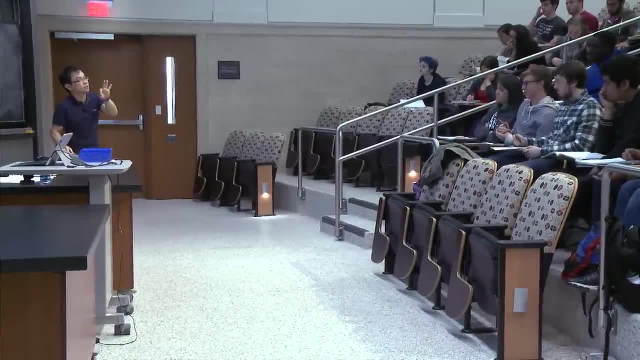 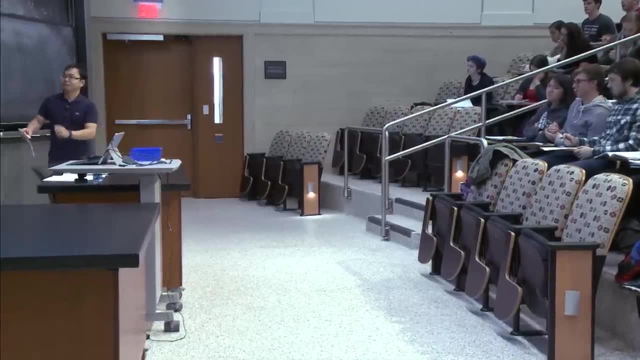 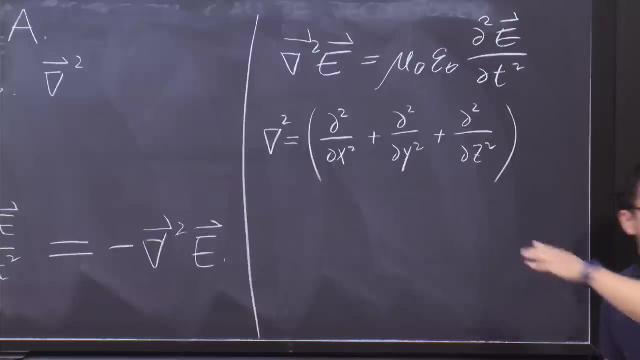 Three turns, Yeah, But you have three turns in x direction. You have three turns in y direction. You have three turns in z direction. Therefore, how many turns? You have nine turns. right, Because each operator is acting on the vector. 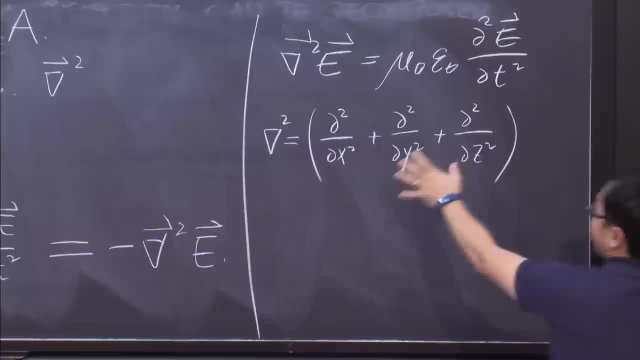 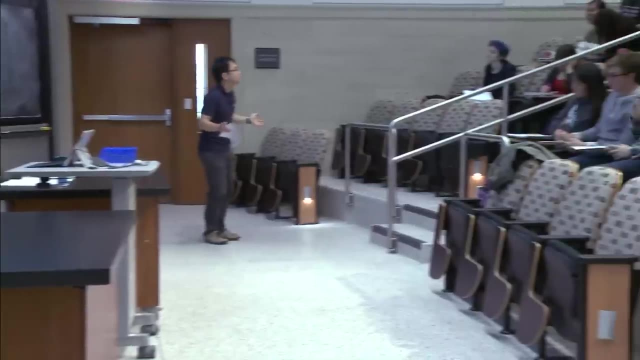 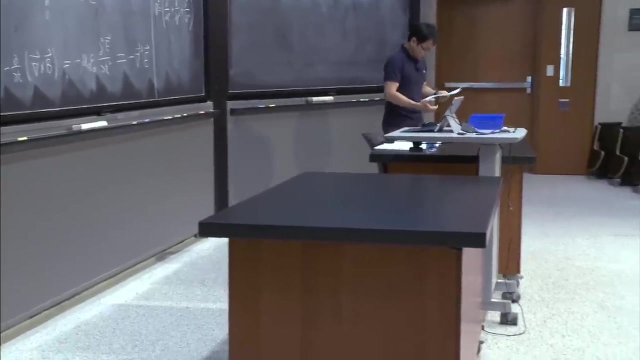 So very important, because this is a common mistake, right? So you have nine turns And it looks really like a wave equation. It tastes like equation, It looks like equation, It feels like equation, that wave equation, But it's actually a wave equation, right? 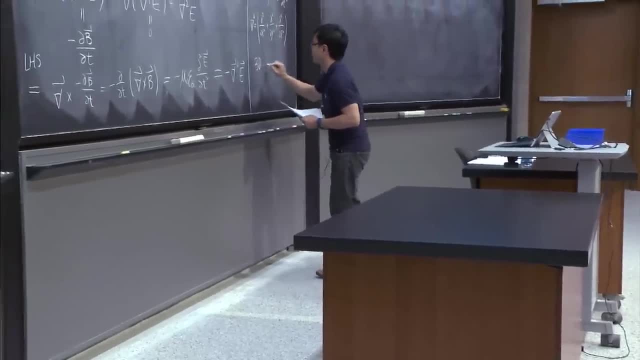 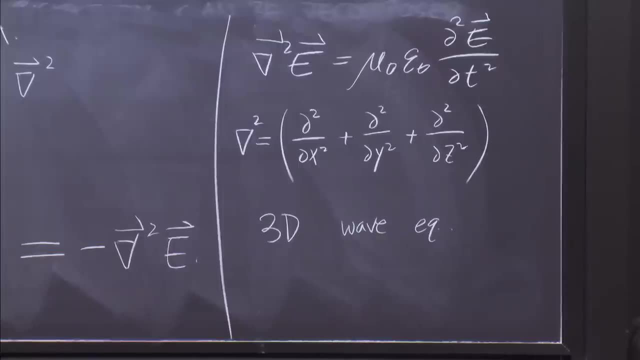 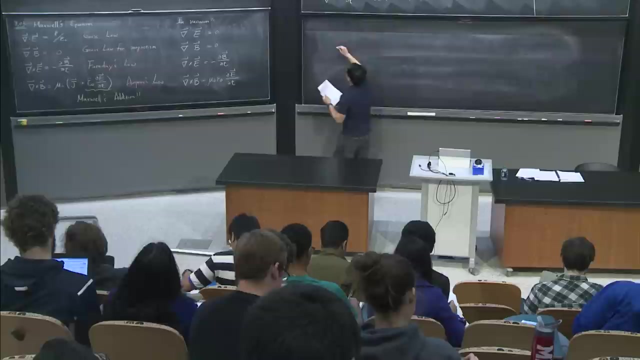 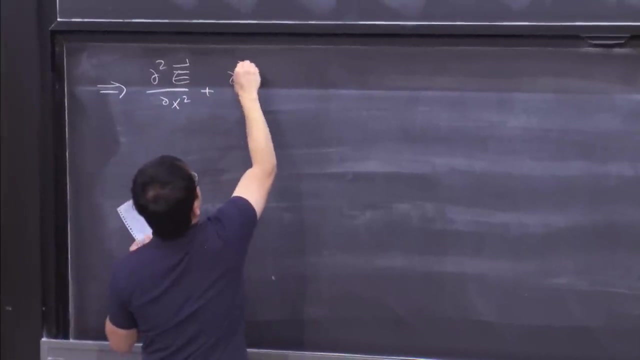 OK, So this is a three-dimensional wave equation. Ooh, very cool. So we are increasing the dimension, So I can write it down more explicitly. So, basically, what I'm getting is partial square E, partial x, squared, partial squared. 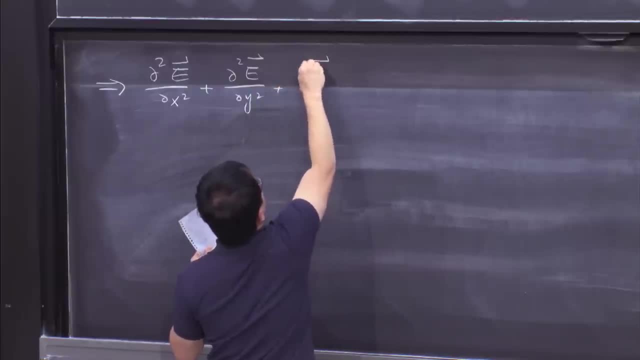 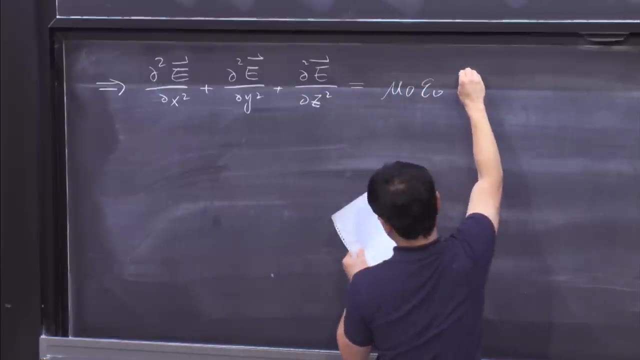 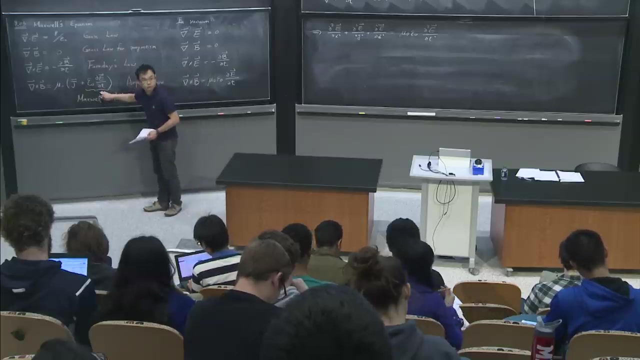 E partial y squared. partial square E partial z squared, And this is equal to mu 0, epsilon 0, partial square E partial t squared. OK, So Maxwell sees this when he actually adds this additional term here. OK, 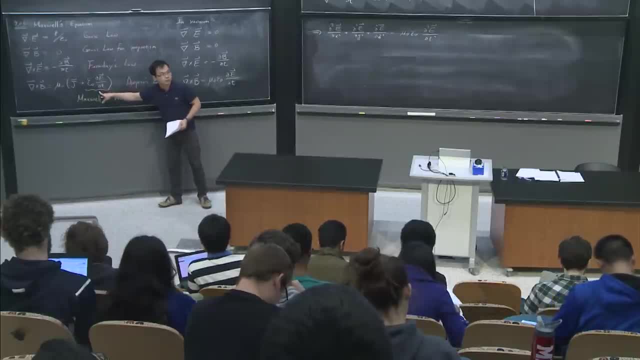 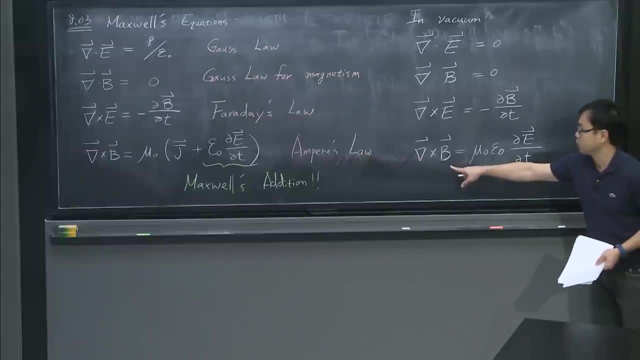 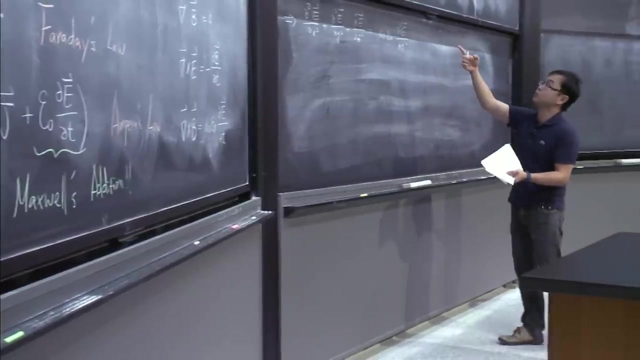 As you can see, if I don't have this additional term, if I take the displacement curve current from Maxwell, what is going to happen? This curl B will be equal to 0. Right, So what is going to happen to this identity? 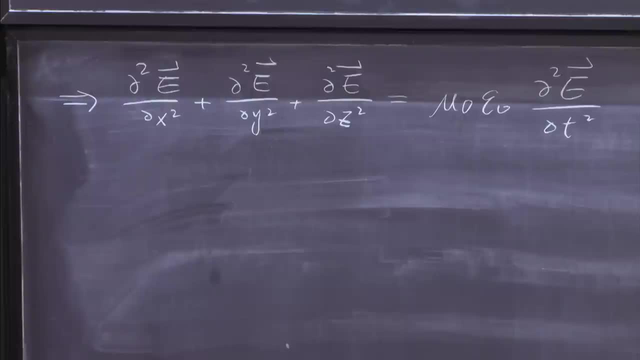 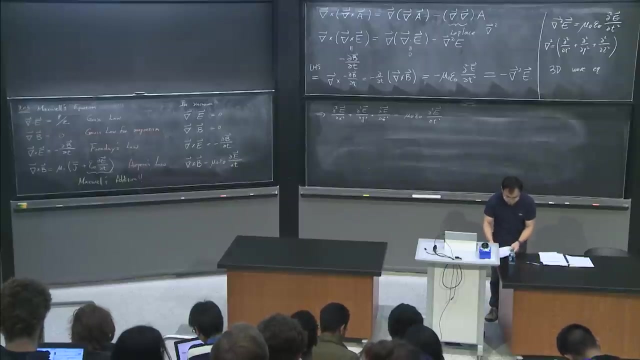 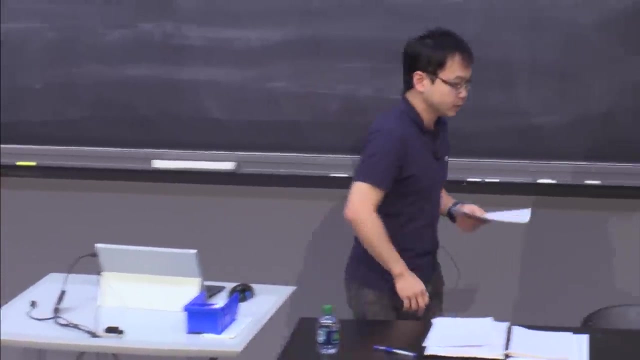 So this left-hand side part will be equal to 0. There will be no electromagnetic waves. OK, So this is really thanks to Maxwell's work And this is actually really an equation which changed the world right, Because that actually gives us a lot. 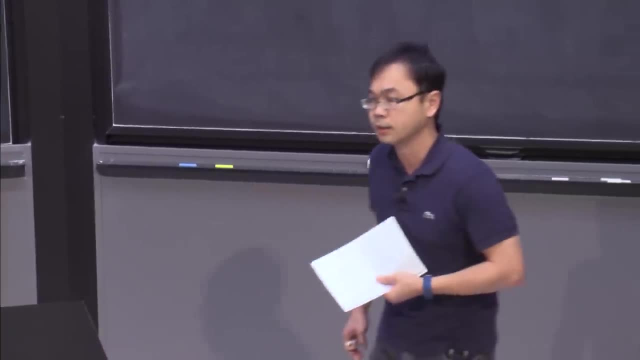 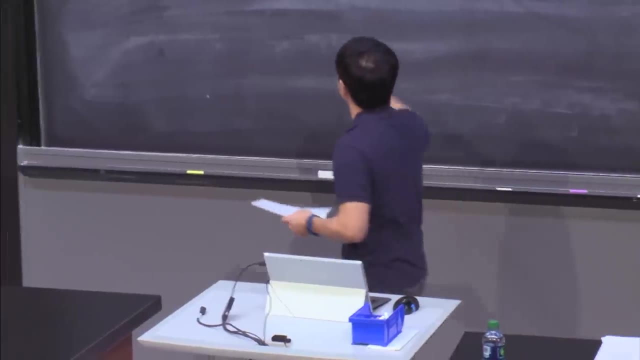 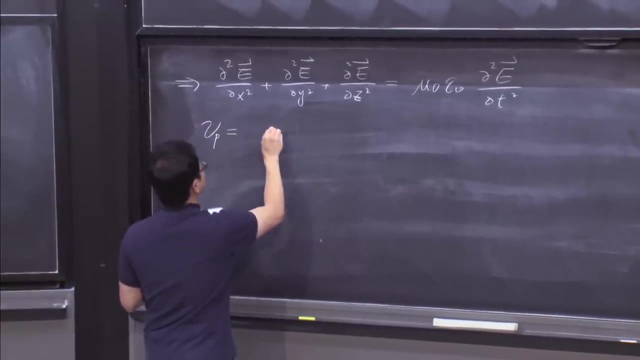 of insights about how we can send energy, how we can actually understand the phenomena related to light. So what is actually the velocity of this wave equation? So velocity vp will be equal to. we usually call it c, right, Because you have been using this constant for a long time. 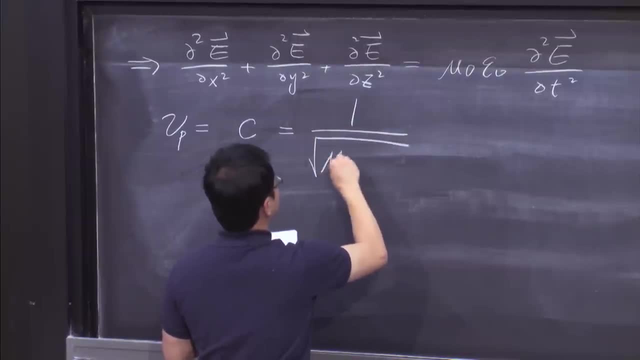 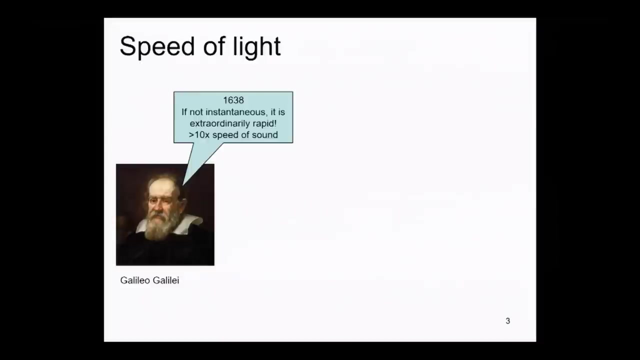 And that will be equal to 1 over square root of mu 0, epsilon 0.. OK, And to measure the speed of light, it takes a long time to achieve that. OK, Let's actually take a look at the history. 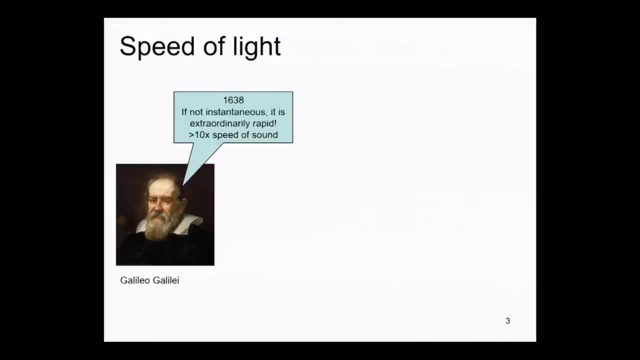 So the first attempt was done by Galileo, So 1638,. he was doing an experiment And he was trying to extract the speed of light, But he was not super successful. So his conclusion was that if the speed of light is not instantaneous, then it is actually super fast. 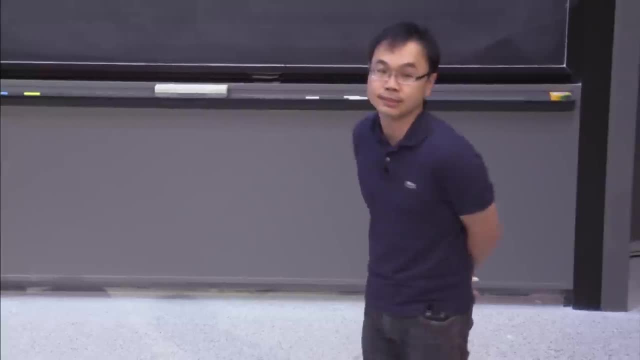 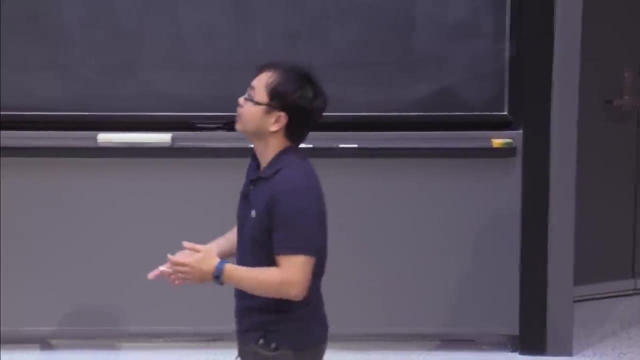 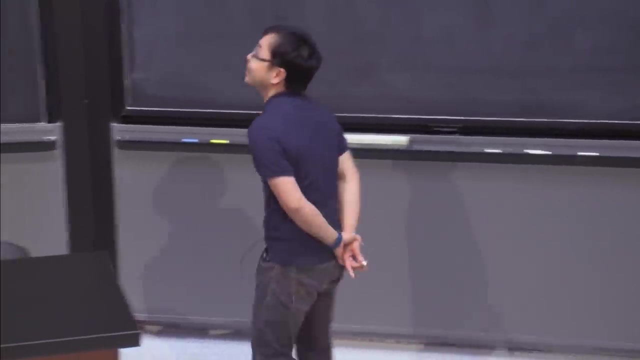 It's actually at least 10 times faster than the speed of light. So at least he said, OK, this is super awesome, very fast, OK, And at least 10 times the speed of sun, not the speed of light. 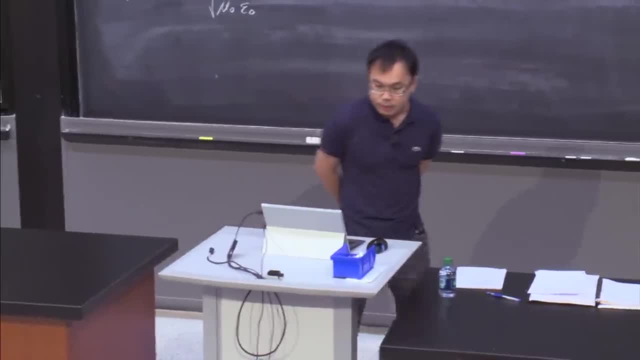 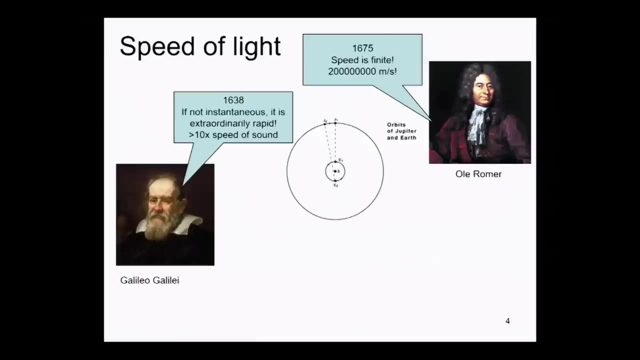 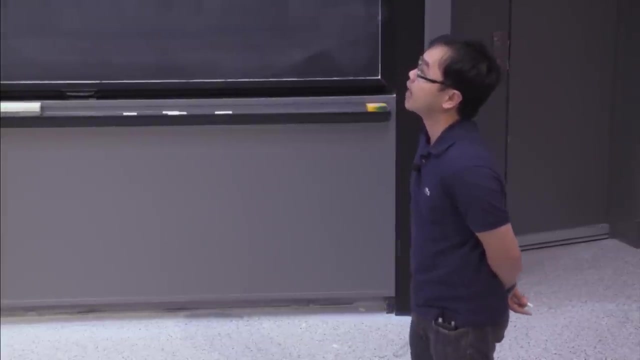 OK, All right, So that's what he found, And later Euler actually made a approach to use the orbit of Jupiter. OK, So basically he used the Jupiter and Jupiter's satellite to measure the speed of light. So when the Earth is closer to Jupiter, 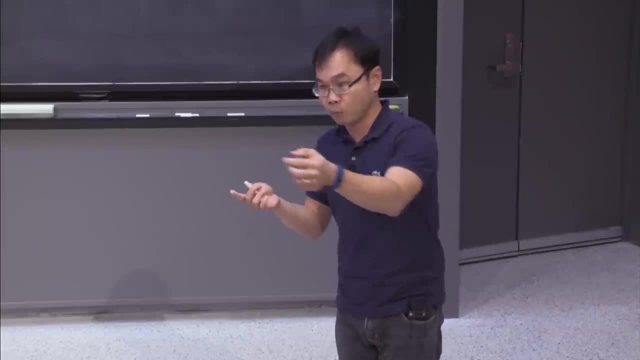 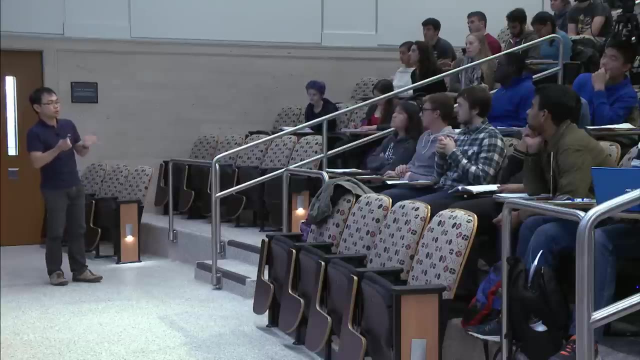 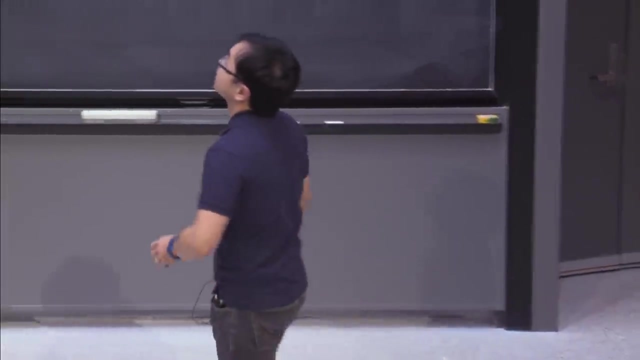 then somehow, the satellite of Jupiter appears faster than when the Earth is actually away from Jupiter, right? Because the light has to travel through additional time, two times of the radius of the orbit of the Earth, right? So basically, that's actually the method he was using. 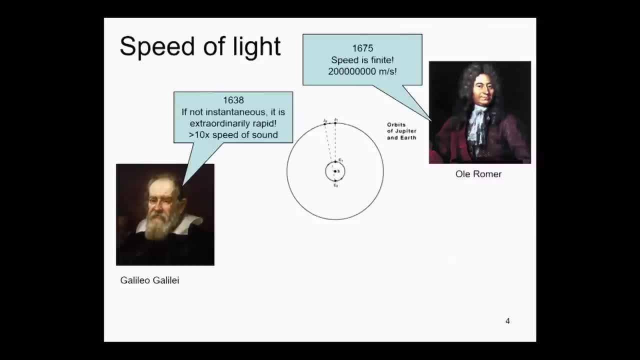 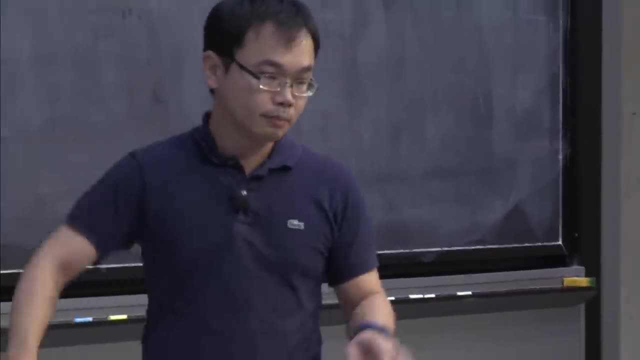 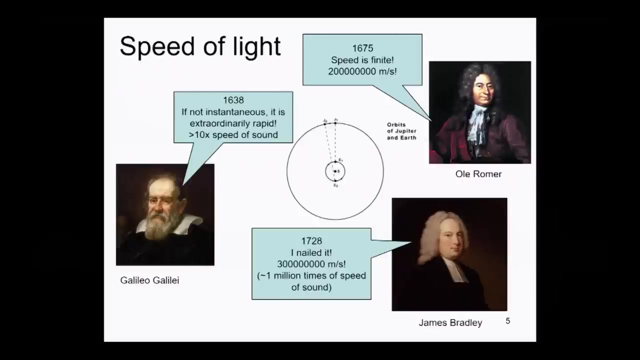 And he is actually making the first quantitative, the first measurement of the speed of light, And the number he found is like 2 times 10 to the 9 meter per second. OK, So finally, again using the star, the observation. 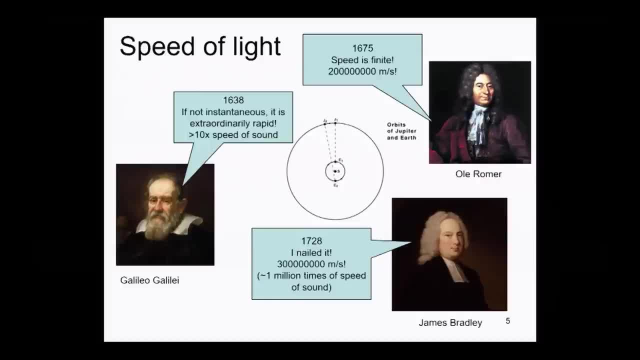 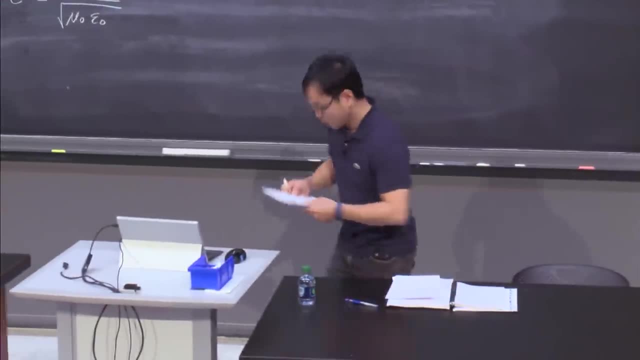 star as an operation, as a tool to actually calculate the speed of light. James actually nailed it And he found a value which is really close to the current understanding of the speed of light, which is 3 times 10 to the 9 meter per second. 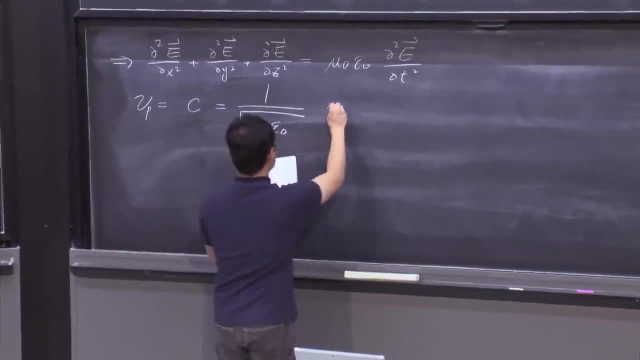 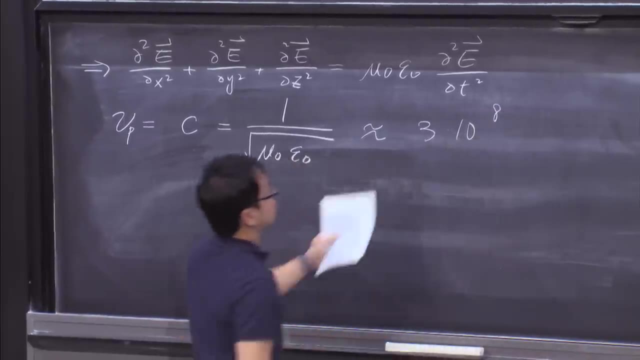 OK. So if you calculate using all those constants here, you will be able to see that indeed, from Maxwell's equation you get: oh, it should be 3 times 10 to the 8, not to the 9.. 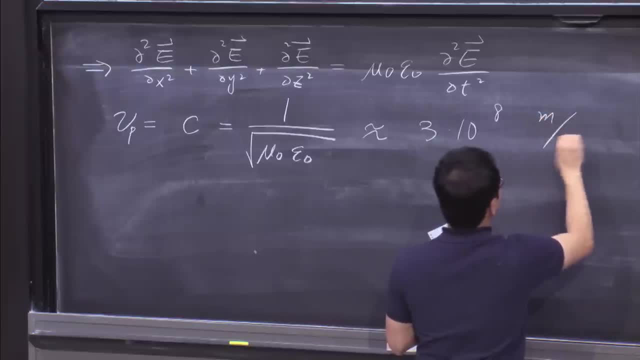 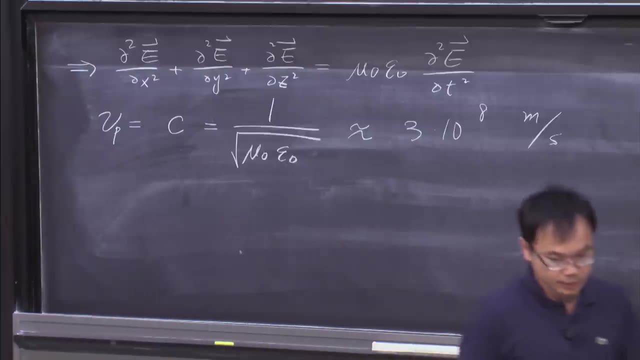 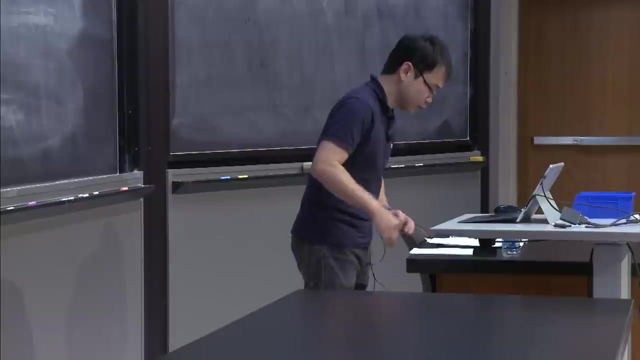 OK, I was saying 10 to the 9.. It should be 3 times 10 to the 8 meter per second. OK, So indeed, this equation is actually predicting the speed of light to be 3 times 10 to the 8.. 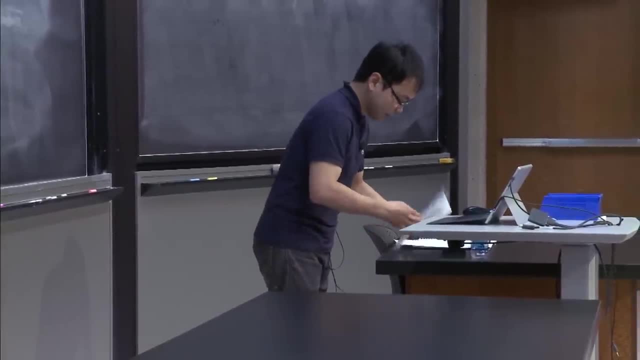 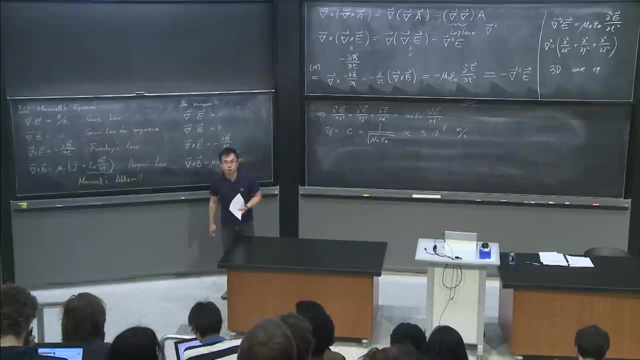 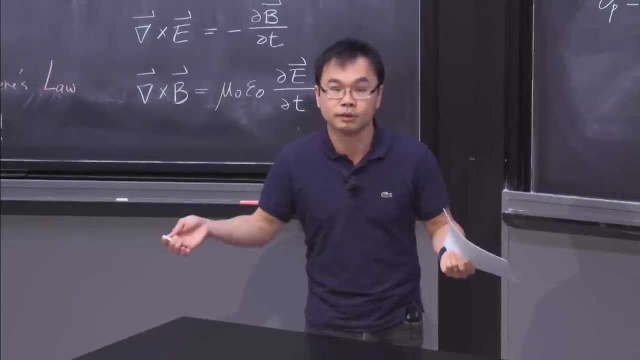 It's actually matching the experimental result. OK, So that is actually pretty nice And you may ask a question, right? So wait a second. You say that this is actually the electromagnetic wave, right? So that's actually what I was talking about. 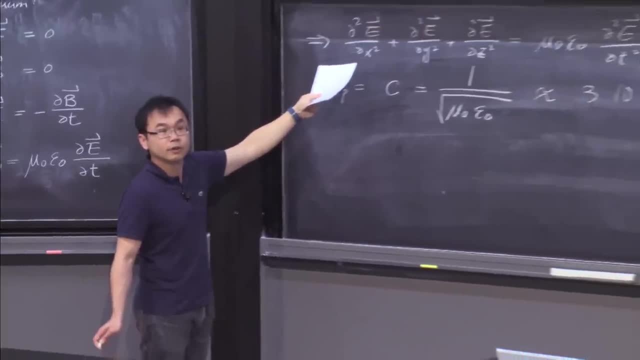 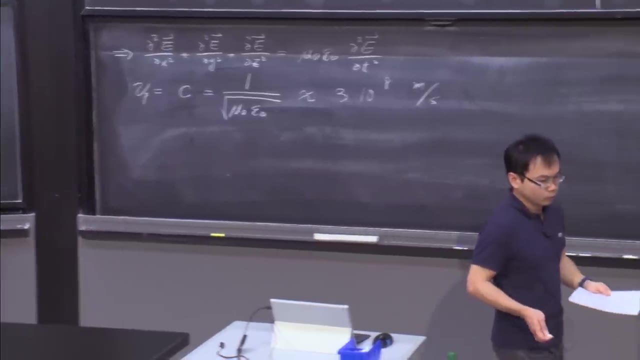 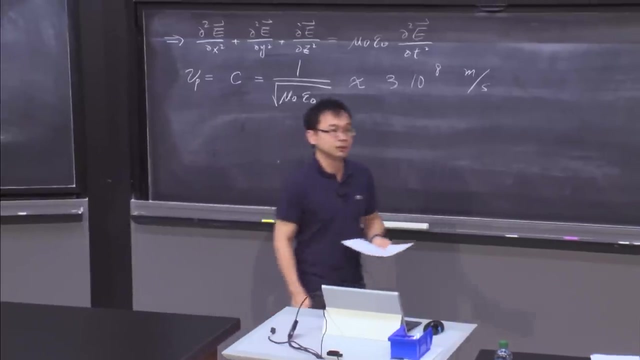 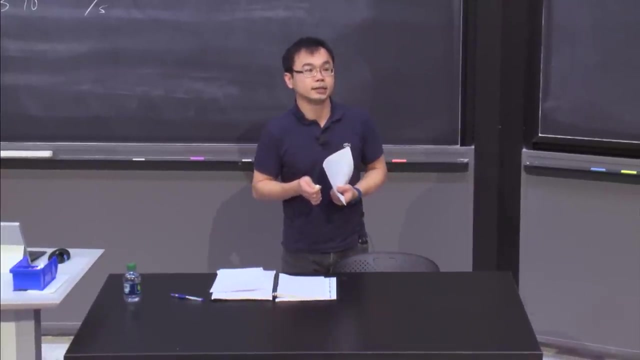 But this equation only talk about electric field, right? What is happening to the magnetic field? Right? So can we actually choose arbitrary magnetic field? Is the magnetic field also obeyed? Is the magnetic field also described by the three-dimensional wave equation right? 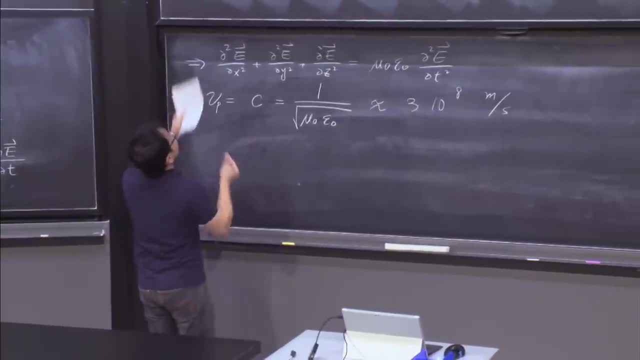 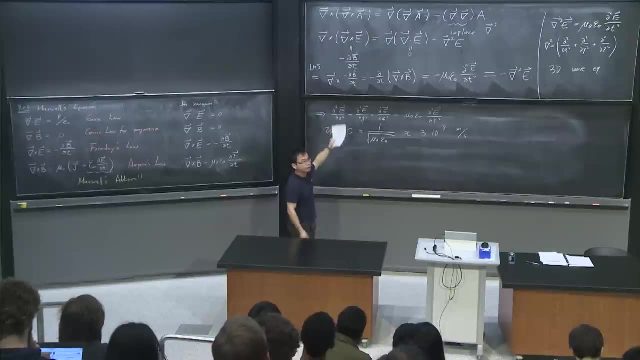 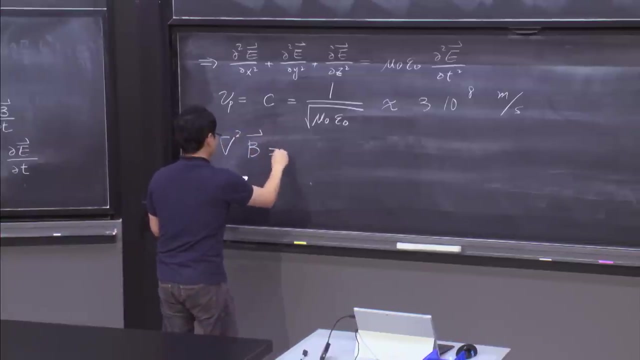 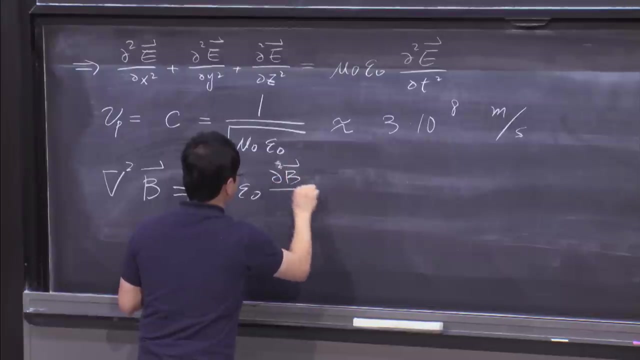 The answer is that, indeed, you can actually do the same exercise. You can now, instead of plugging in electric field, you can plug in magnetic field And you will extract exactly the same conclusion. You will conclude that del squared b will be equal to mu 0, epsilon 0. partial squared b, partial t. 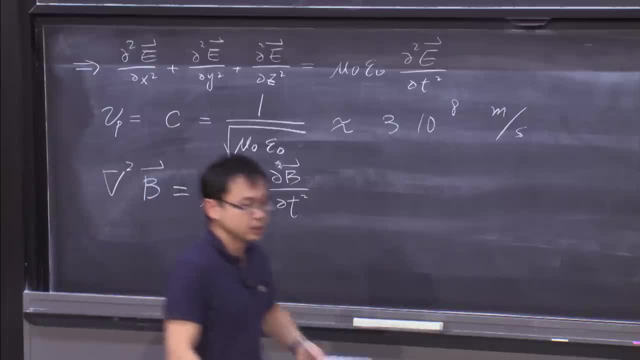 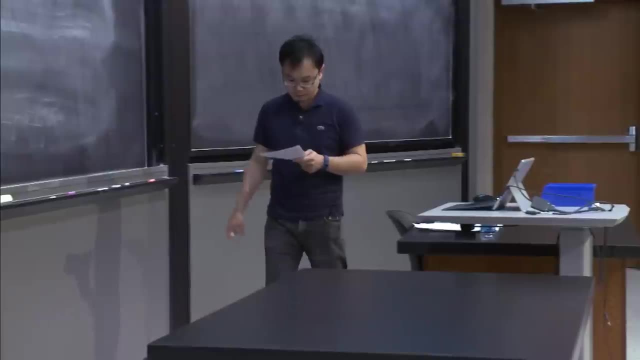 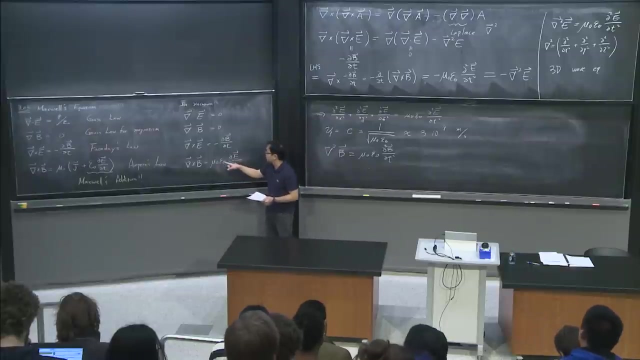 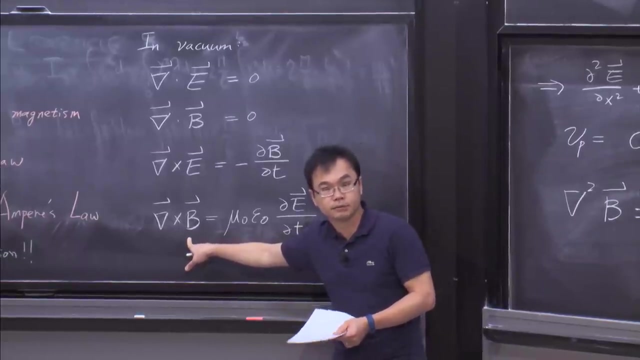 squared, OK. So it is actually very important to see that the magnetic field also obey this wave equation, OK. And also from Maxwell's equation, OK, you can see that the changing electric field will produce a current around magnetic field. The same thing also happens here. 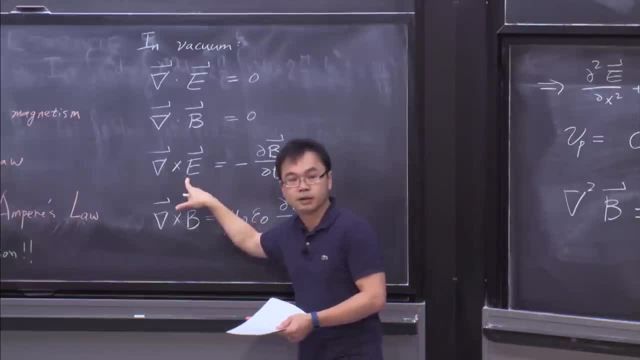 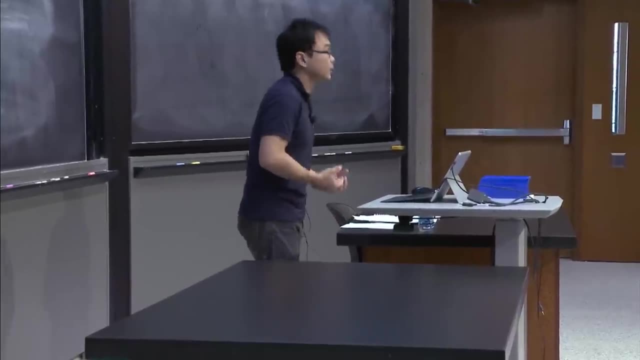 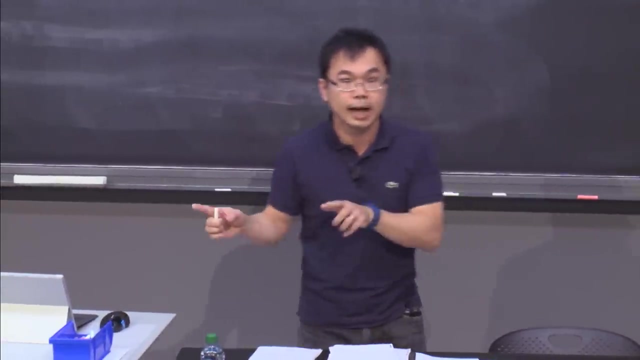 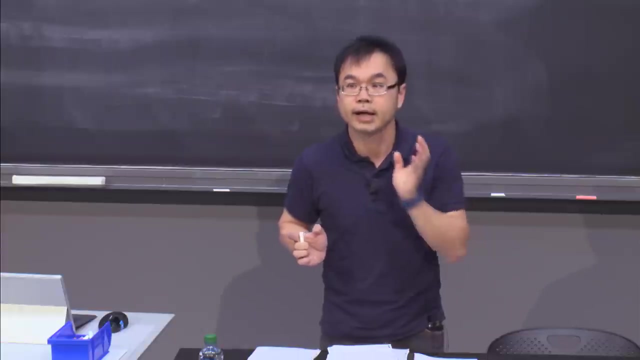 The changing magnetic field also produce a current around electric field, right? So what does that mean? That means electric field create magnetic field, Magnetic field create electric field, And this happens all the time. Therefore, one cannot live without the other. OK. 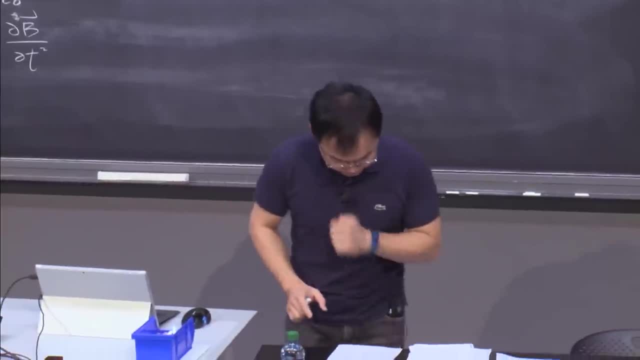 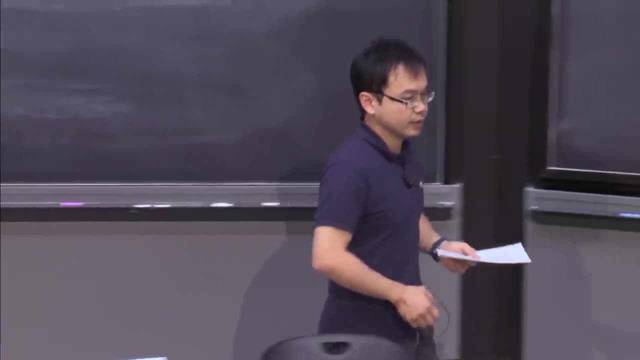 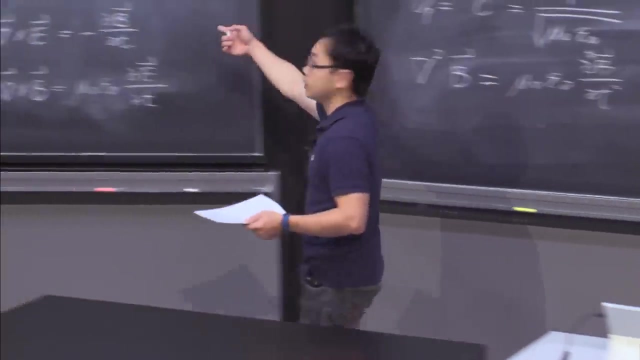 They are living together, They are all together forever. OK, All right. So what is actually oscillating is actually both electric field and the magnetic field, right? So you may ask: OK, we are talking about vacuum, right? What is actually oscillating? 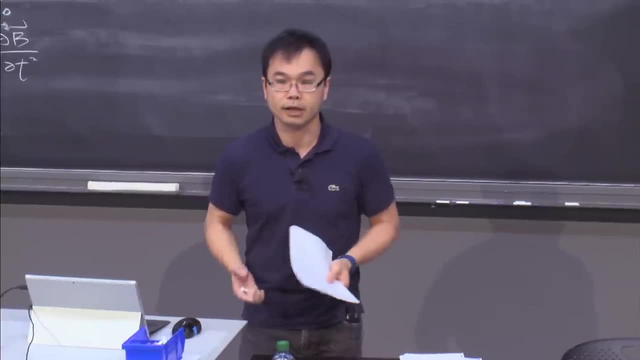 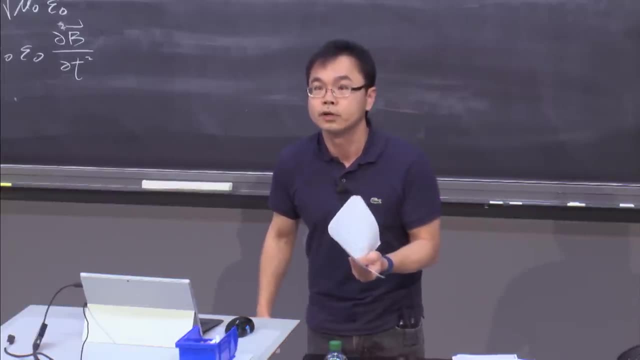 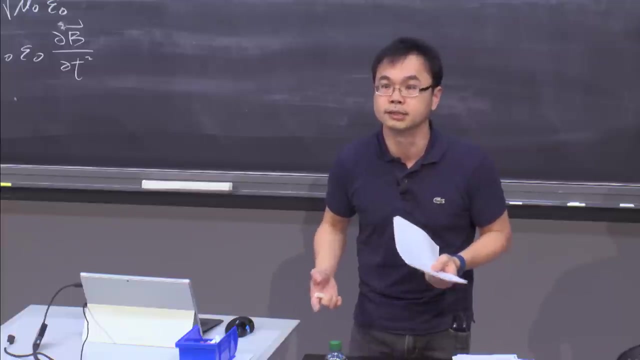 Vacuum means there is no material, no charge, no whatsoever in vacuum, right? So what is actually oscillating? Who is oscillating? It's the electric field and the magnetic field. OK, It's this so-called field, all those vectors which 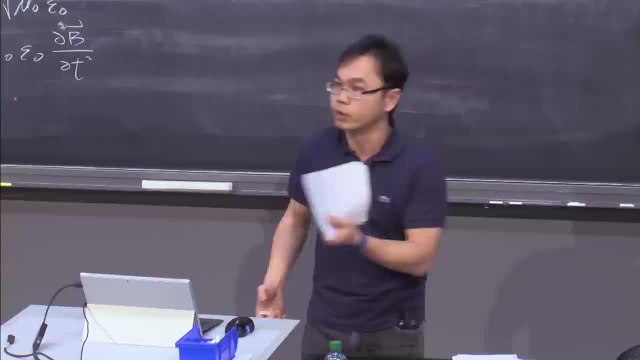 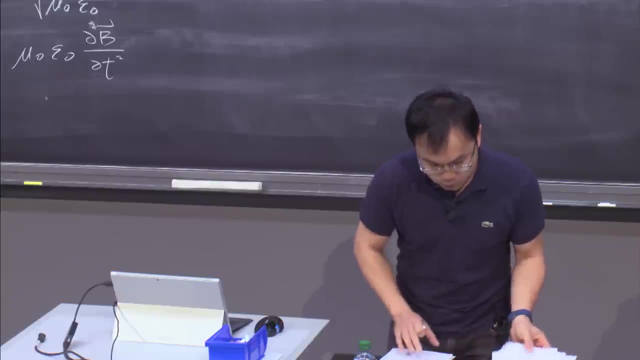 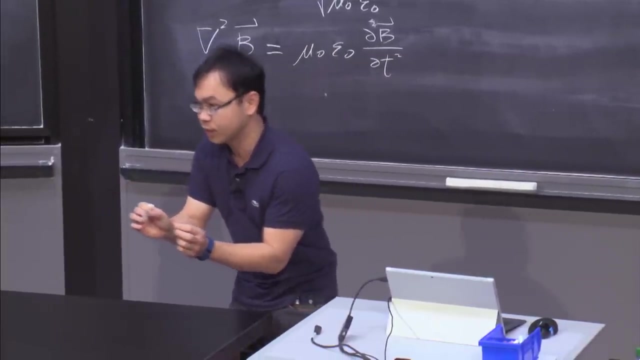 are actually oscillating. It's not the material, but all those vectors associated with the space which is actually oscillating up and down. OK, All right. So originally I would like to show you a pulse of light in front of you and show you. 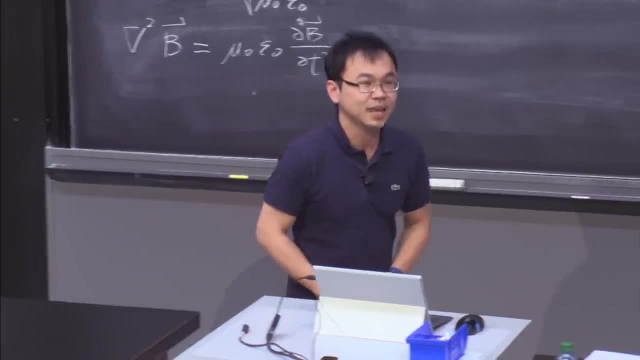 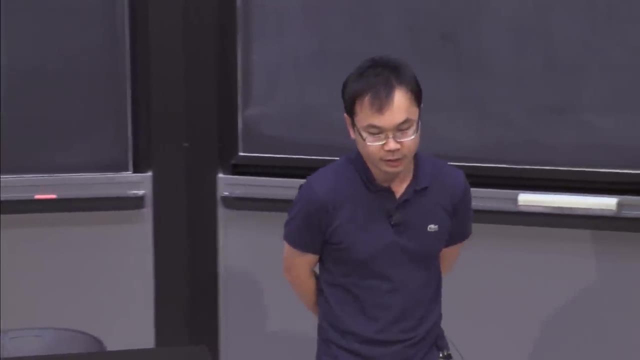 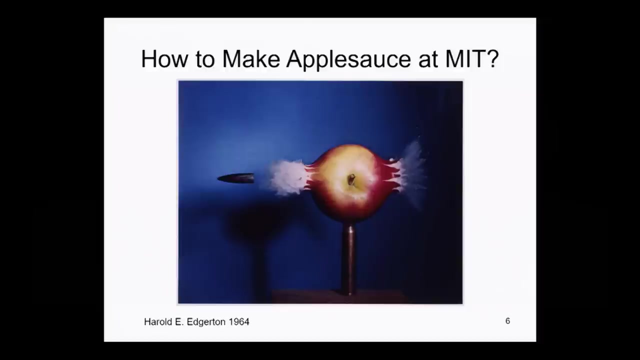 that it's moving, but it's still too fast, Right? So I couldn't do that. Fortunately, we have photos. which photos are actually collected? recorded photons emitted from the object, Right? So this is actually how we make apple sauce at MIT. 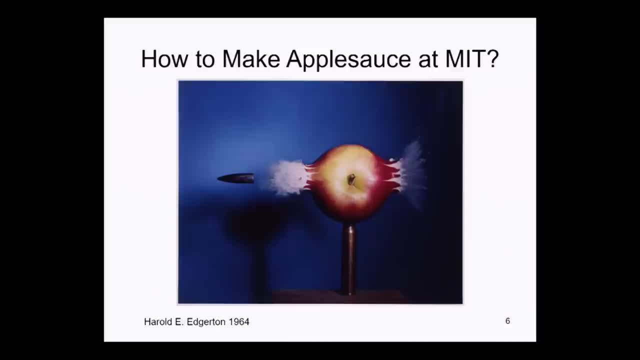 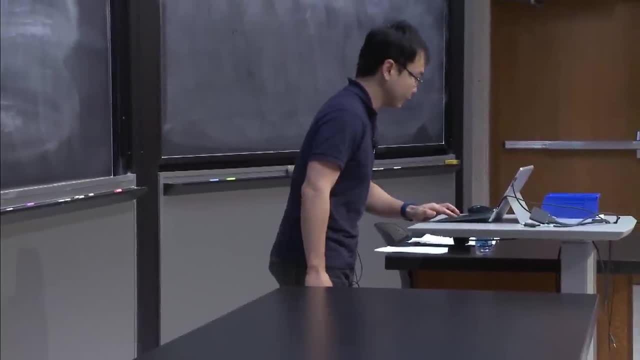 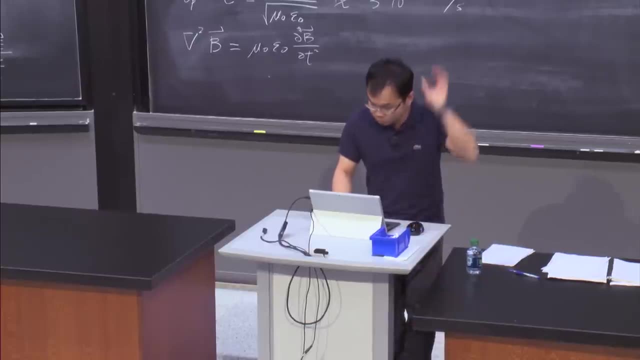 We should put it through the apple. Then we have the sauce, But not sure if that's tasty enough or not. But that's how we do it in MIT, MIT style. OK, And the good thing is that this kind of technique is improved dramatically these days. 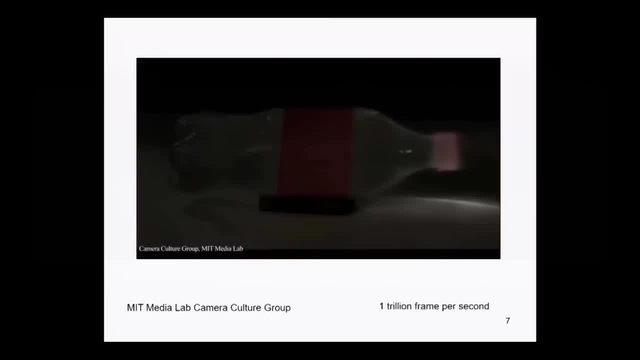 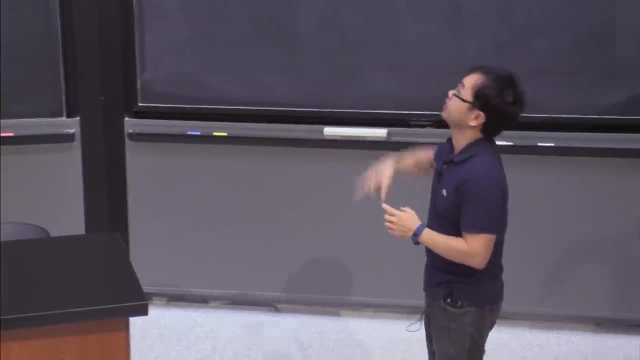 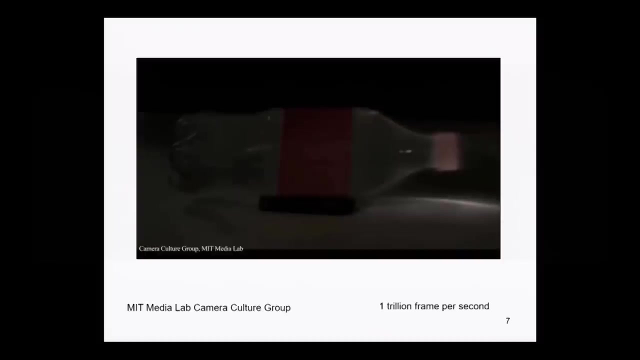 I would like to show you a short video, which is actually a recording video of a recording experiment which you shoot some beam of light through some plastic container, OK, OK. And the speed of this recording corresponds to 1 trillion frames per second. 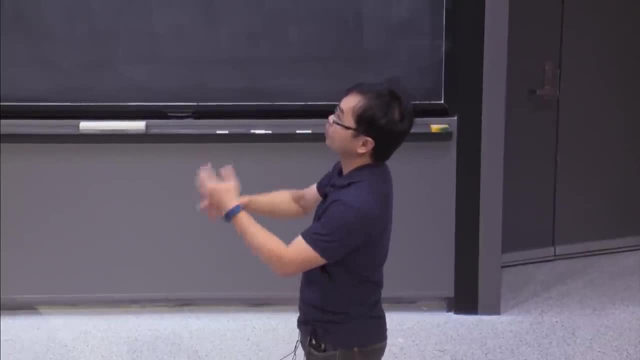 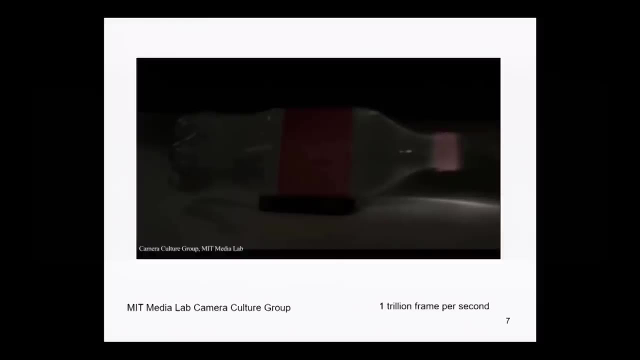 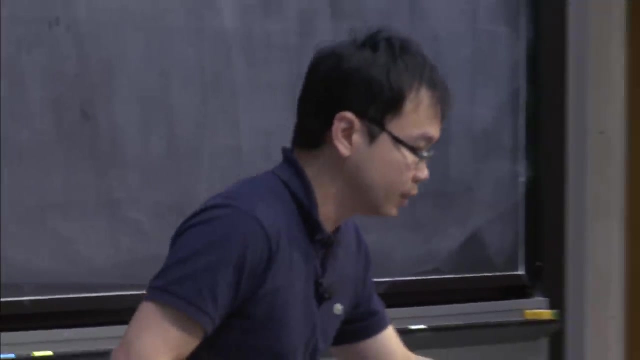 OK, So this is super fast recording. And then we contract the propagation of the light through this bottle, And this is actually the credit to the Media Lab Camera Culture Group. OK, And let's take a look at the video. Just one second. 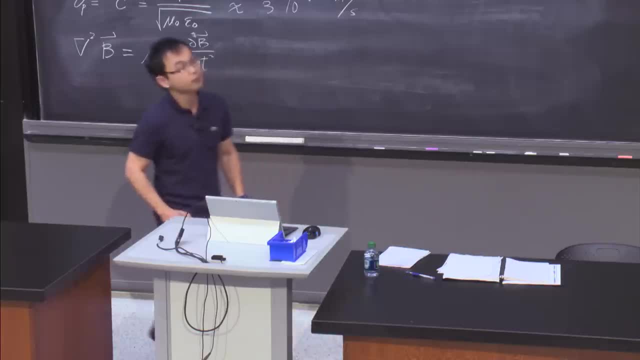 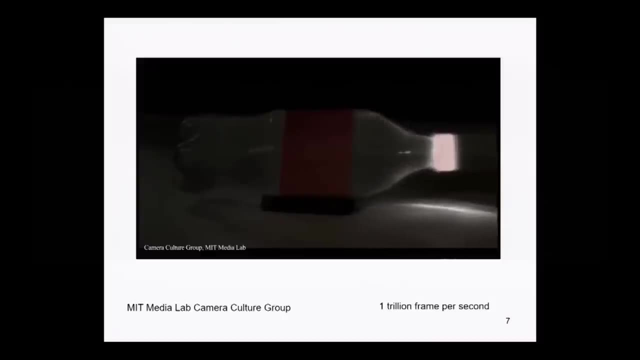 OK, so this is actually recording at 1 trillion frames per second, So you can see that there's a light pulse, very short pulse- here, And it's really passed through the bottle And it can be recorded with the technique created by Media Lab. 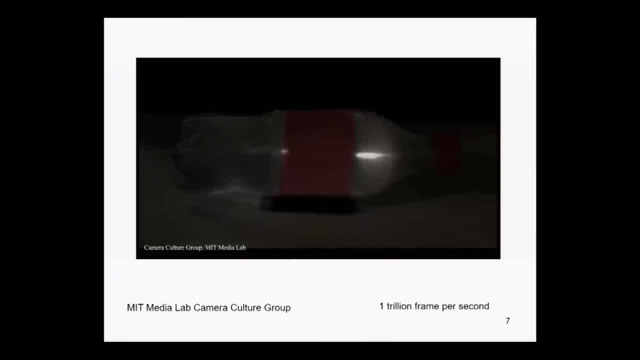 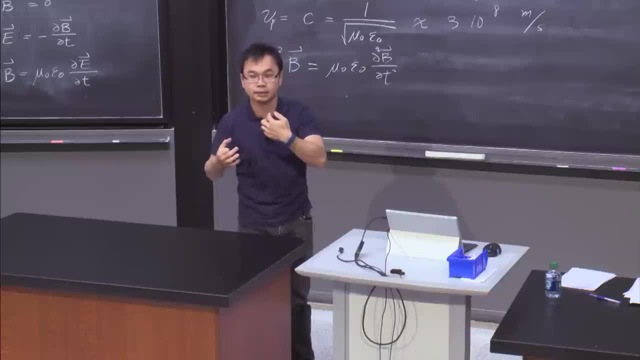 OK, So you can see that the pulse is really propagating through it, And the reason why we can see the pulse is because their air, their material, which actually changes the direction of the light, OK, And therefore those are recorded by the camera. 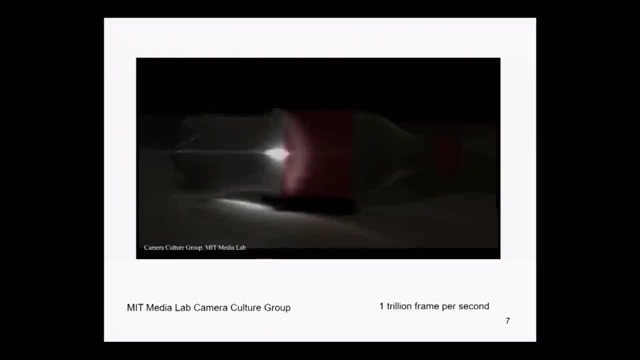 And if you take the trillions of frames of this thing and put them together, then basically they take many, many frames and put them together to recontract this movie. So, as you can see, indeed you can see- the propagation of the light through this kind of video. 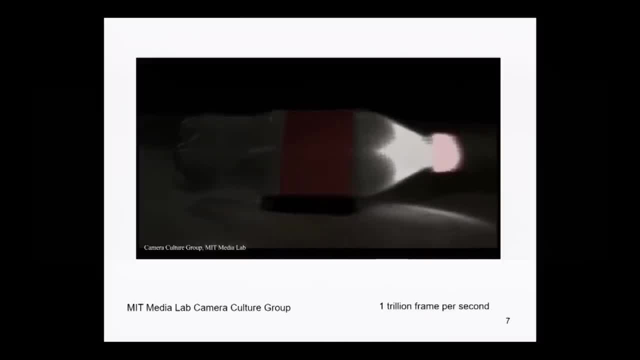 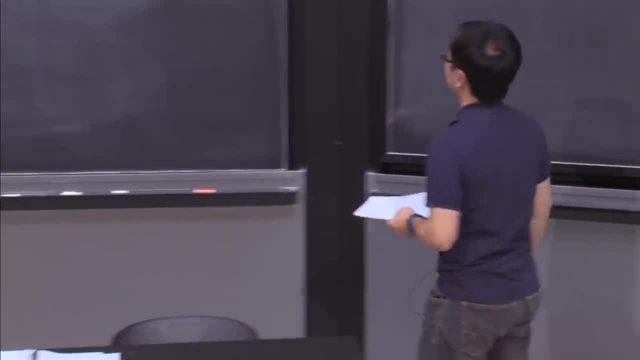 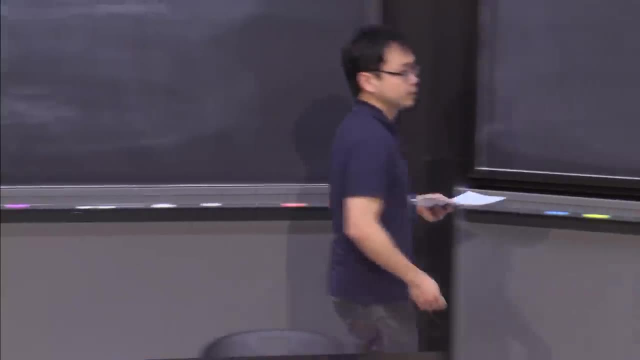 OK, So I hope you enjoyed this video, And that's actually So. let's take a look at some concrete example which make use of the wave equation which we actually derived here. OK, So let's consider a plane wave solution. 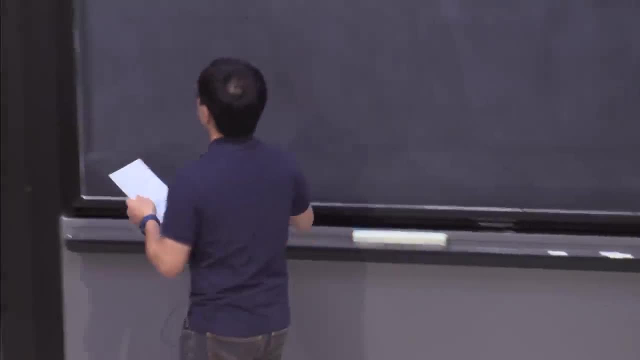 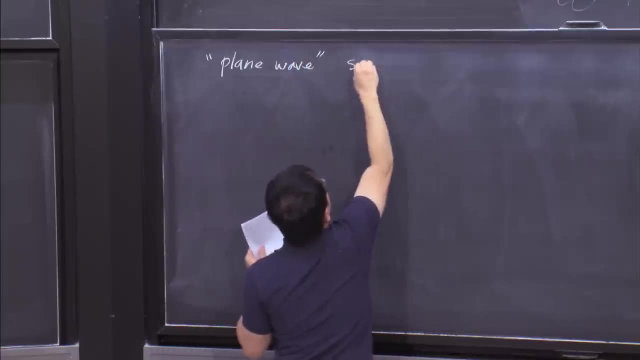 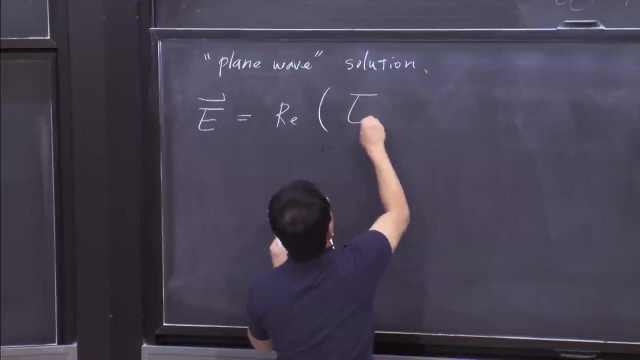 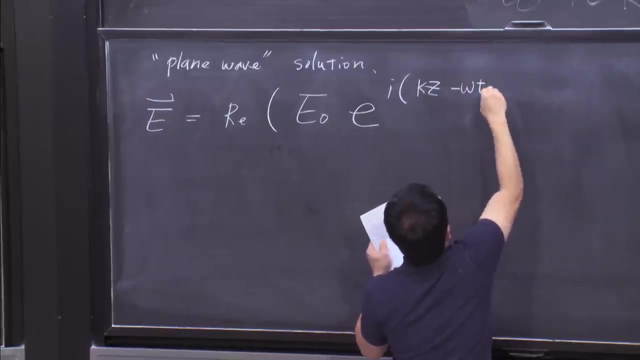 Right, Since we are entering a three-dimensional world, so let's actually consider so-called a plane wave. OK, So in this example I am considering, the electric field is actually equal to the real part of E0, exponential i kz minus omega t. 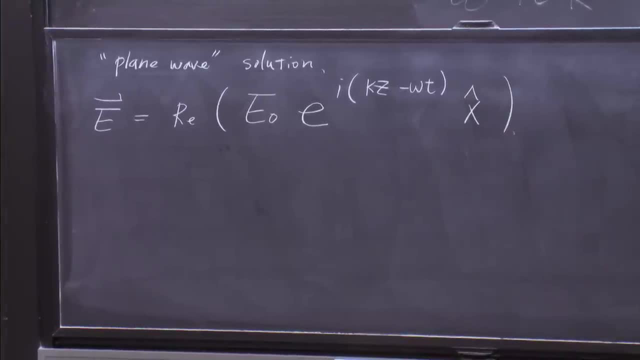 And this electric field I actually consider here is in the x direction. OK, And if I write all the terms from this expression explicitly, what I am getting is: OK, the x component will be E0, cosine, kz, minus omega, t, 0 and 0.. 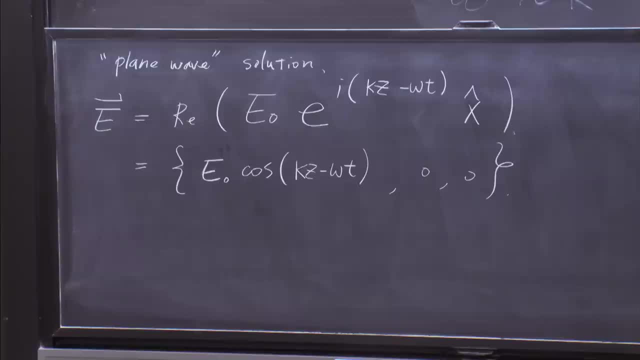 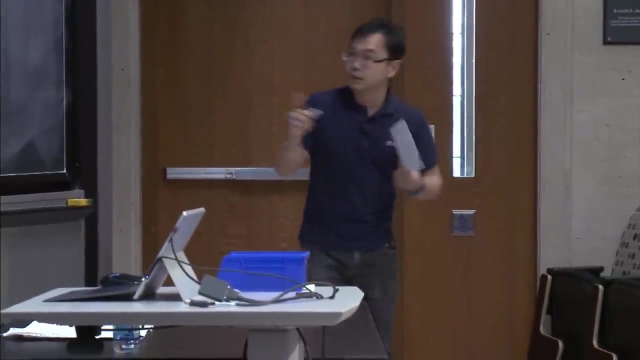 Right. So what does this mean? What is actually a plane wave? The plane wave, basically, is actually fielding the whole space. What I mean by plane wave is that I have a whole space with electric field. This electric field only have one direction. 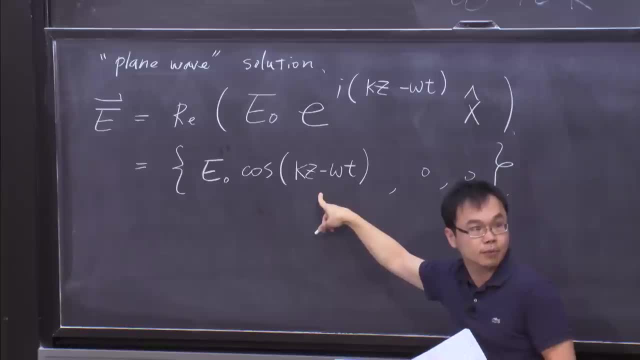 have non-zero value, which is x direction in the example, OK, And in the other direction the magnitude is actually equal to 0.. OK, So that's actually what I mean by plane wave, And also the electric field is fielding a whole space. 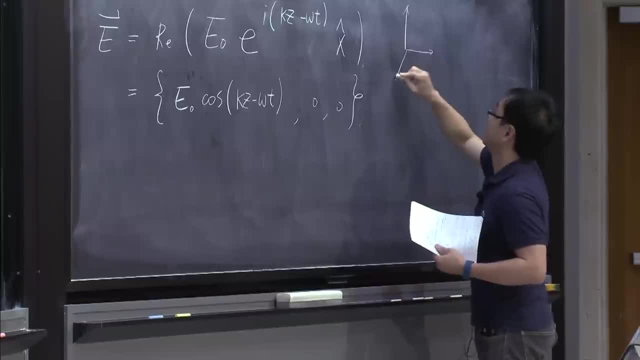 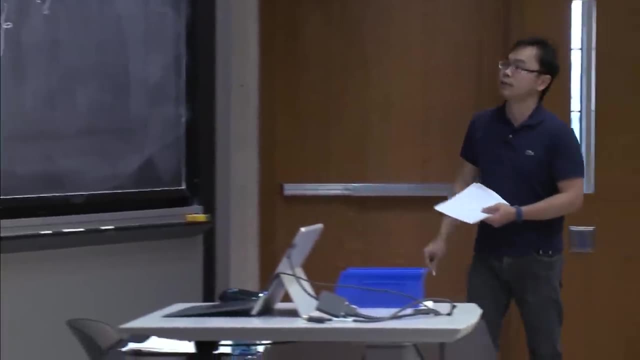 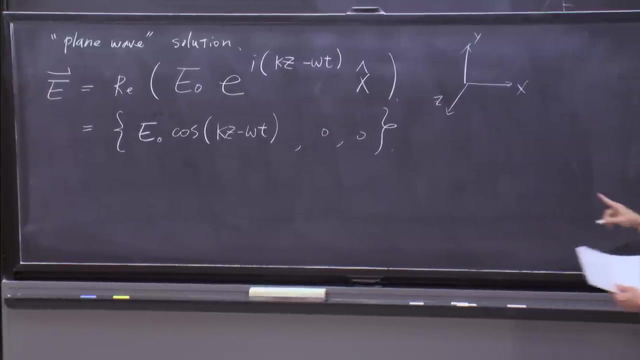 And this is in the discussion in the example which I discuss here, And if I define my coordinate system like this: x is in the horizontal direction, then that means everything is actually all the electric field is actually pointing toward the x direction in this coordinate system. 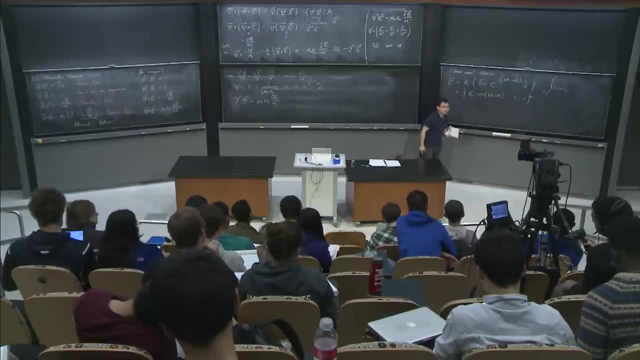 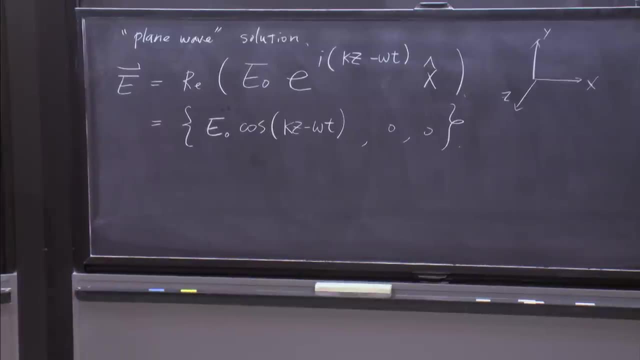 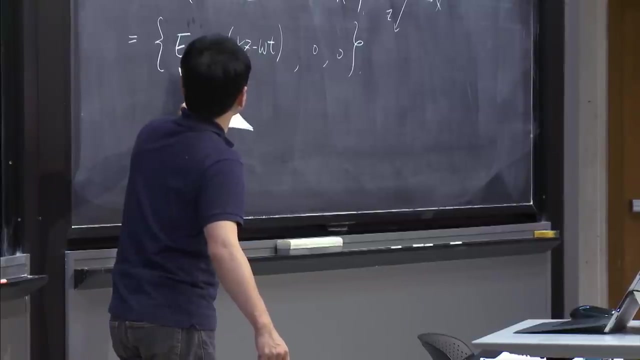 OK, So we have discussed progressing wave in the past few lectures, Right? Can somebody actually tell me the direction of propagation of this plane wave? So the hint is that this is actually equal to E0.. The magnitude of the x component is equal to E0. cosine kz. 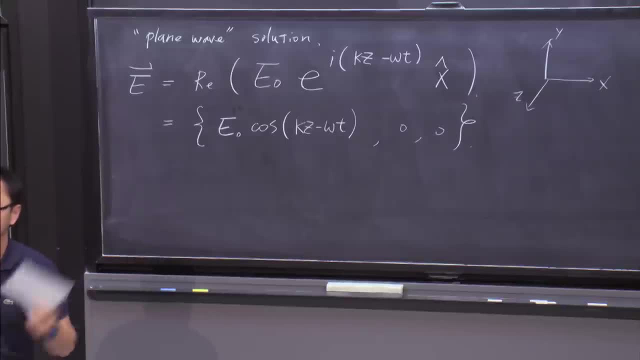 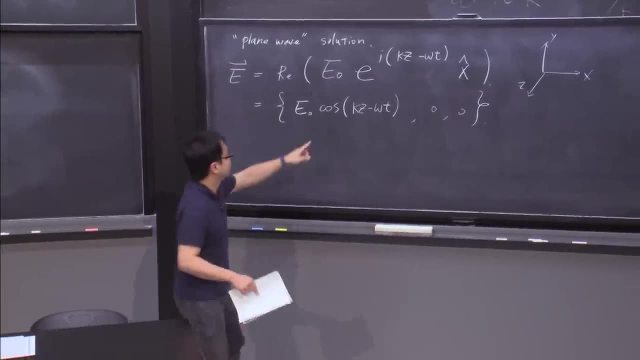 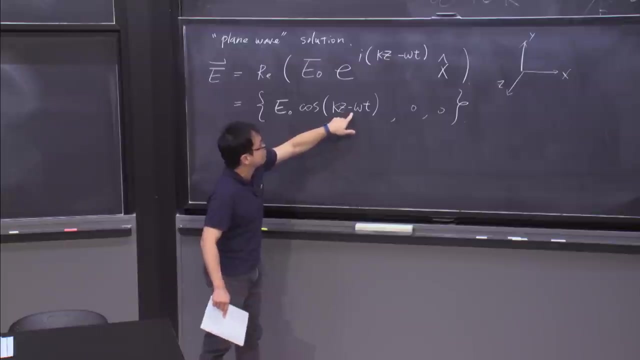 minus omega t. Right. What is actually the direction of propagation of the electric field? It's in the z direction. Yeah, Very good, Because we know that this is actually going in the positive z direction. Right, Because this is actually kz minus. 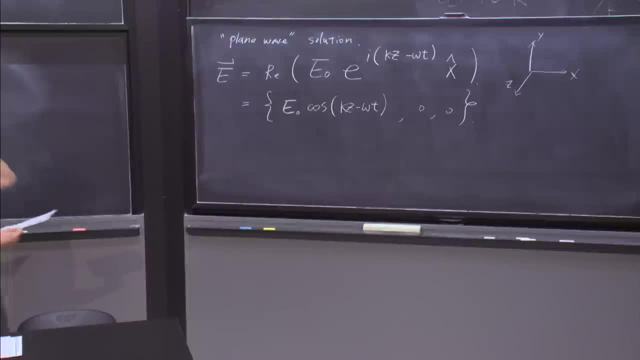 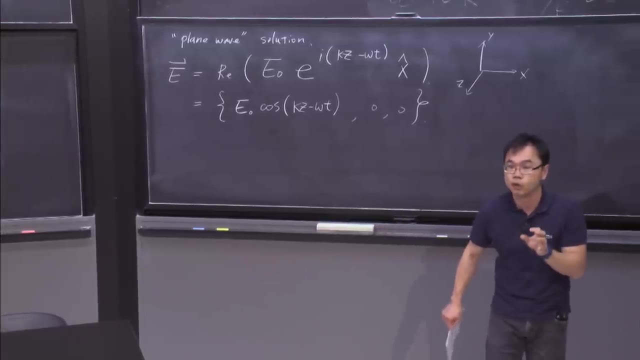 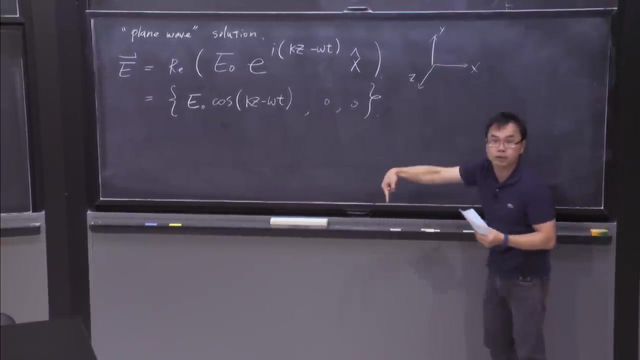 There's a minus sign, omega t. Therefore it's going to work. the positive z direction, not x direction Or x direction, is where the electric field is pointing to And the direction of propagation is toward the z direction. OK, So there's a difference. 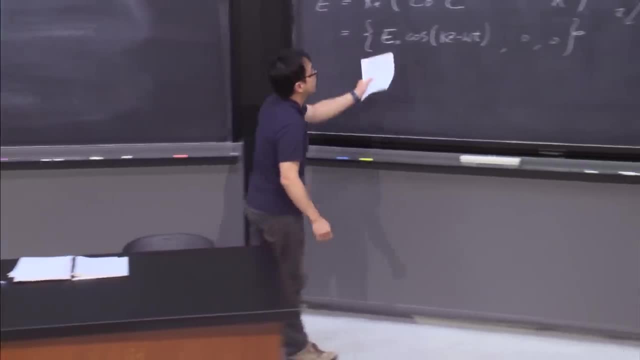 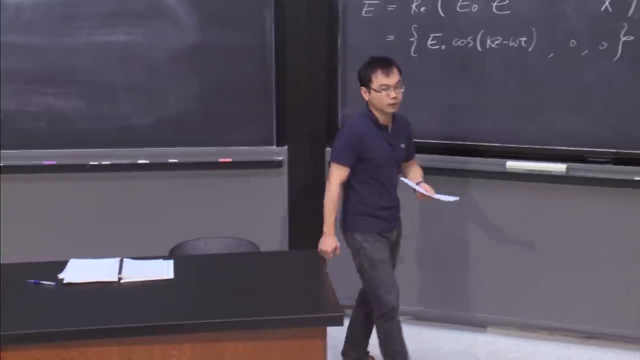 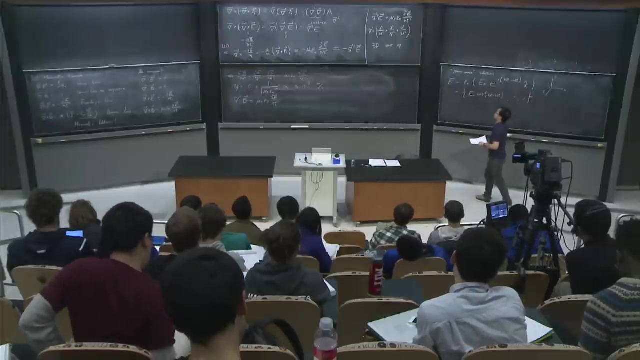 OK. So first thing which I would like to do is to check if this so-called plane wave solution actually satisfy the equation, the wave equation which we derive here. Right, The del squared E equal to mu 0, epsilon 0 partial squared E. 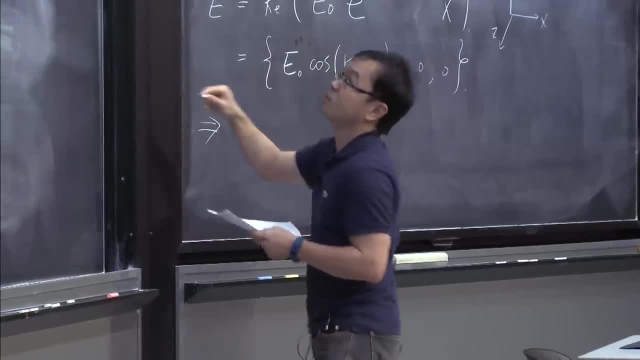 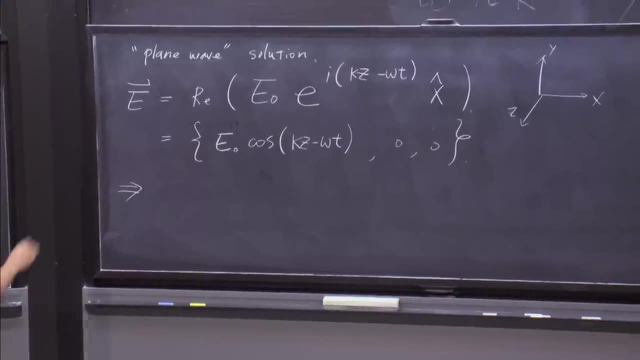 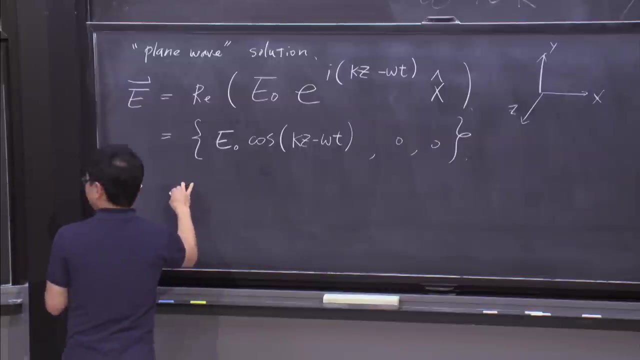 partial t squared, So I can now plug that in to that equation. I can now plug in to this equation. If I plug in the plane wave solution which I have here to that equation, basically I can get the left-hand side. 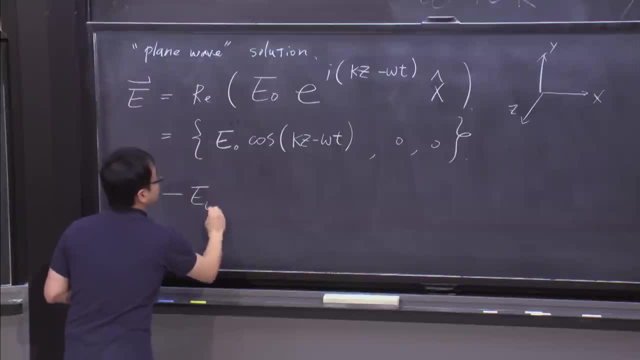 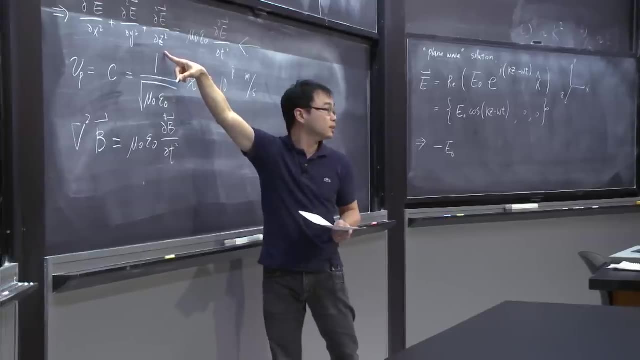 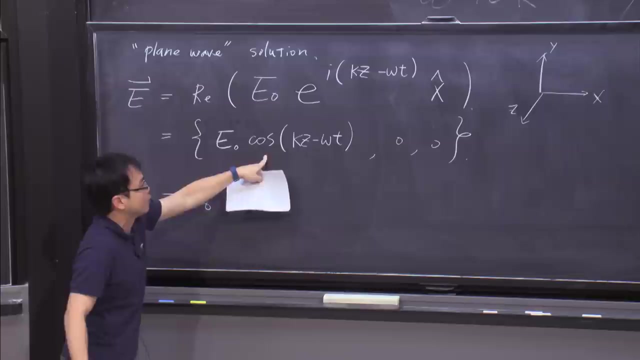 The left-hand side of the equation, you will get minus E0.. OK, Only one term which contribute is the partial squared E, partial z squared term which contribute Because the magnitude of the electric field only depends on z and t Right. Therefore, you get minus E0. k squared cosine kz minus omega t. 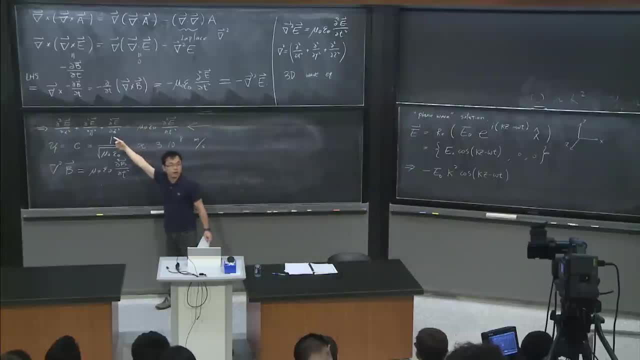 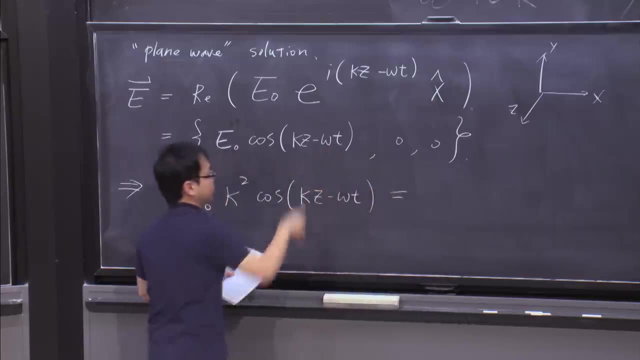 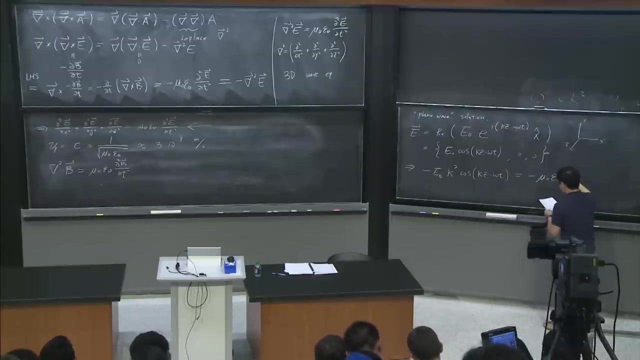 in the left-hand side of the wave equation. OK, How about the right-hand side? Right-hand side, basically, you are taking partial derivative with respect to t. Basically you get minus mu 0.. Mu 0, epsilon 0 are copied from that formula there. 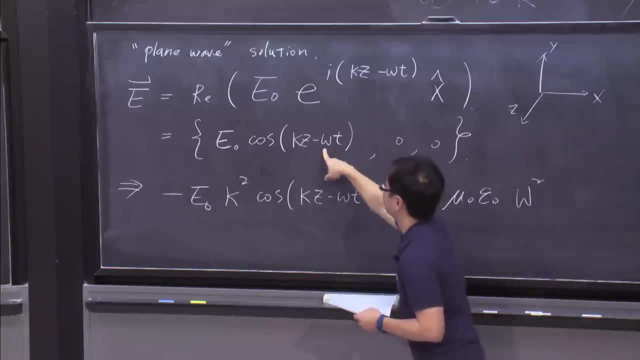 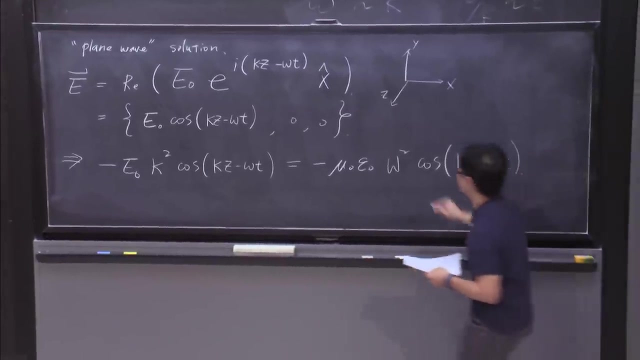 And you basically get omega squared out of it because of the partial squared, partial t squared operator And you basically get cosine kz minus omega t. And of course I missed the E0 term. E0 should be copied from there, OK. 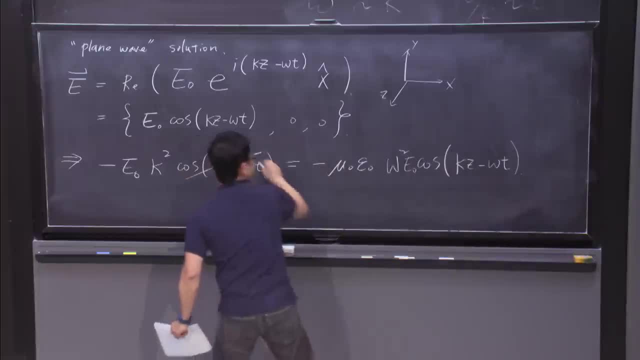 All right, So now I can show that. OK, this cancel. Basically, this is the same cosine: kz minus omega, t Right And E0 also cancel, And I can cancel the minus sign. OK, What I'm going to get is k squared. 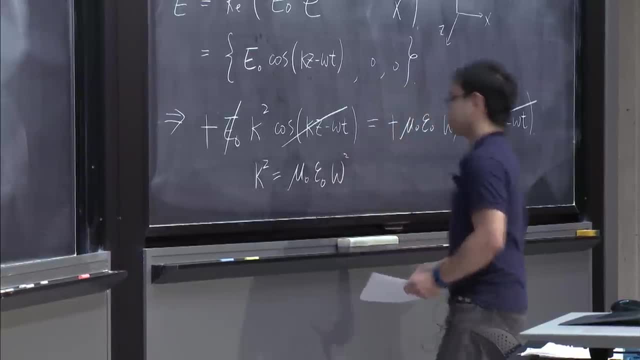 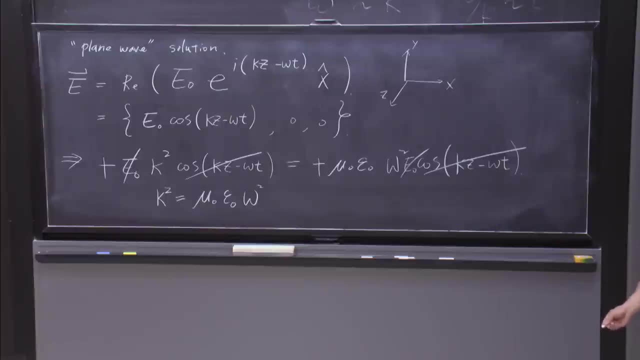 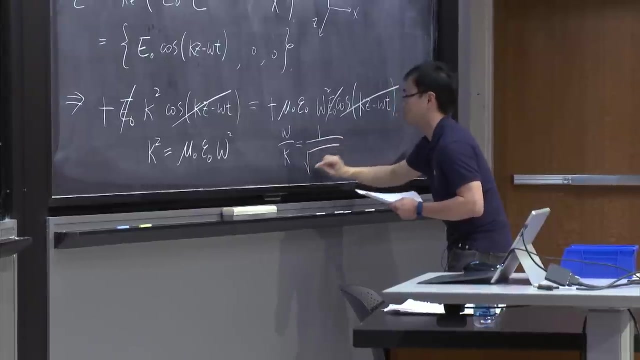 times mu 0, epsilon 0, omega squared. OK, So that means there should be a fixed relation between k and omega, which is actually: omega over k will be equal to 1 over square root of mu 0, epsilon 0. And this is equal to c. 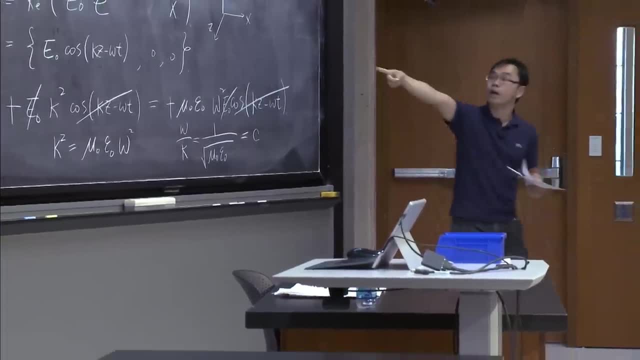 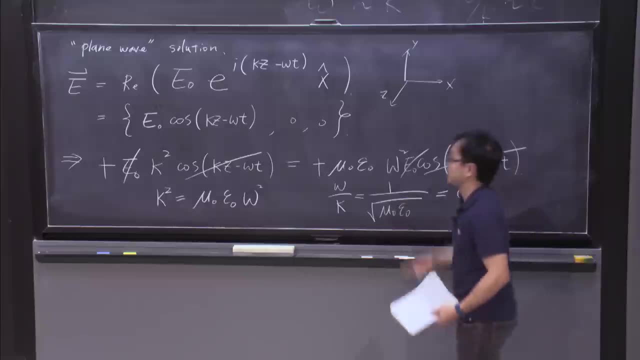 If this is satisfied, then the plane wave is a solution to the wave equation. OK, Only when this is actually satisfied, OK, Otherwise you can write down arbitrary plane wave equation, But they are not the solution of that equation. from Maxwell's equation. 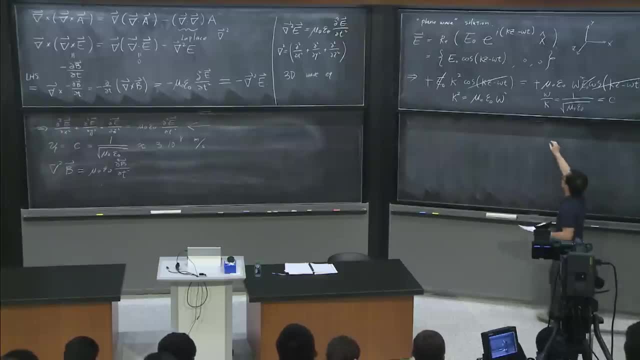 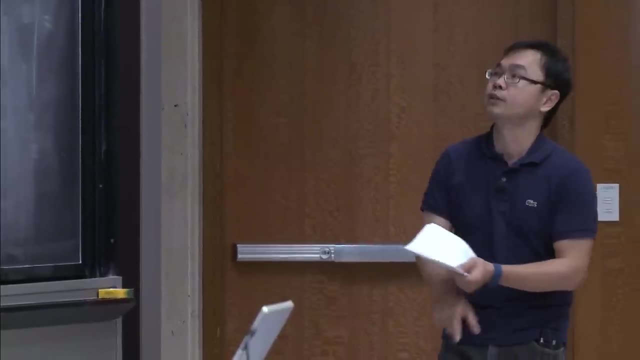 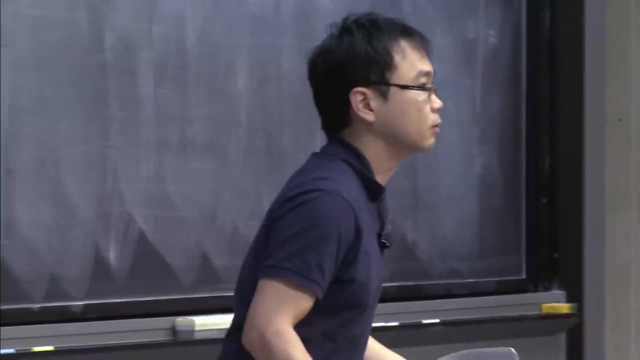 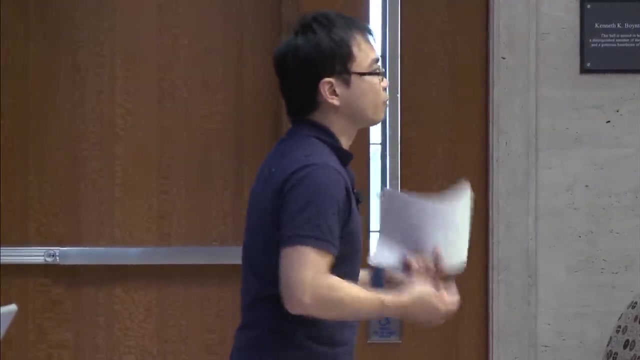 OK, So now I have derived the electric field and also know the relation between omega, the angular frequency, and the k, the wave number. OK, So now what about magnetic field? Right? So I just mentioned before, right, Magnetic field cannot live without electric field. 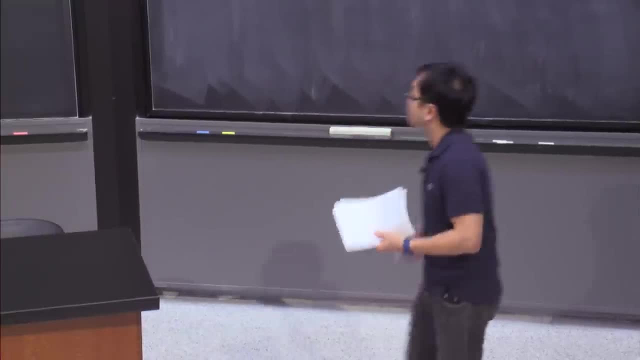 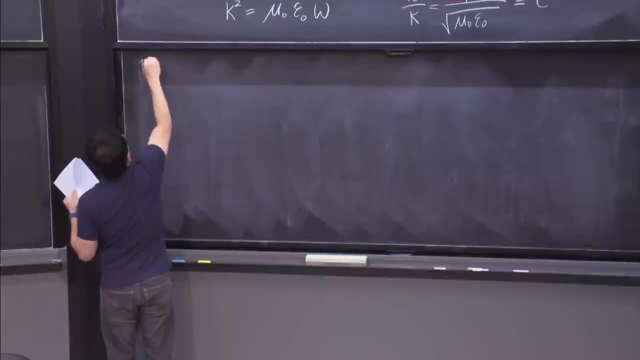 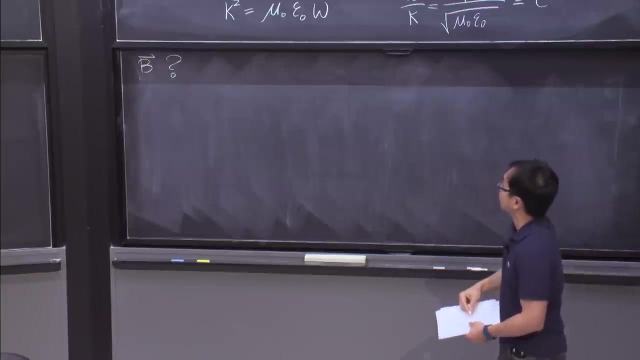 And electric field cannot live without magnetic field, Right? So what is actually the responding magnetic field? We can actually evaluate that, Right? So now the question is: what is actually the magnetic field, And how does that vary as a function of time? 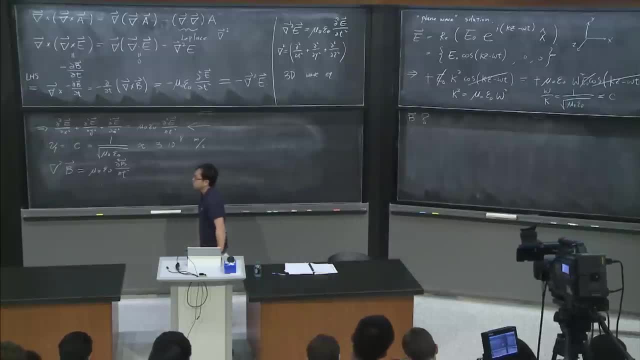 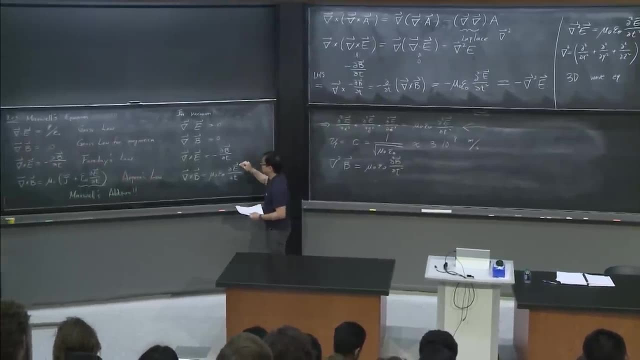 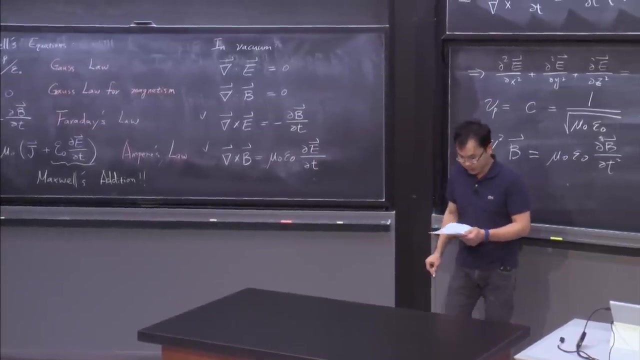 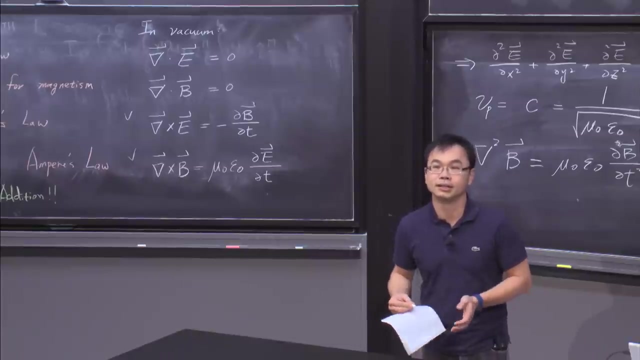 or as a function of position in the space. OK, So we are facing a choice. OK, So there are two equations which relate electric field and the magnetic field, Right? OK, It is actually very important you make the right choice when you start your calculation. 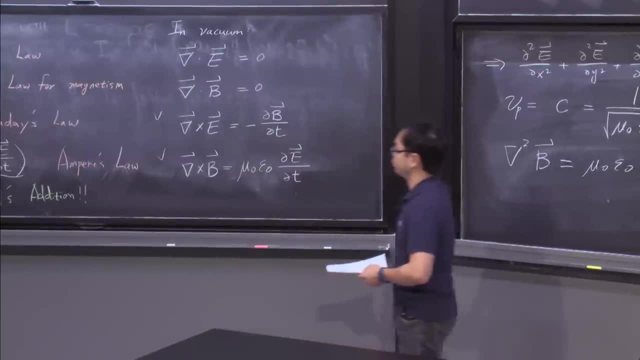 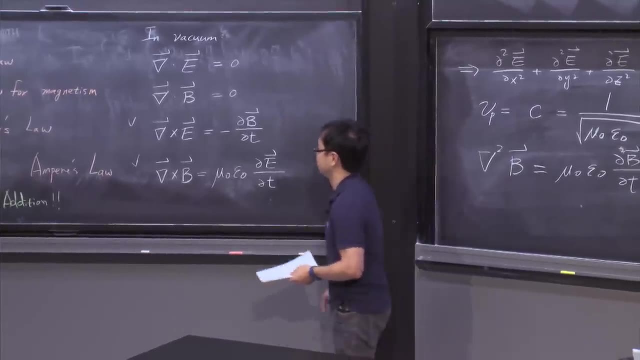 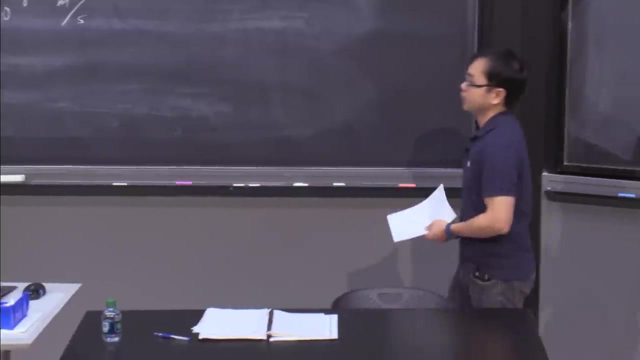 Right, So we can use Faraday's law And we can also use Ampere's law, But there's only one, which is actually much easier to derive the solution, which is the choice of Faraday's law. OK, If you choose to use Ampere's law to evaluate B. 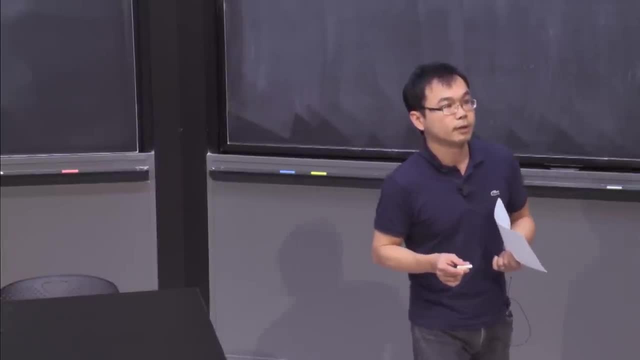 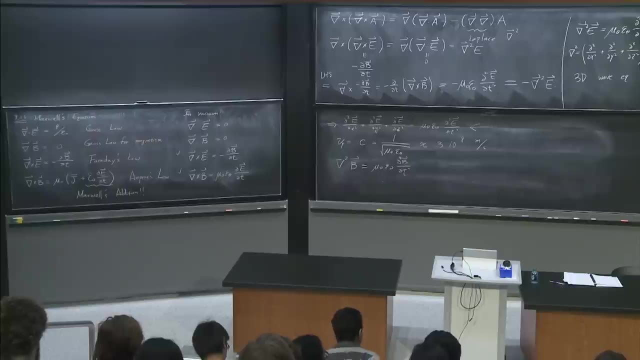 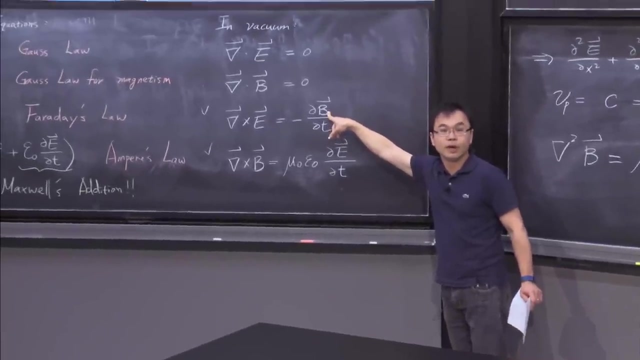 then you are going to get a really super complicated problem to solve. OK, But on the other hand, if you choose to use Faraday's law to solve this problem, then you can actually evaluate the unknown. The unknown is the magnetic field. 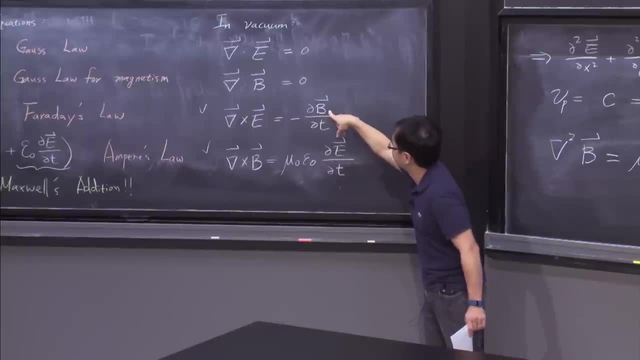 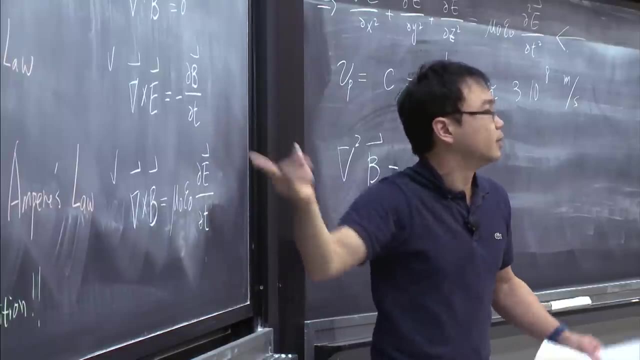 the field which I would like to evaluate Right, And the expression for the B is actually rather simple. It's actually just a partial derivative: partial B, partial T, Right, So it's pretty simple And you can actually evaluate the known part. 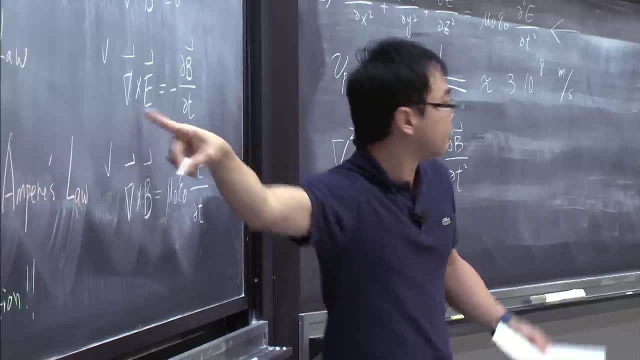 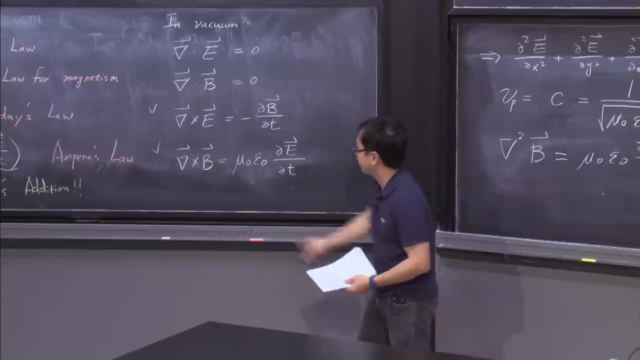 This curl looks pretty complicated, Right, So you can actually evaluate that. because you know what is the electric field, OK, And if you use Ampere's law, then you will be in trouble. Right, Because you don't know what is B X, B Y and B Z. 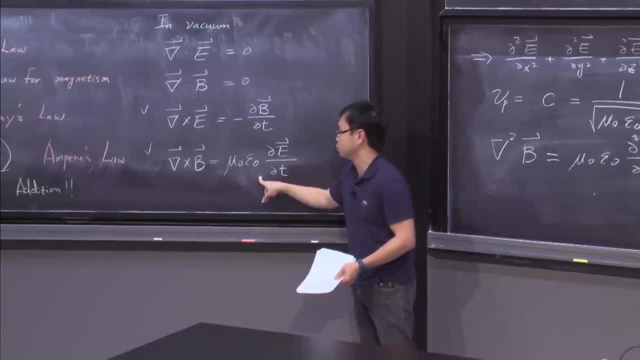 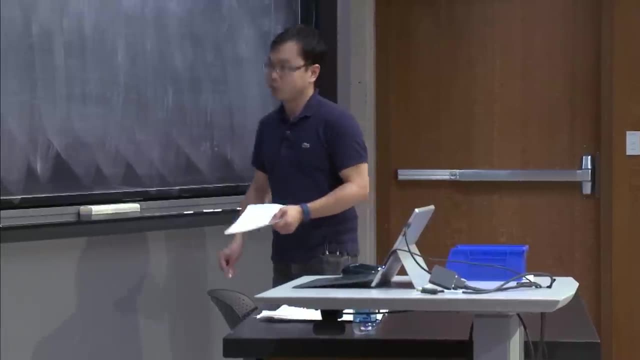 And you have to evaluate curl And you get a lot of terms And that is actually equal to something from the information, from the electric field, And that would be very difficult to evaluate. OK, So therefore, what we are going to do is to use Faraday's law. 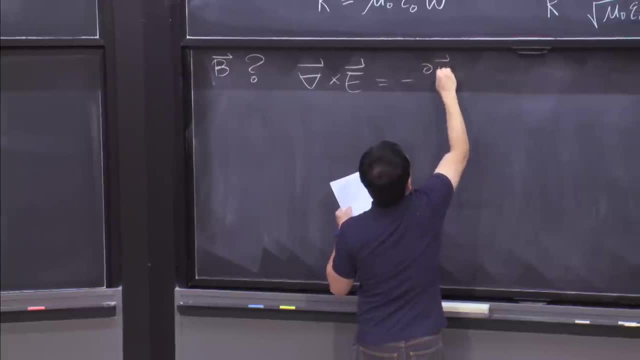 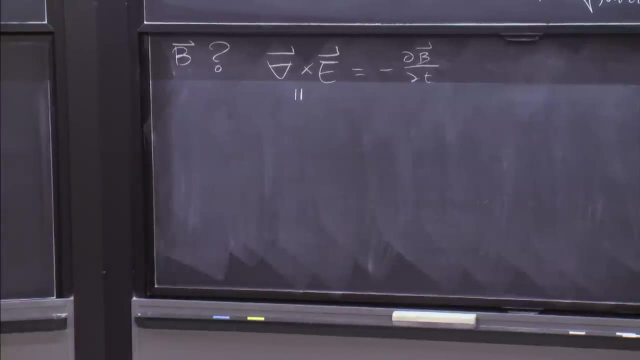 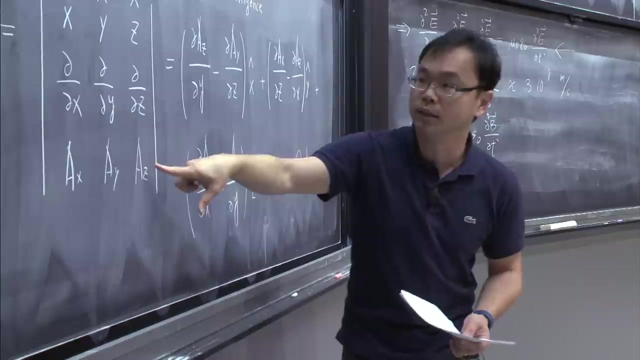 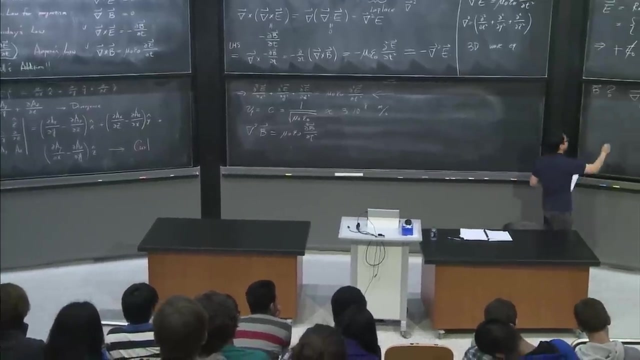 Curl B. This is equal to minus partial B, partial T Right. So basically, as I mentioned in the beginning, we can make use of the equations, the determinant of metrics, to evaluate the curl Right. So therefore, I am going to use that. 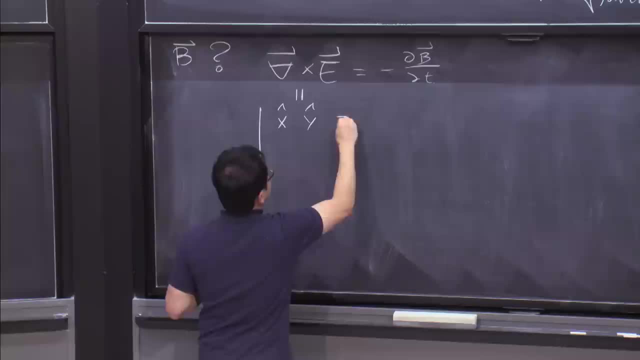 And what I am going to get is X, Y, Z univactor- This is the first row- And partial X, partial partial Y, partial partial Z, which fill the second row of the metrics. Then I get E, X, 0, 0.. 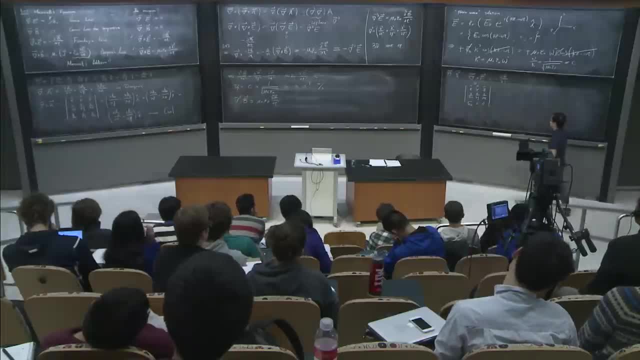 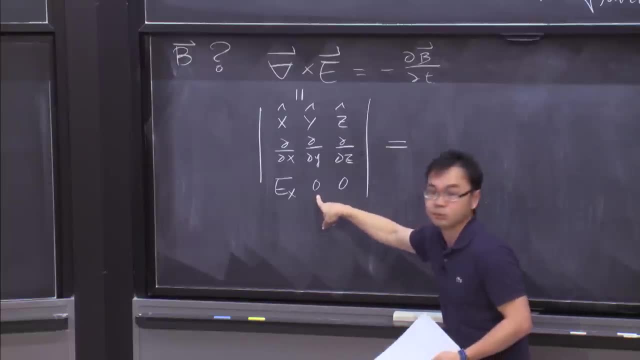 Right, Because the electric field is only in the X direction. OK, And this will be equal to only two terms survive. Right, Because of these two zeros. Right, So a lot of terms are killed. So, basically, two terms are now zero. 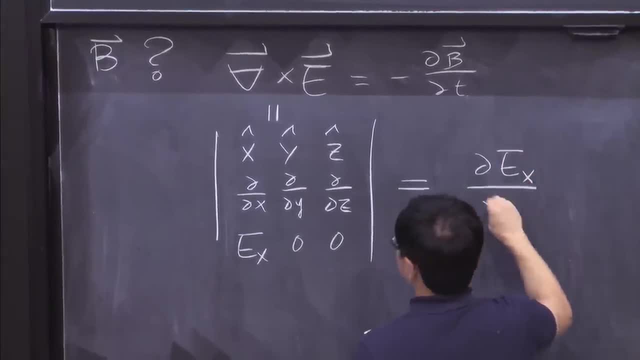 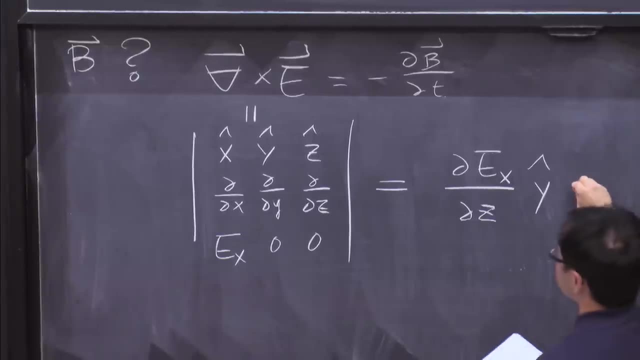 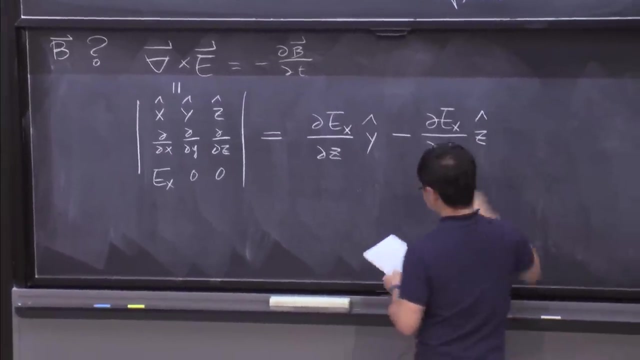 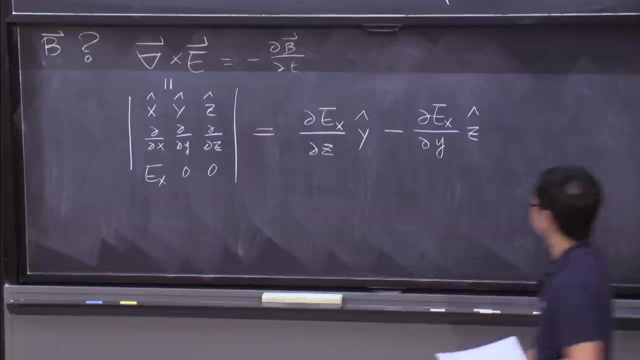 The first term is actually partial E X, partial Z in the Y direction. OK, And the second term is actually minus partial E X, partial Y in the Z direction. Any questions? Am I going too fast, OK? 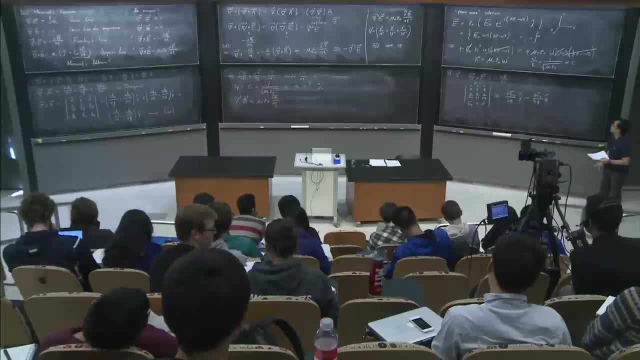 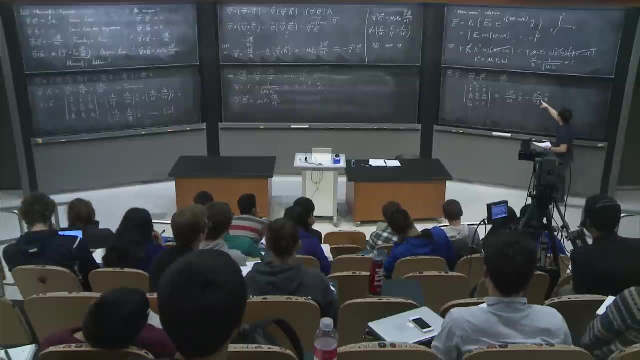 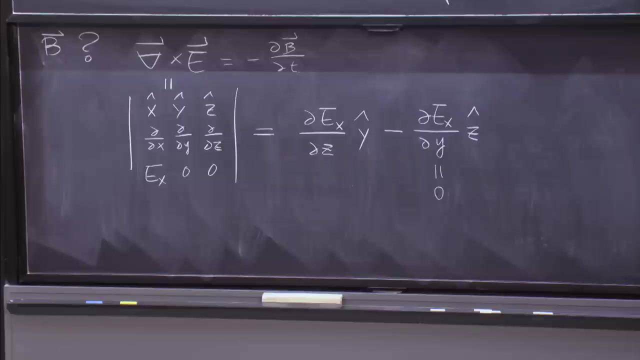 All right, So the electric field only depends on the position Z. It's independent of Y, Right? Therefore, partial E, X, partial Y is actually equal to 0.. Wow, this becomes much, much easier, Right, Because there's only one term, which 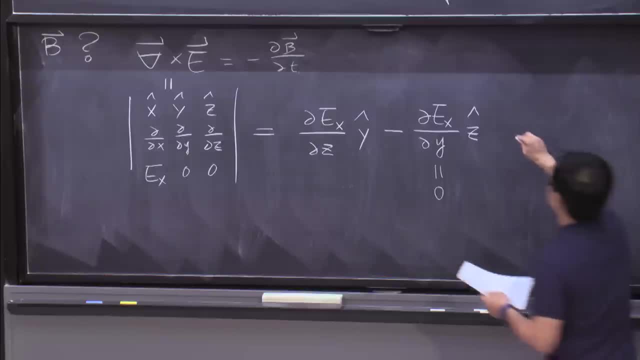 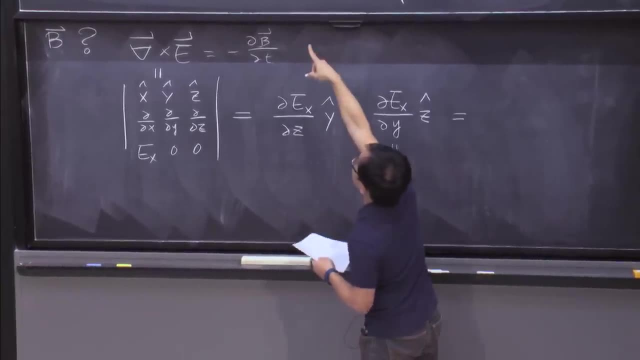 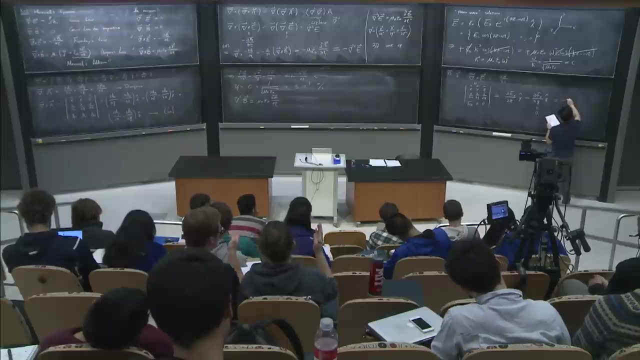 is surviving this operator. OK, And basically what we're going to get is: I can now calculate partial E, X, partial Z Right Based on that equation: E0, cosine kz minus omega t, Then basically what I can get is minus. 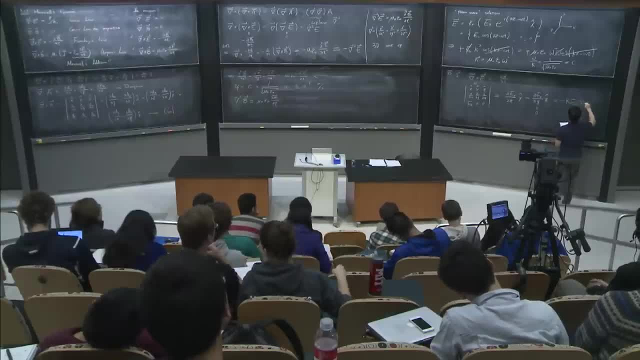 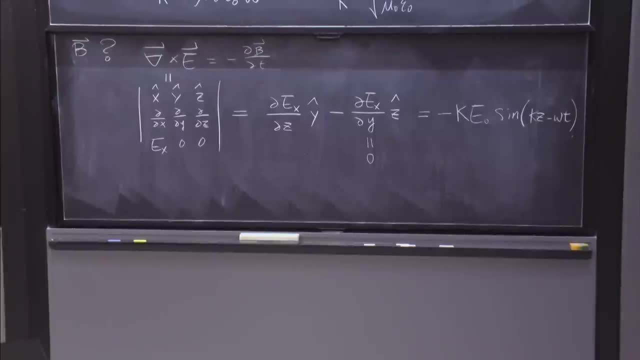 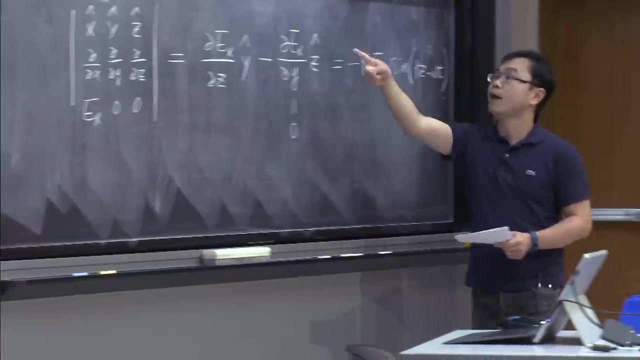 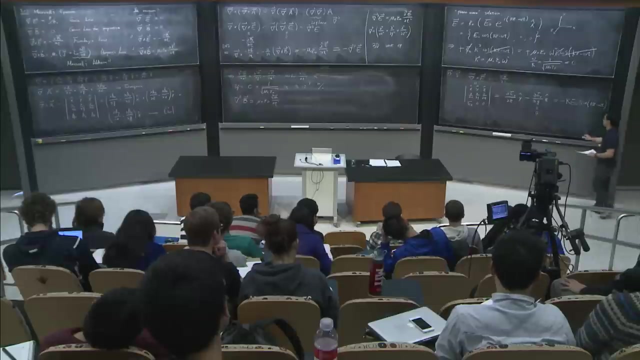 I get a k out of it: E0 sine kz, minus omega t. OK. So this is actually the result of the left-hand side, OK, Of the equation of the Faraday's law is: minus partial B, partial t, Right. 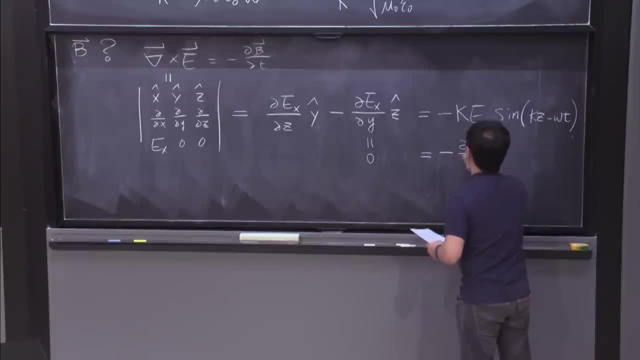 So this will give you equal to minus partial B, partial t, OK And OK. So very important. I don't want to drop the Y direction Right. So this is Y direction, OK, And this is actually a vector, And this is also a vector. 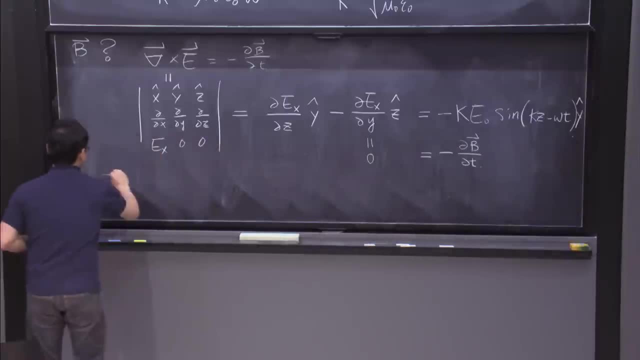 Right. So what I could do is to do integration over t and also cancel the minus sign, Right. So if I integrate over t, then basically what I'm going to get is k over omega E0, cosine kz minus omega t only OK. 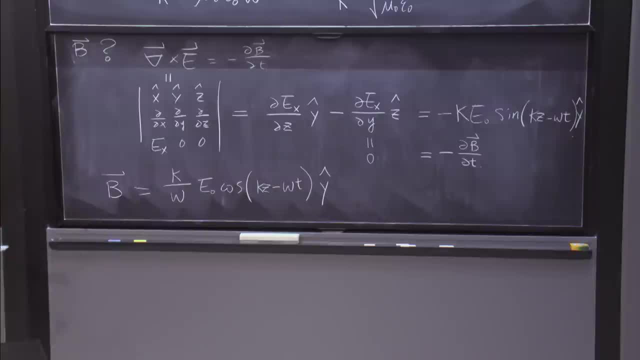 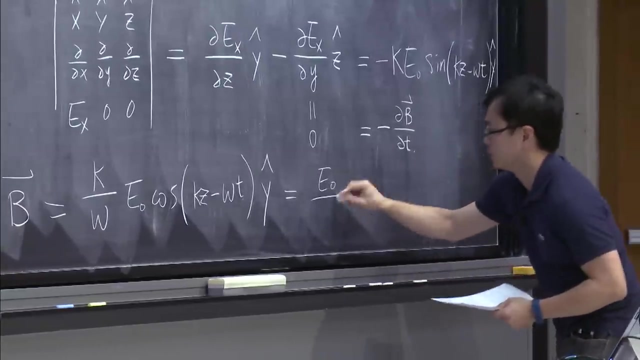 So I'm doing the integration over t. Cancel the minus sign, Then this is what I get. And of course, k over omega is actually 1 over c, Right? So therefore you have E0.. You can actually simplify this expression. 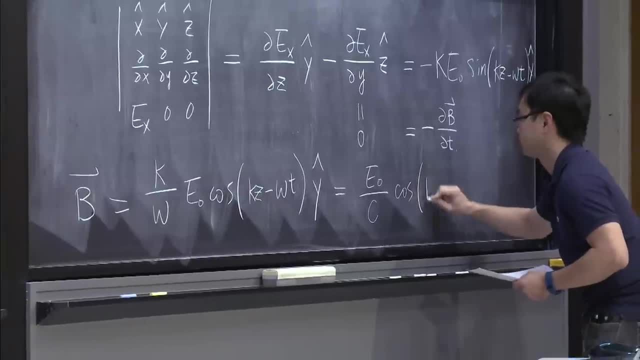 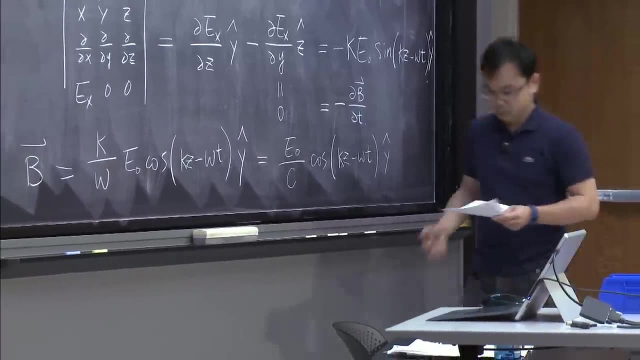 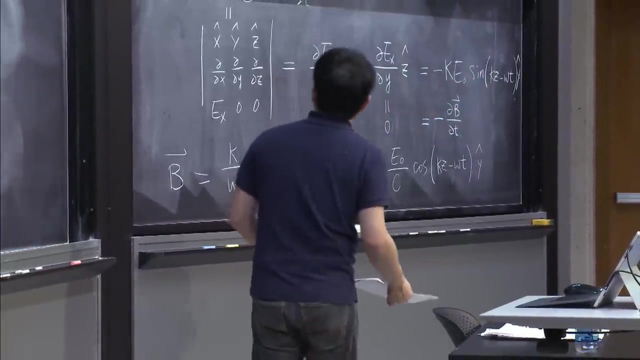 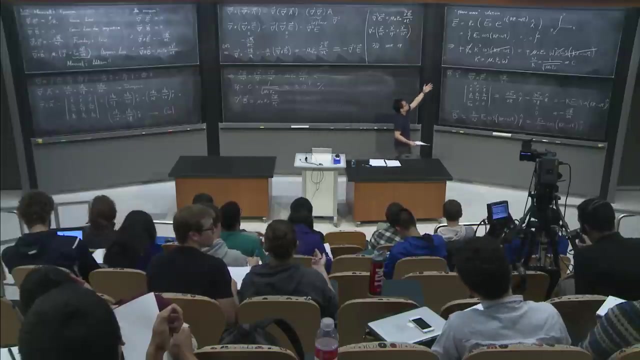 And this is actually equal to E0 over c, cosine kz minus omega t in the Y direction. OK, look at what we have learned from here. OK, What we have learned from here is that? OK, I got started with a plane wave solution of the electric field. 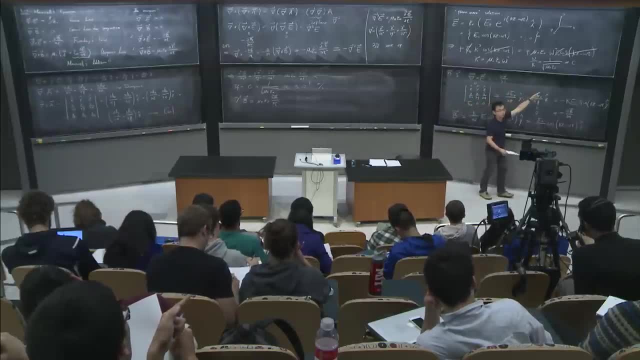 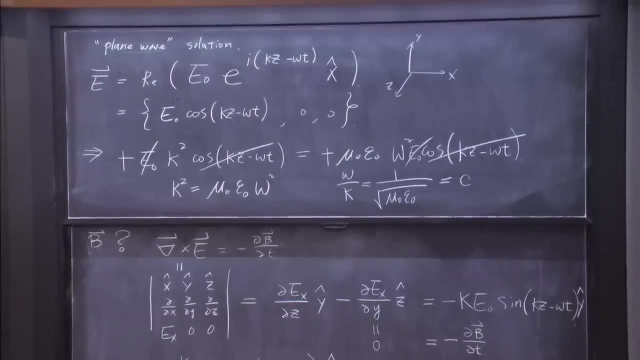 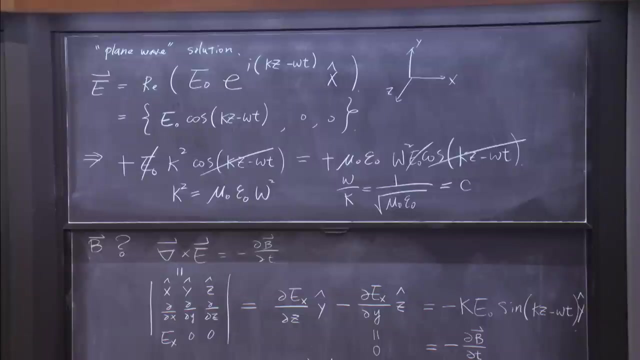 And I can show that only when omega over k is equal to the speed of light. this is actually a solution to my wave equation. OK, And also because the electric field and the magnetic field have to satisfy the Maxwell's equation all the time. 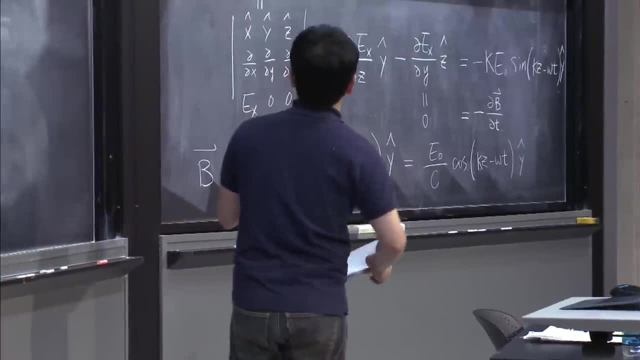 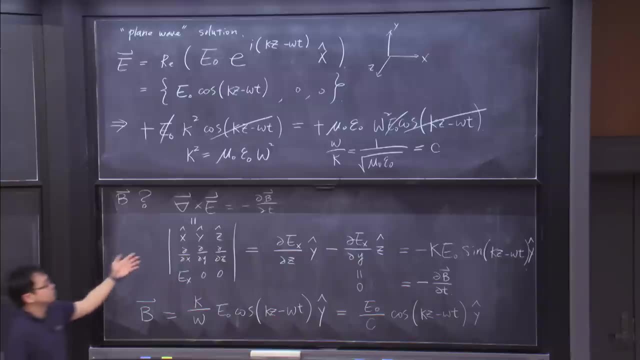 right, because that's the fundamental law. therefore, I can use those equations to evaluate and to find what is actually the corresponding magnetic field And, using Faraday's law and plugging in and solving the equation, I will be able to figure out that B is. 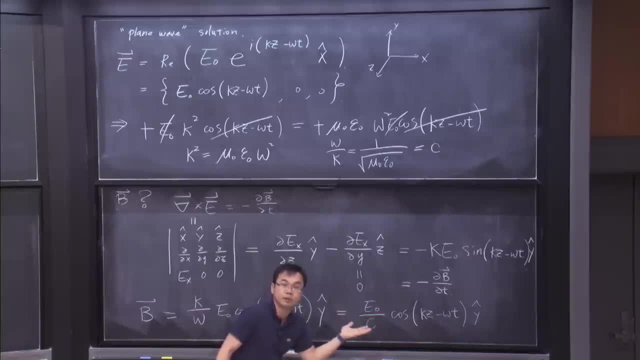 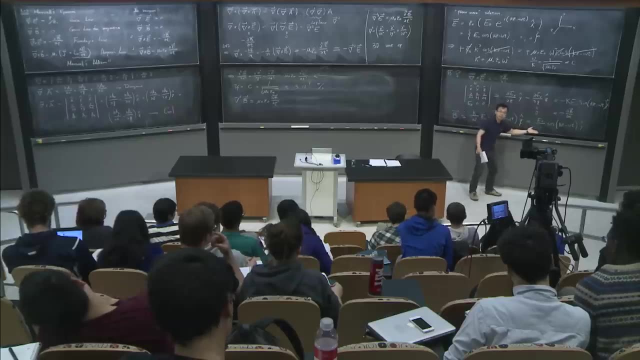 also what kind of wave. B is also what kind of wave I was talking about? Oh, sorry, Plane wave. right, It's also plane wave, You see. So if I got started with a plane wave in the electric field side, 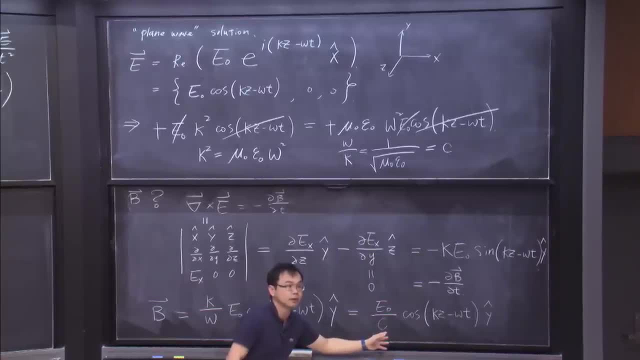 then I also get the plane wave in the magnetic field side. OK, They are proportional to each other. Originally the magnitude of the electric field is E0. The corresponding magnetic field, the magnitude, is proportional to E0. But there is a factor of 1 over C difference. 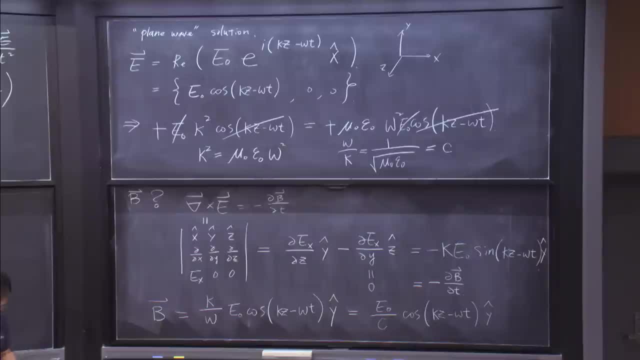 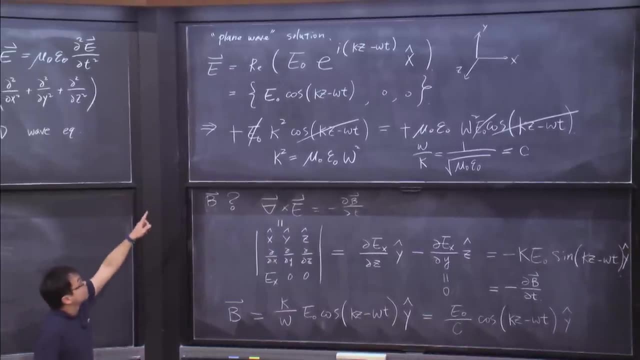 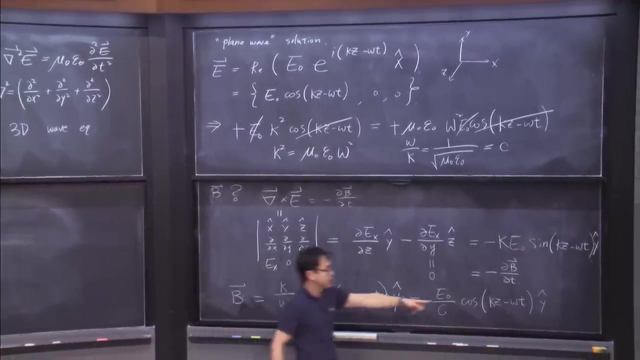 between the magnetic field amplitude and the electric field amplitude. OK, The third thing which we learn from here is that, OK, electric field is actually in the x direction. B field is actually not in the x direction, It's in the y direction. 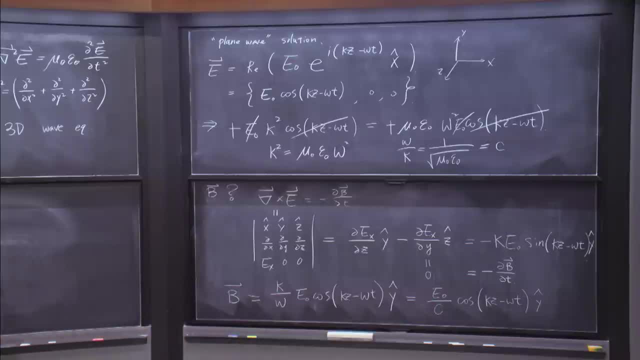 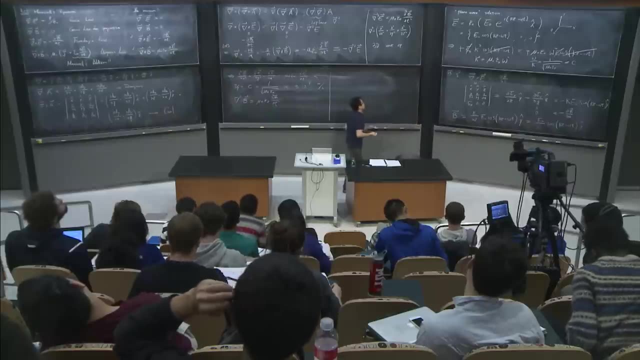 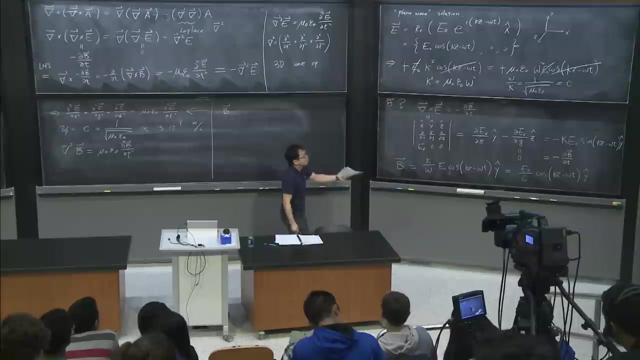 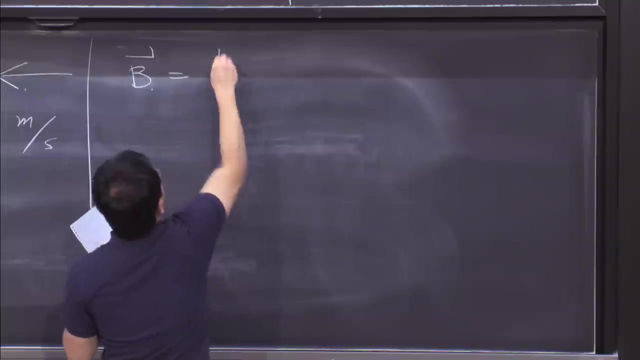 OK, So actually what we learn from here is that the direction of the B field can be determined by a simple calculation. So basically, the B is proportional. The magnitude of B is proportional to the electric field, So it's 1 over L. 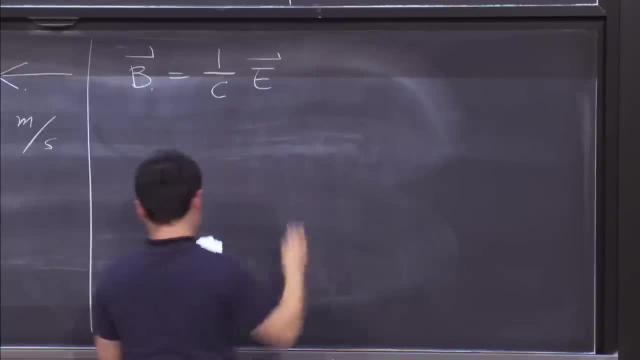 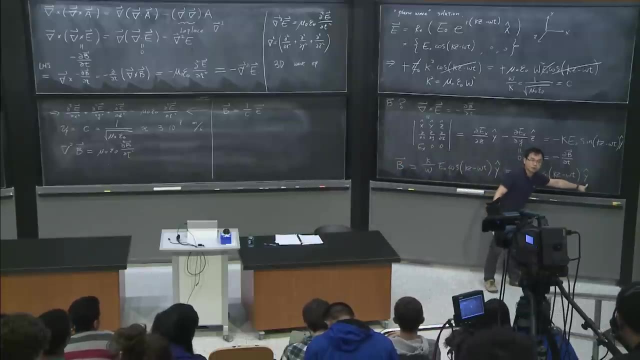 But you have to multiply the magnitude by 1 over C, And also this is actually not correct because the B is actually in the y direction, Right? So the original direction of the electric field is in the x direction. Also, we know the direction of the propagation. 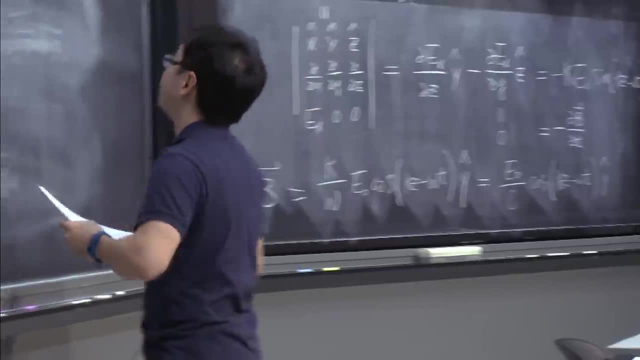 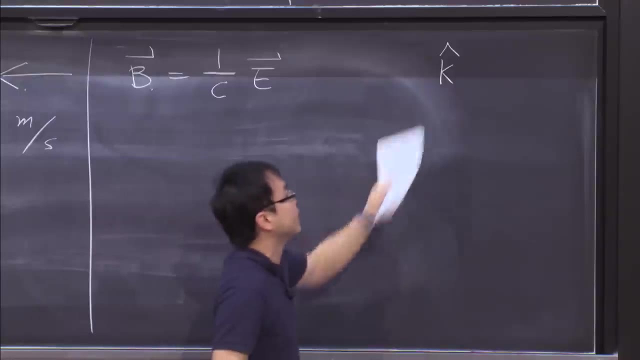 is in the z direction. OK. Therefore, if I take univector k, OK, k is actually the web number, But now I make it a vector And I take the univector is equal to z, the direction of propagation. 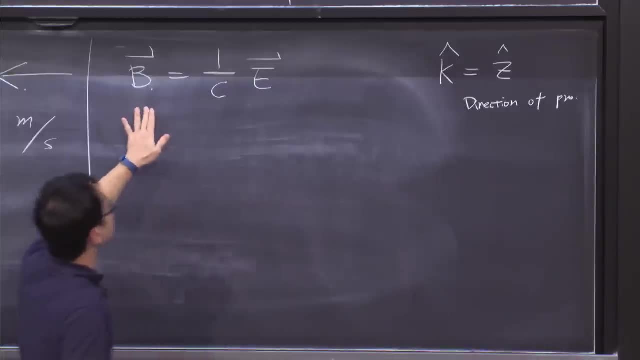 OK, If I make this definition, then I can now rewrite this relation Basically. I can express the magnitude of B by k hat, which is the direction of propagation. cross the E field. OK, And we can check this And basically what you are going to get is z cross E. 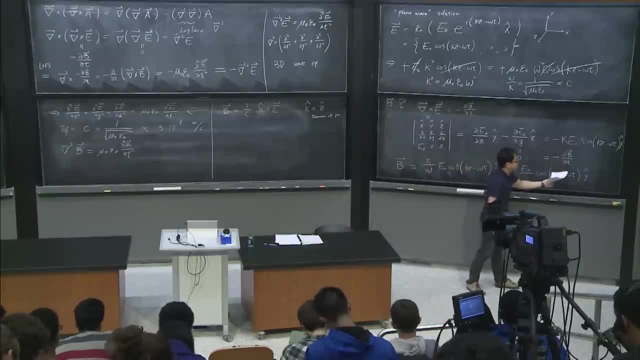 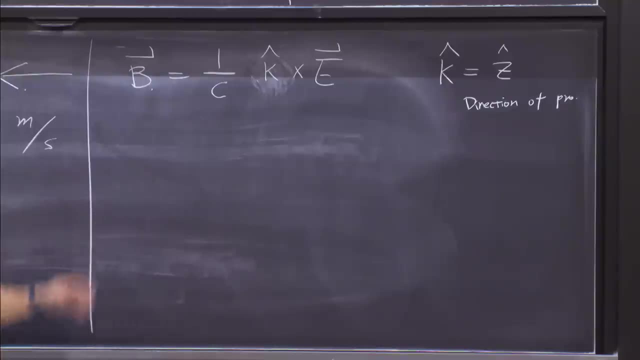 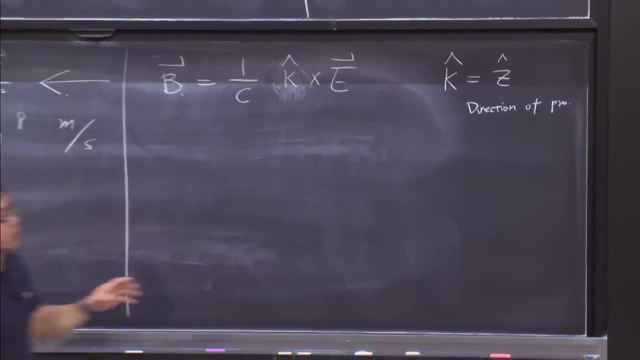 Then actually really z cross x, you are going to get y direction, OK, And that is actually telling you that B and the E have a rather simple relation, And also you don't really need to go through all those calculations again. 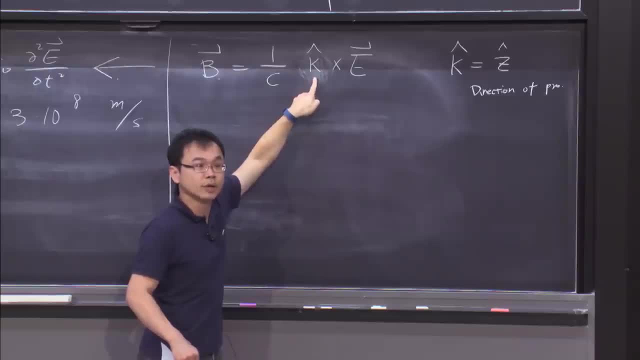 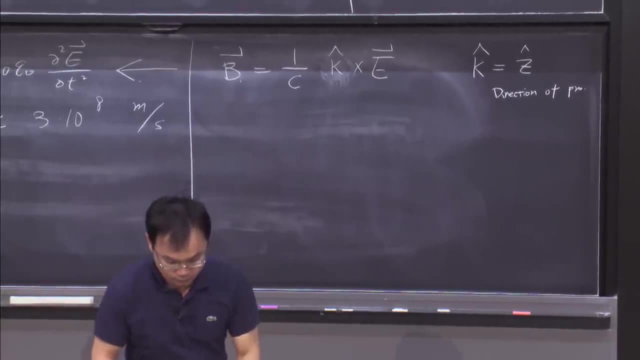 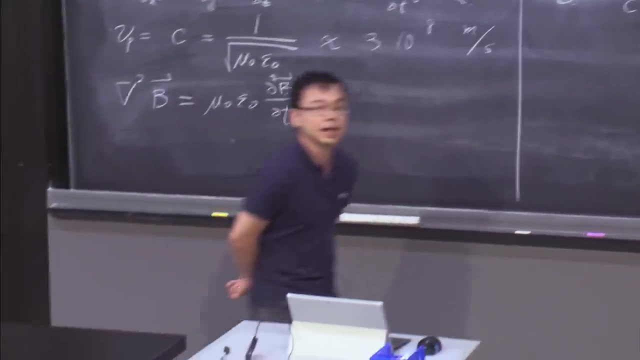 Because now you can see that if you know the direction of propagation and you know the direction of the electric field, then you can already evaluate what will be in the B field. OK, OK, so we will take a minute break. We'll come back in 29.. 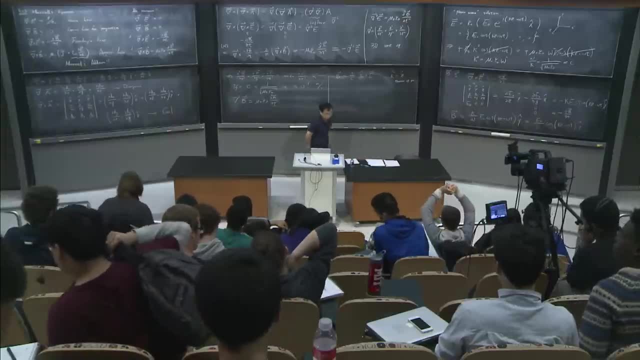 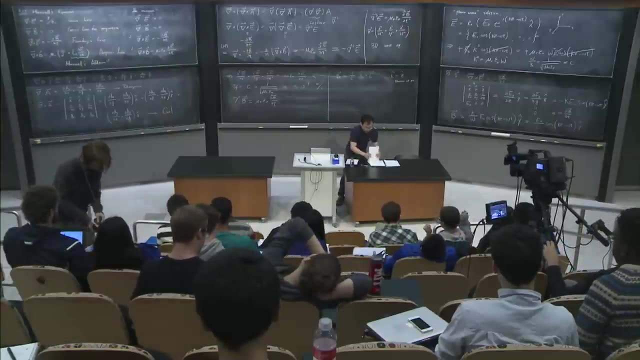 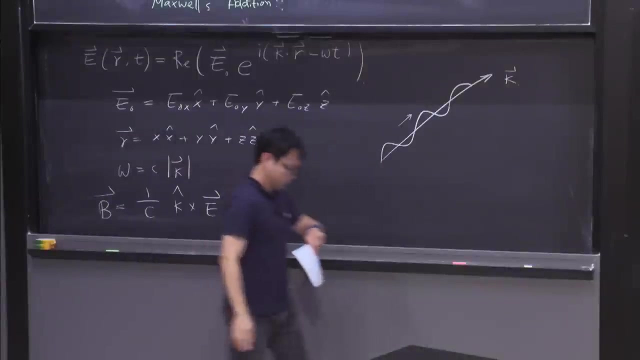 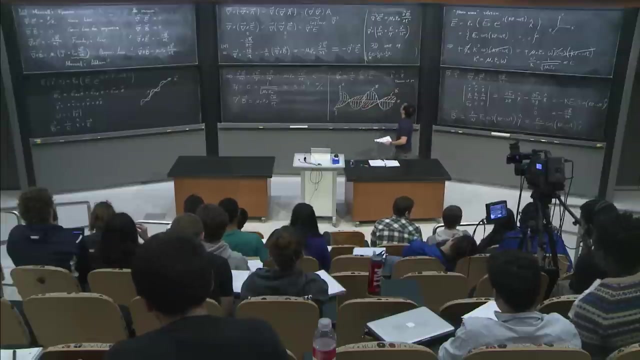 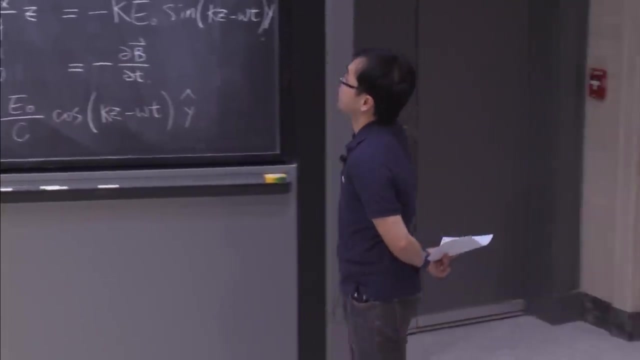 And we will continue the discussion about this solution. Let me know if you have any questions about the content we discussed. OK, we'll come back everybody. So we will continue the discussion of what we have learned on the wave equation. So basically, we start with the plane wave in the electric field. 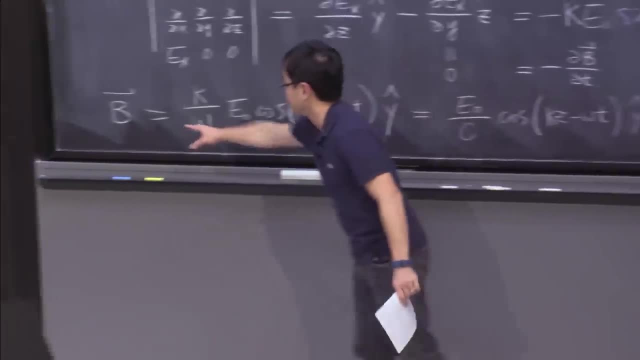 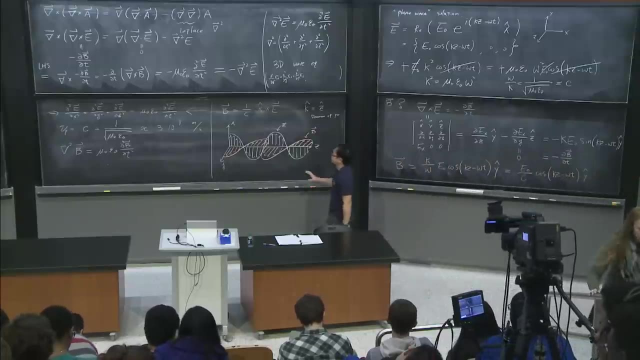 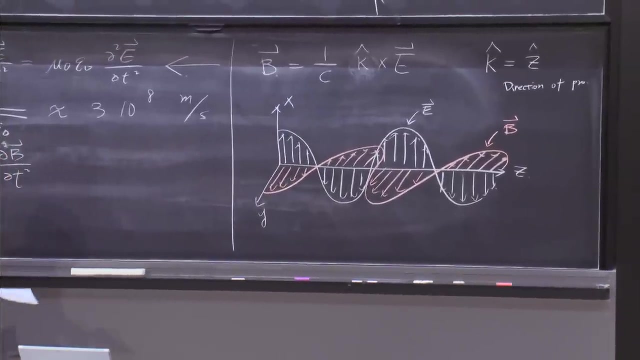 And the electric field is in the x direction, And we evaluated the corresponding B field, which is in the y direction, Right, And what we found is that actually we can find a pretty simple relation between electric field and the magnetic field, which is actually a magnetic field. 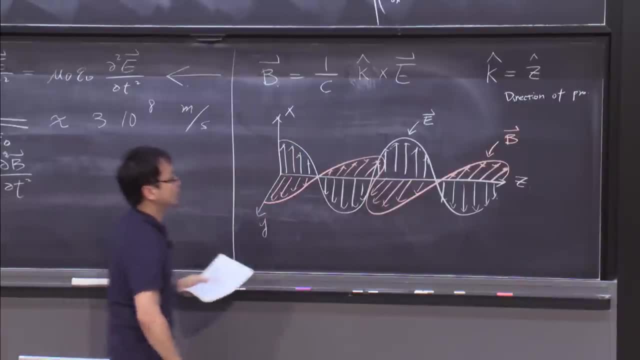 vector is equal to 1 over c, k hat cross E And the k hat now which is defined here is actually the direction of propagation. So basically, in this case, in the discussion we had before, the direction of propagation. 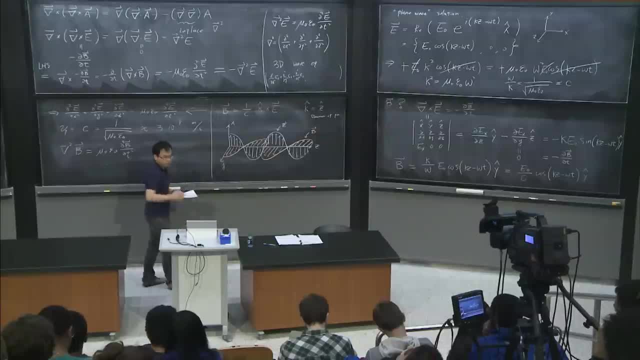 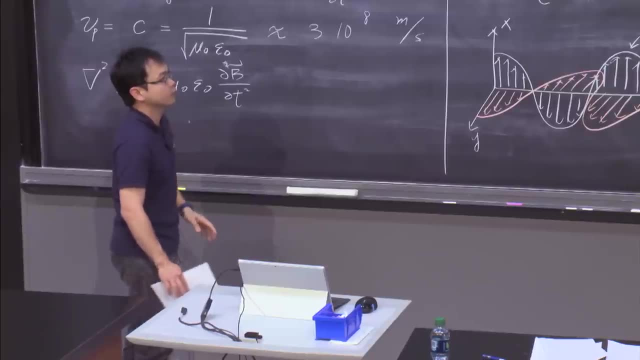 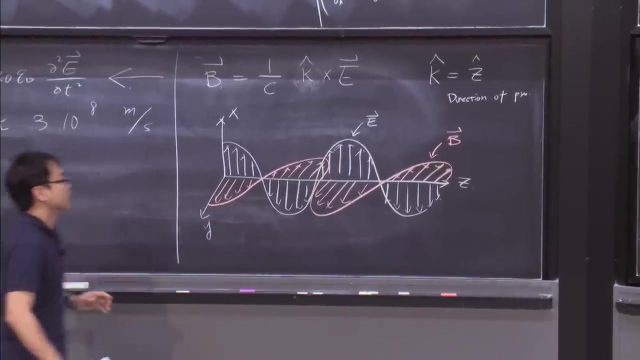 is in the positive z direction. OK, So if I go ahead and visualize the whole solution plot the magnetic field and the electric field as a function of z, x and the y as a function of z, actually here, and I only evaluate the value, 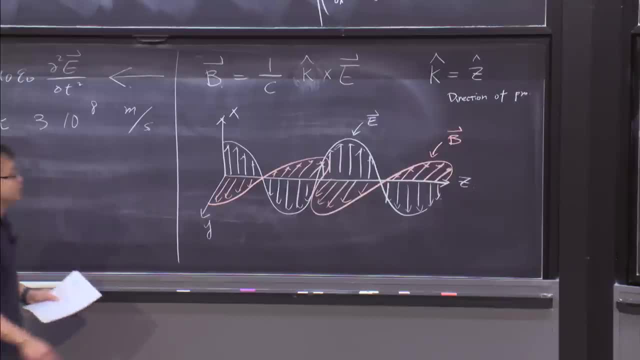 by looking at x equal to 0 and y equal to 0. And basically, this is actually what you have. So basically, you have two sine wave. One is actually pointing to the x direction And the other one is actually pointing to the y direction, which is the B field. 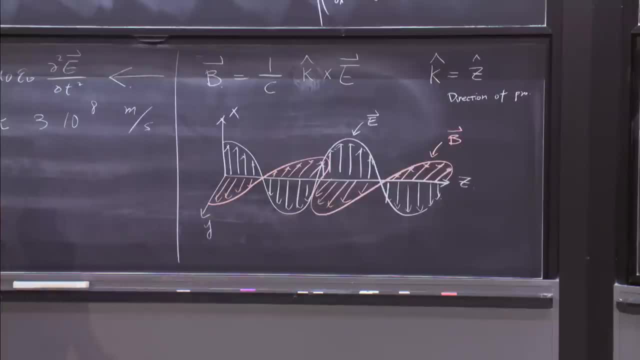 OK, And those lines doesn't mean a lot because those are actually just connecting the endpoint of all those vectors, Right? So you can see that there are sine wave structure or cosine wave structure when you connect all those vectors And keep in mind that those are evaluated at x and y equal. 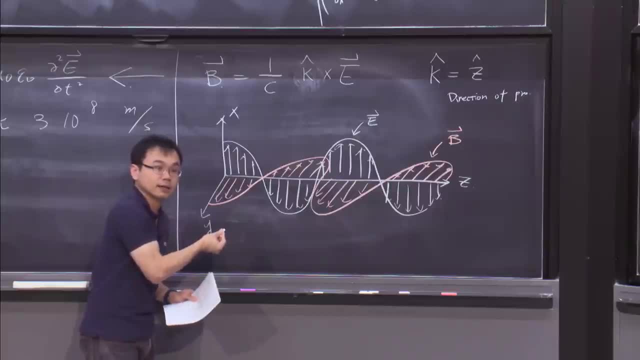 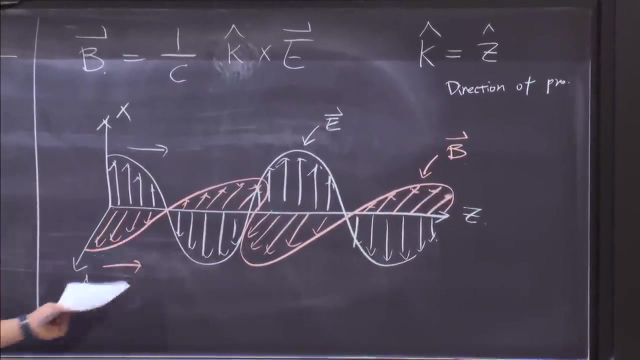 to 0.. Therefore, what we actually get is actually a lot of vectors. OK, So those individual arrows are vectors And this whole thing, this whole electromagnetic wave, is propagating to the positive z direction. So the magnetic field and the magnetic field. 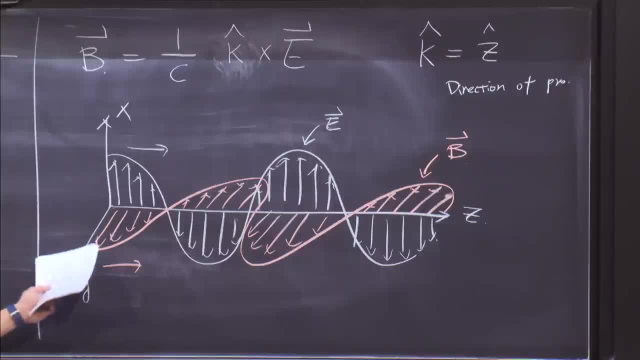 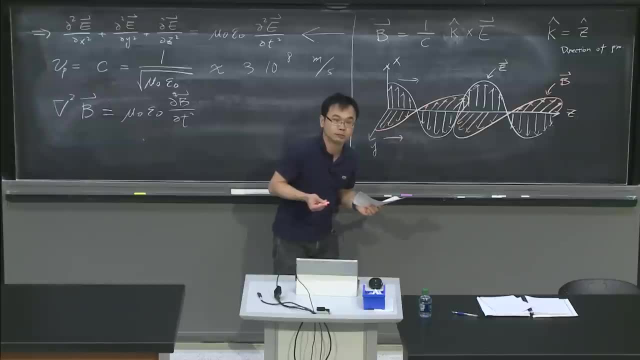 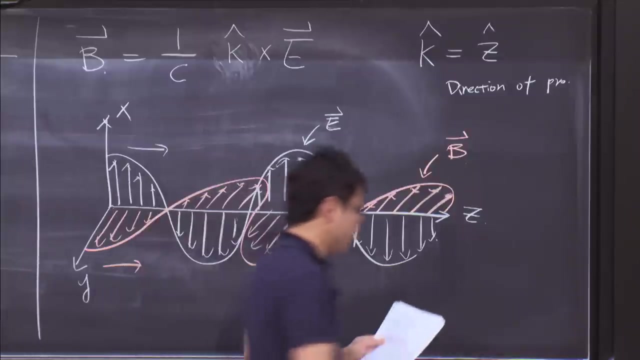 are propagating at the speed of light which you see, And also you can see that the magnitude, as I probably hear the magnitude. there is no phase difference between electric field and magnetic field. OK, This is actually not always the case. 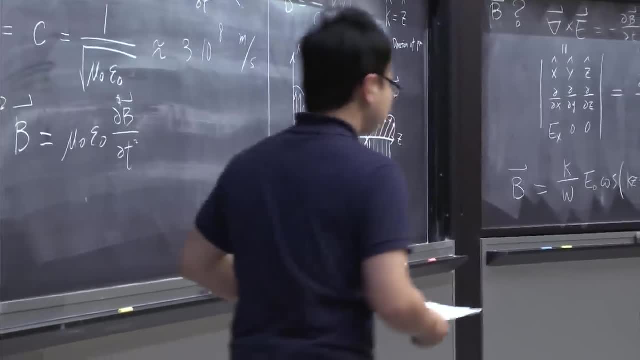 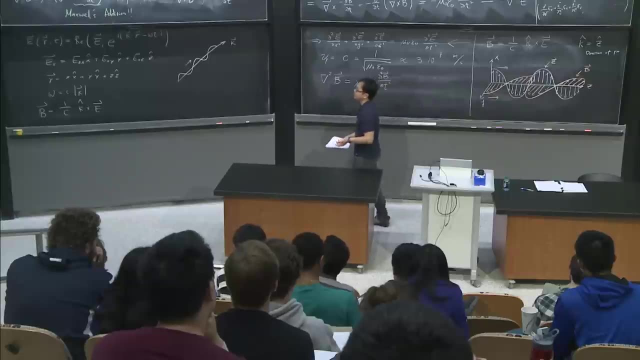 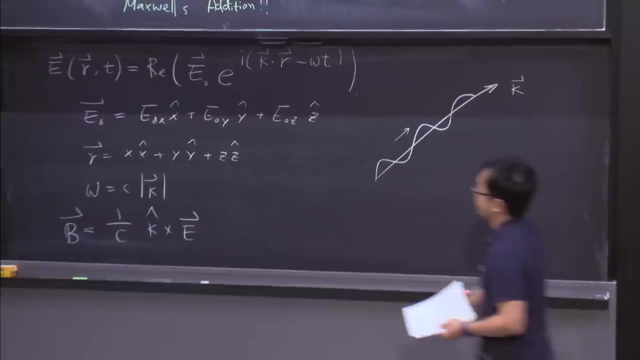 and which we will show an example, probably later in the lecture. OK, So in general, what we can actually do is to write down a general expression for the plane wave. So, for example, I can have a plane wave which is actually propagating in some direction, which is actually 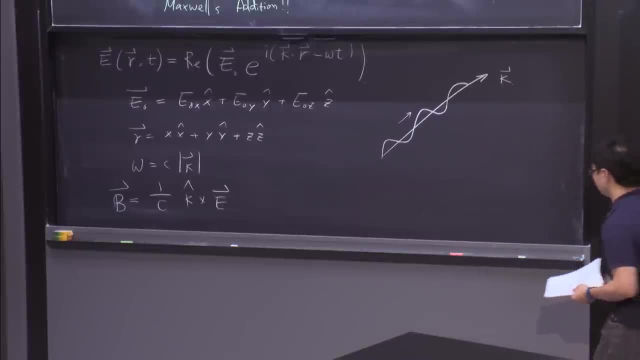 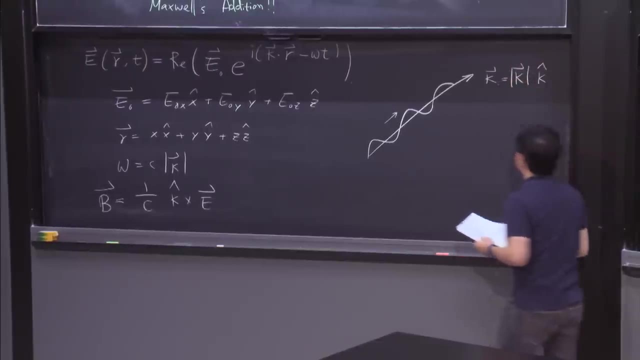 given by this k vector. OK, The k vector is actually giving you information about the wave number, And the k vector is giving you the direction of propagation. OK, And in this case, what I'm trying to construct is a solution which is actually propagating along. 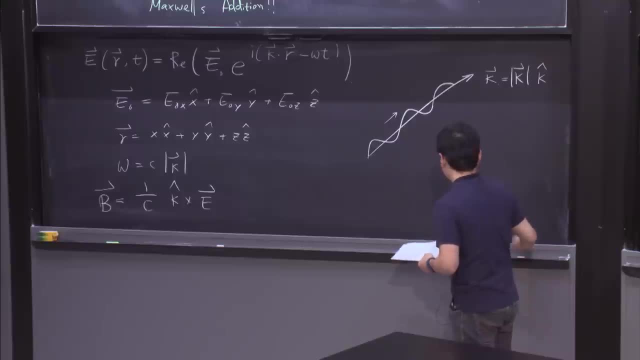 in the direction of the k vector And the electric field is actually going to be pointing to a direction perpendicular to the direction of the k vector. OK, So what I can do is I can write this plane wave in this functional form. E0 is actually a vector, which is actually 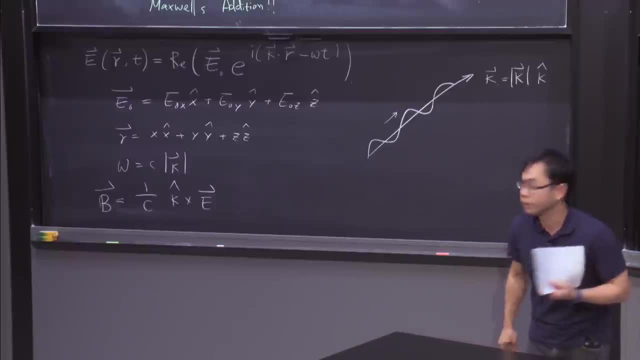 telling you the direction of the electric field. OK, E0 vector is actually have this functional form. OK, And the k vector is actually placed in the exponential function, inside the exponential function. So this is actually i k, dot r minus omega t. 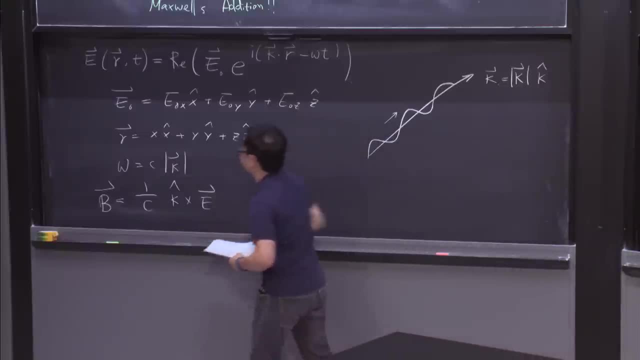 OK. And what is actually r? r is actually xx hat plus yy, hat plus cz hat. OK. And omega is actually the angular frequency which we are familiar with, And this is actually equal to c times the magnitude of k, which is actually the wave number. 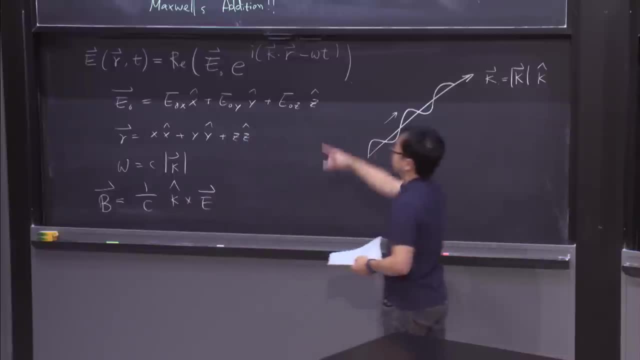 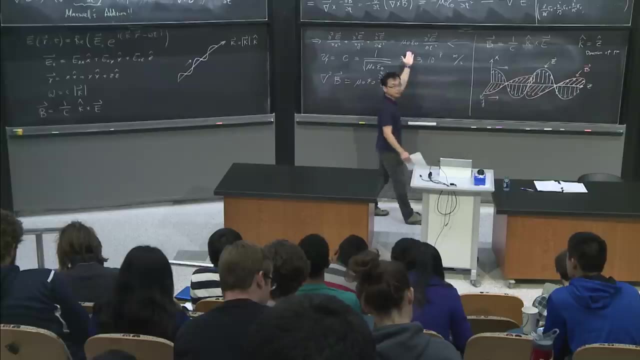 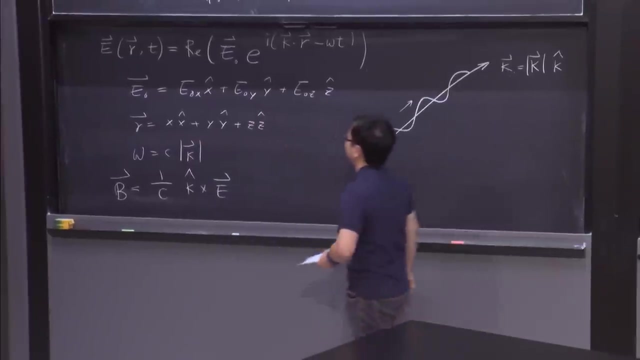 OK, And you can actually show that? OK, indeed, this expression can satisfy the wave equation which we derived for the electric field And of course, there are some requirements, which is actually that the direction of the electric field have to be perpendicular to the direction 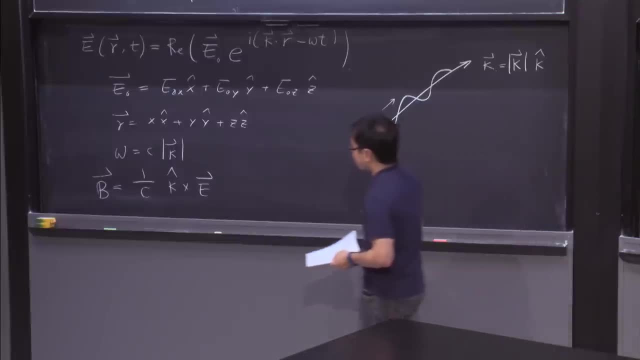 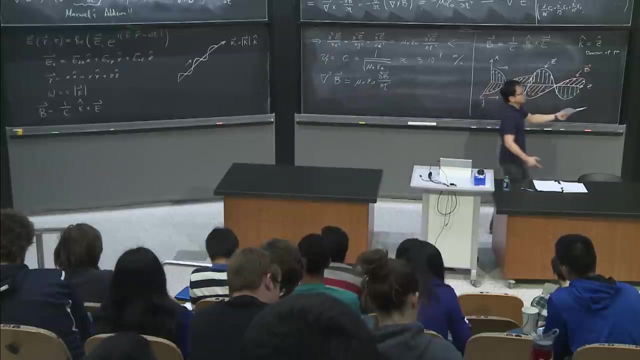 of the electric field, OK, Which you can actually derive that? And finally, this expression, b field equal to 1, over c, k, which is the direction of propagation, cross e field, is still valid because, basically, we have shown that it works for the plane. 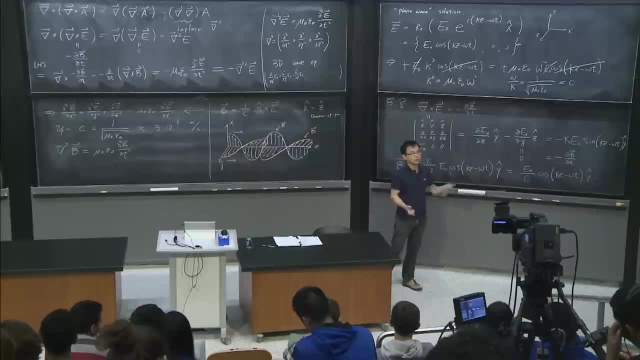 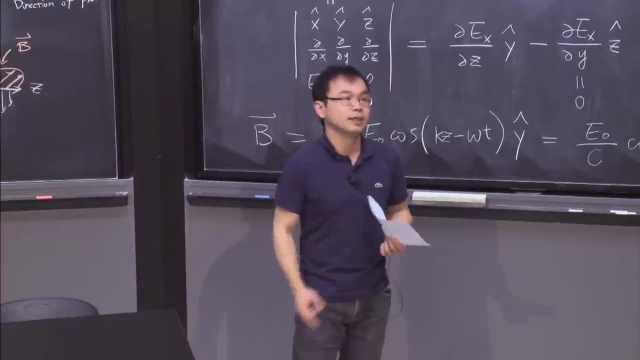 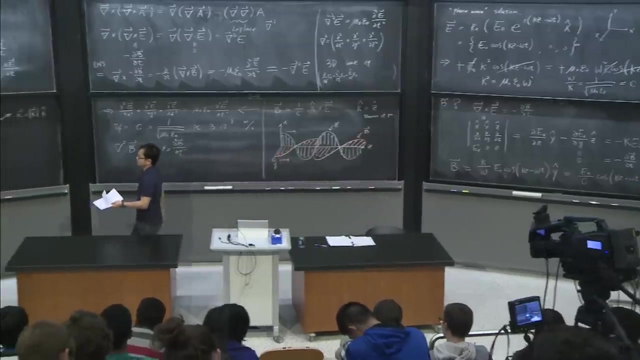 wave pointing to the x direction, propagating to the z direction. We can always redefine a coordinate system right. Basically, we can actually rotate the coordinate system and the physics should not change Right. Therefore, you must see that this expression must. 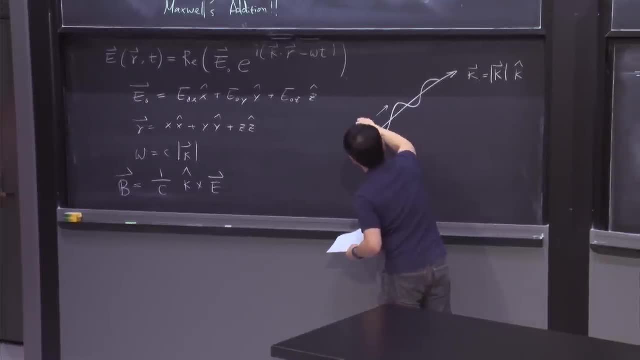 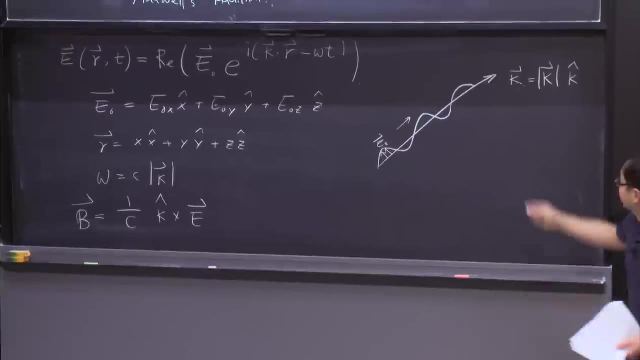 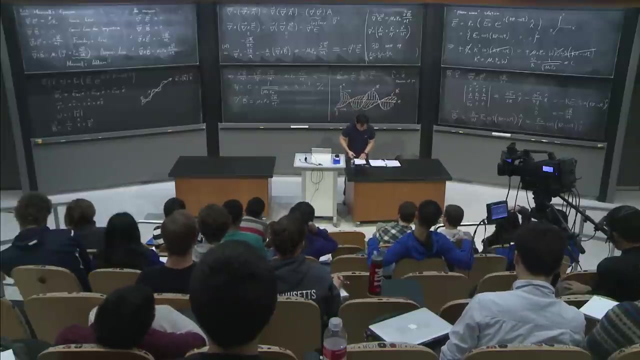 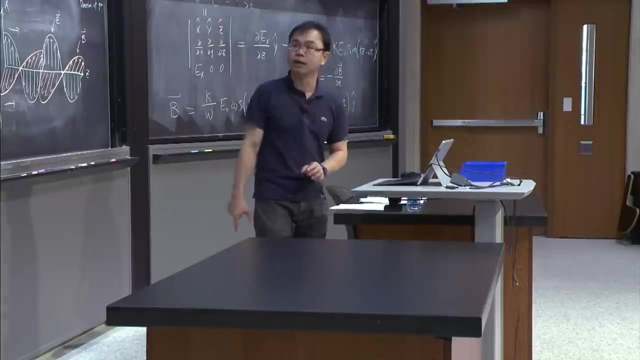 be still valid. And also the direction of the electric field- OK, which is actually proportional to e0, must be perpendicular to the direction of propagation. OK, So that is actually what we can actually derive: a general description of electric field pointing to some random direction. 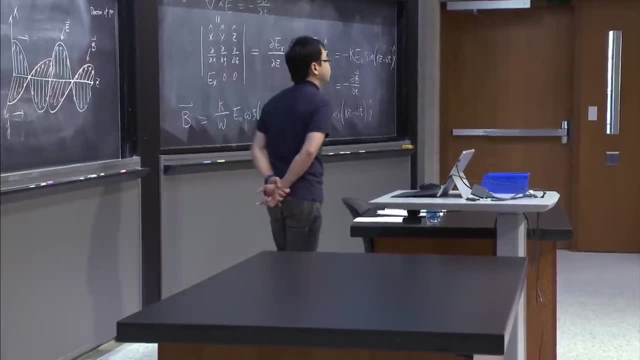 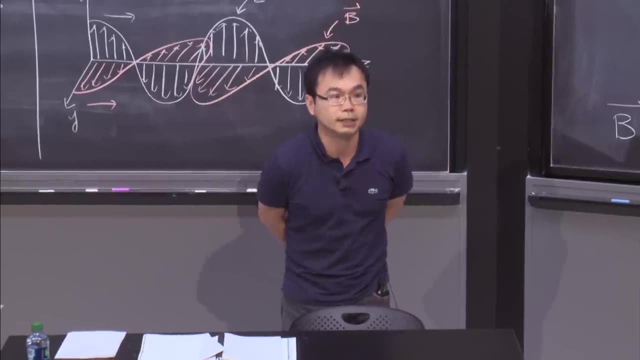 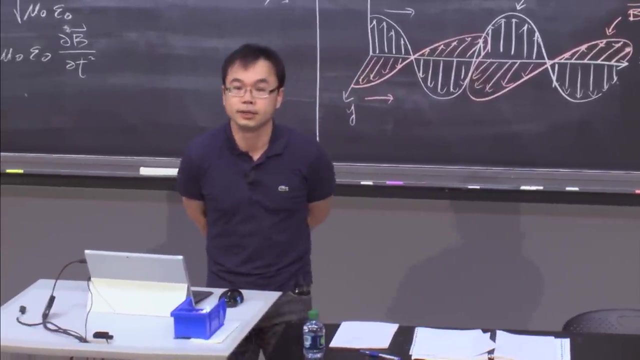 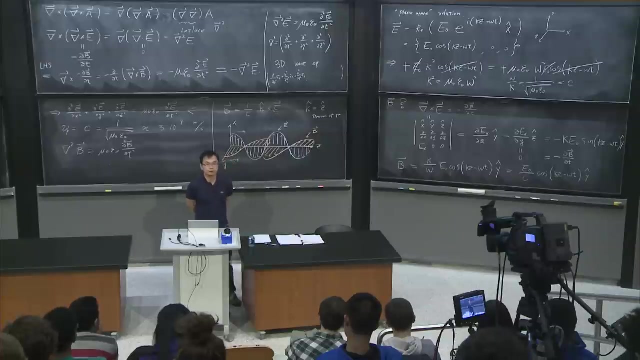 OK, So we have talked about a progressing wave solution and also the plane wave and also the corresponding magnetic field. I hope that you can actually apply this technique which we learned here: If you are given a magnetic field, then there must be a corresponding electric field. 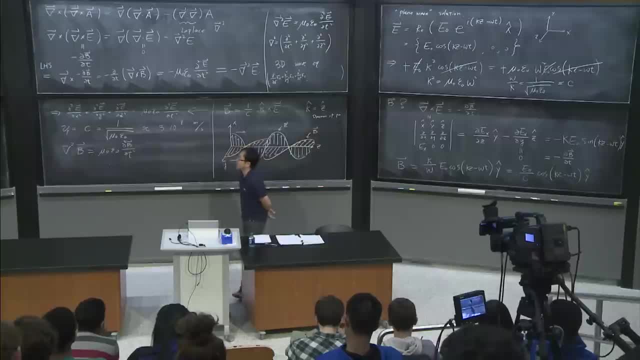 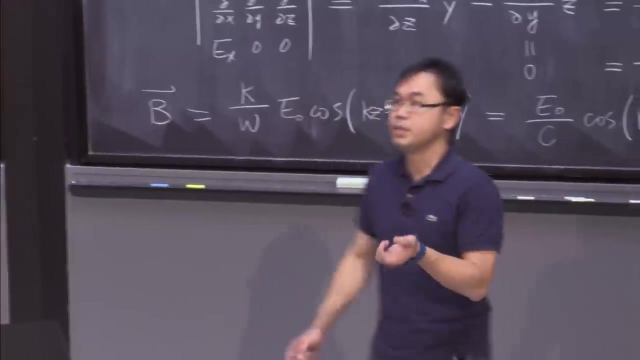 because they cannot be separated from each other And you can actually obtain the corresponding electric field if you are given magnetic field by using Maxwell's equations. OK, So what is going to happen is that now, if I emit this photon, or say this electromagnetic wave, 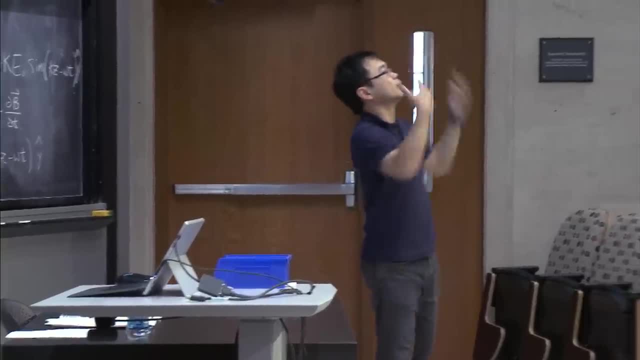 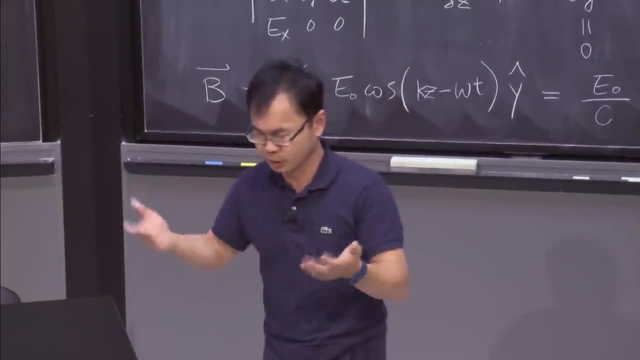 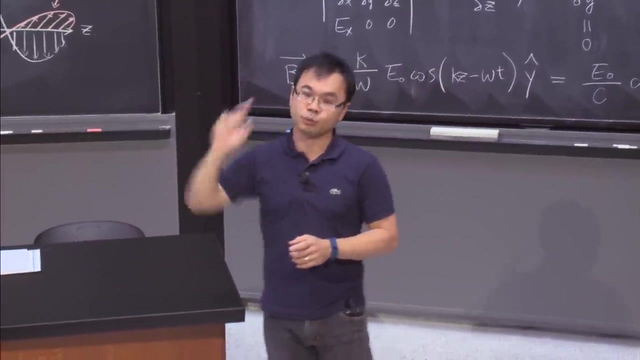 from a light source, for example the one which is pointing at my face. basically, my face is going to bounce some of the electromagnetic field around And some of them actually go out of the window Right. And then, when they go out of the window, 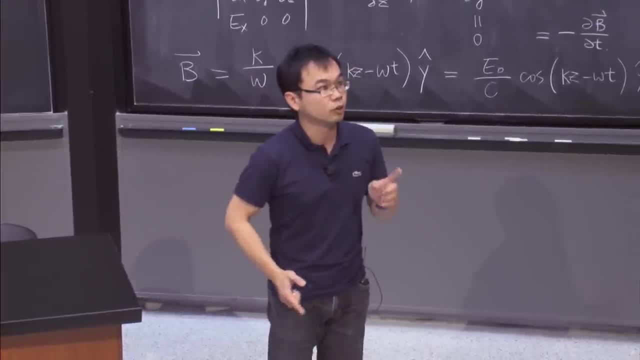 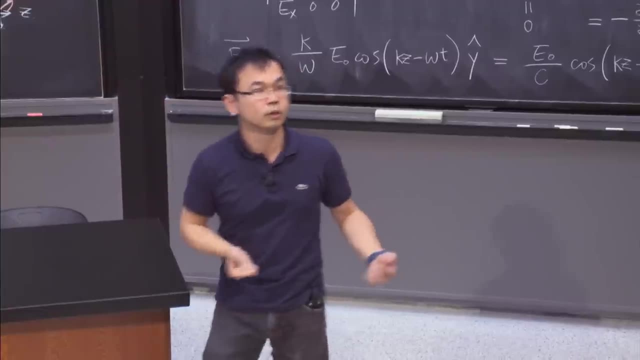 maybe they are lucky they are not hitting any building in the NIT. Then what is going to happen is that they are going to propagate forever toward the end of the universe. Really, they are going straight. They are going to propagate forever, As you can see from this solution. 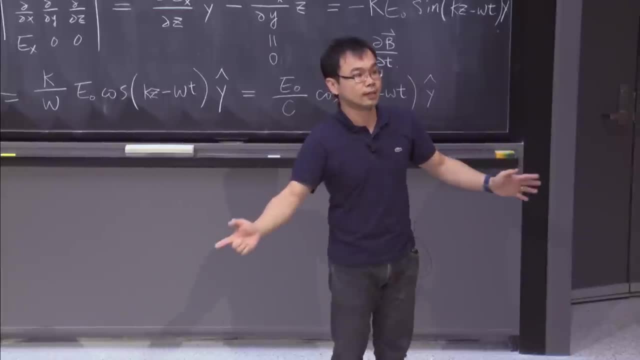 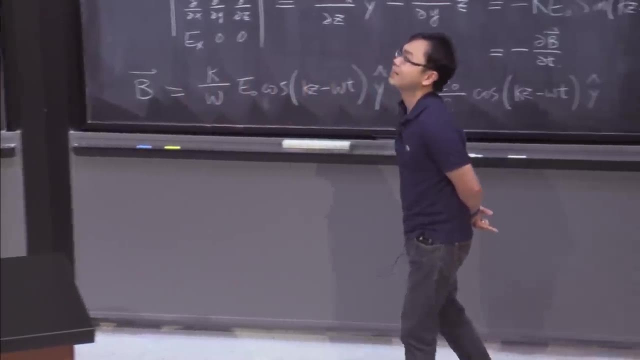 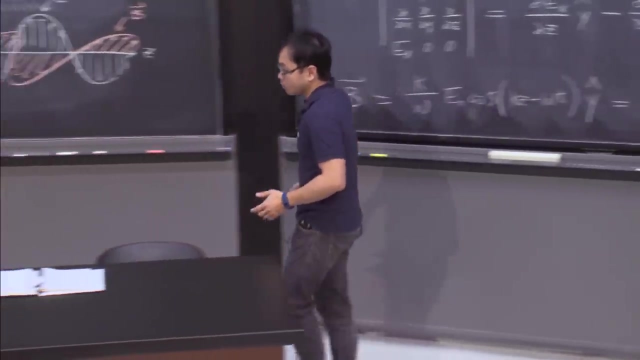 it's like some kind of wave propagating forever at the speed of light. If they don't encounter anything before the end of the life of the electromagnetic wave, it's going to be propagating forever toward that direction. OK, Escaping from the window. 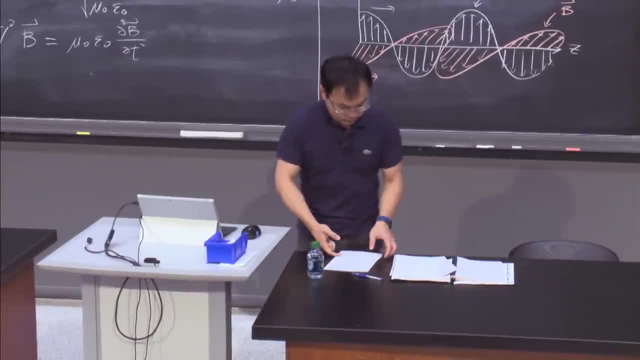 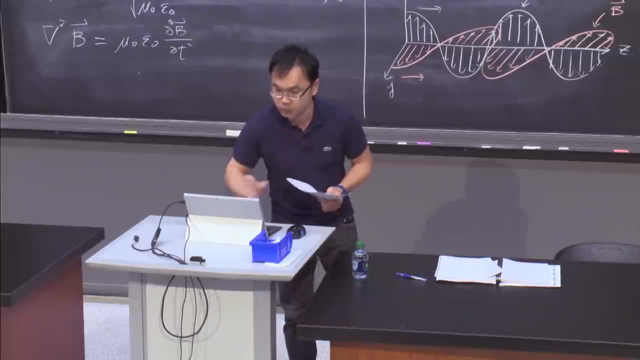 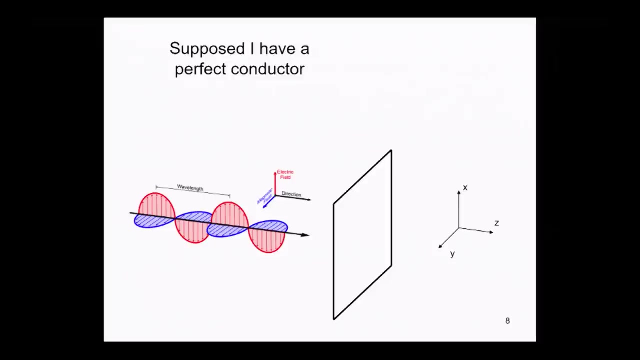 OK, So that is actually fascinating, But we would like to introduce some more excitement and see what is going to happen. So what I am going to do is now, instead of only discussing about the plane wave, what I am going to do is that I would 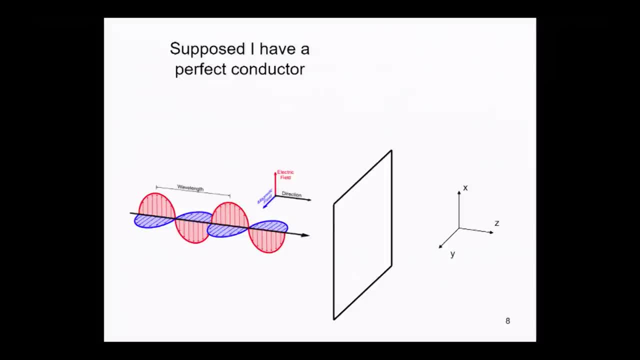 like to add a perfect conductor into the game and see what is going to happen. OK, So what do I mean by a perfect conductor? OK, A perfect conductor can be seen in a musical, in a concert, But the one which I am talking about, 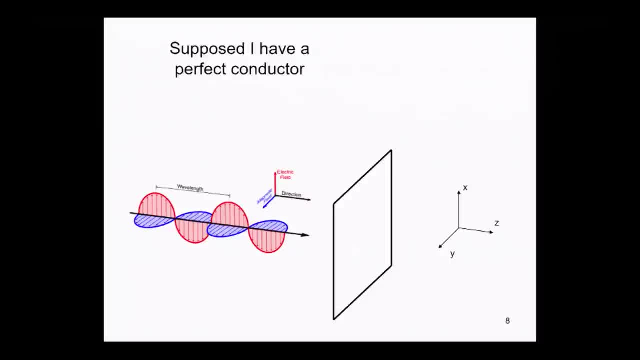 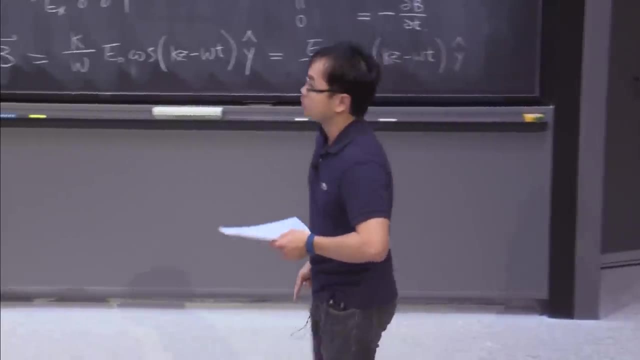 it's not that one, which is also fascinating, But this is a different system. The interesting thing is that both the conductors in the concert and this one is very busy. Right, It's a very busy system. OK, What do I mean by perfect conductor? 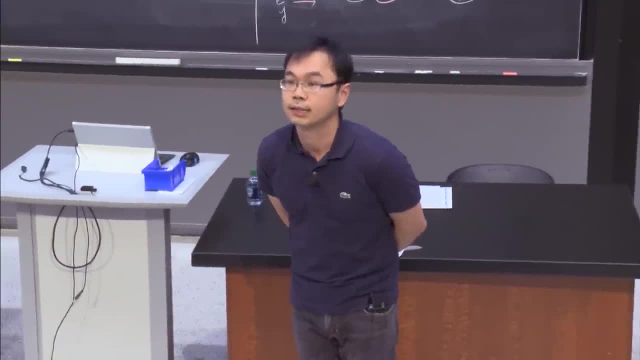 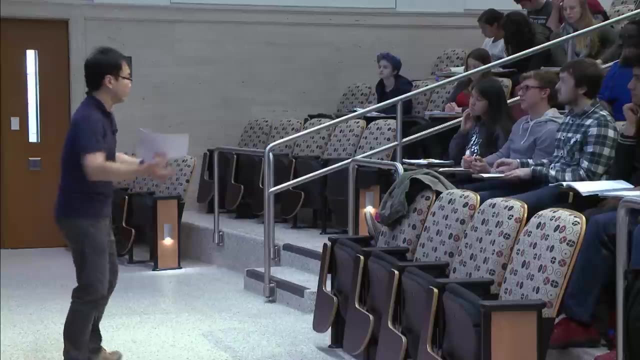 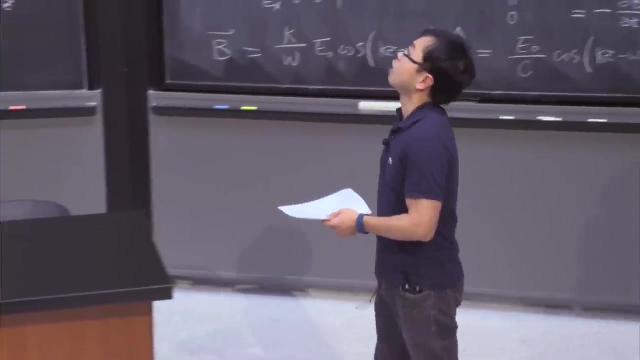 OK, That means all the little charges inside the conductor can move freely. So if they move they don't actually have any energy. OK, They can move around. All the electrons inside the conductor can be moved freely without causing anything. OK. 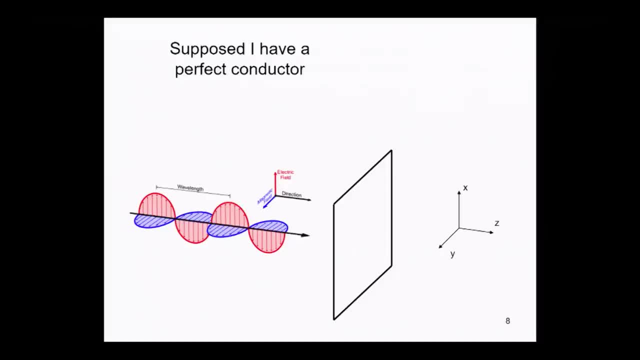 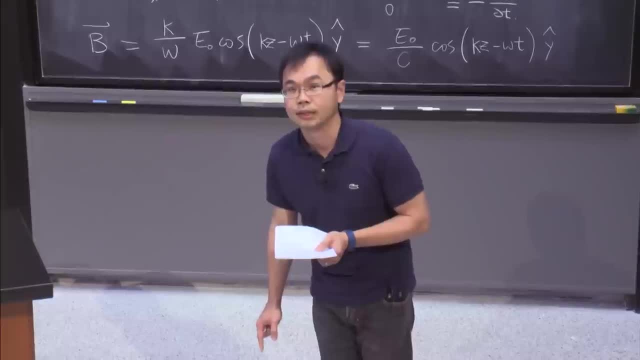 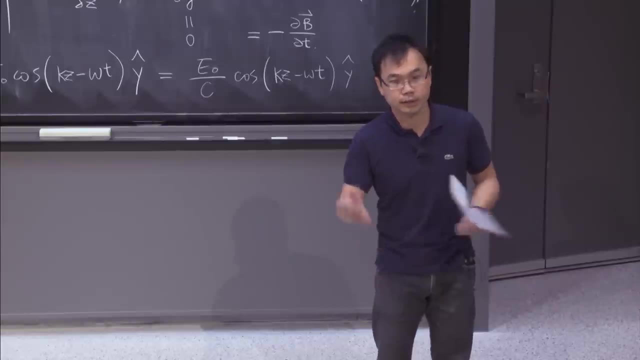 Without any energy dissipation. So that's actually what I mean by perfect conductor. OK, What do I mean by a very busy system? That means whenever there are any distortions on the electric field. Let's say there's an electric field approaching. 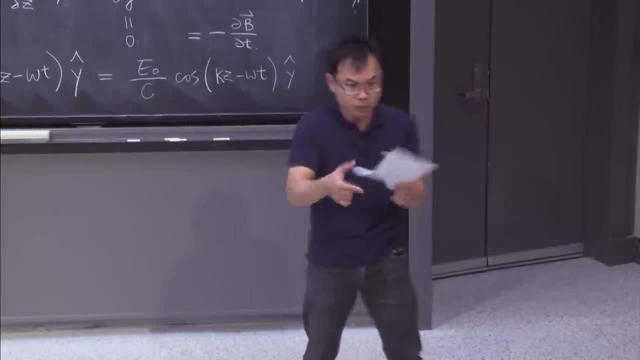 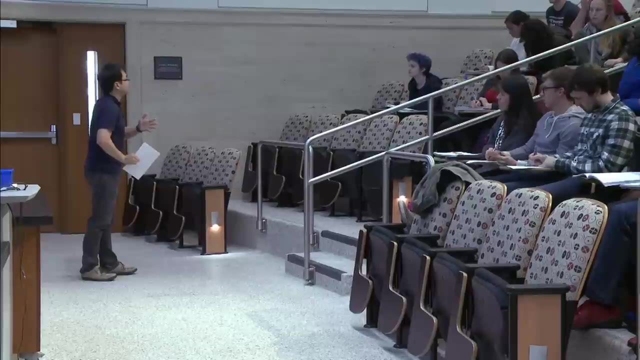 to this conductor. What is going to happen is that this conductor will ooh this electric field So I have to move some of my electrons. Then it's going to cancel all the electric field inside the conductor Right, Because it costs nothing. 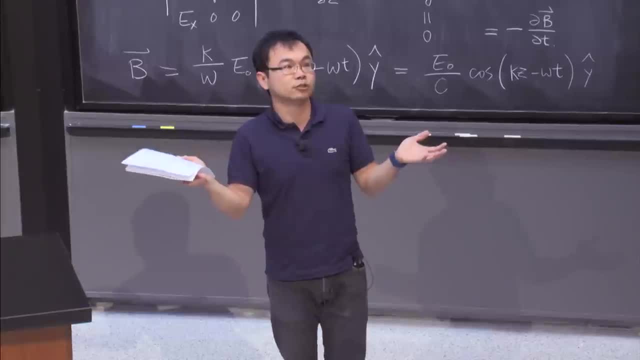 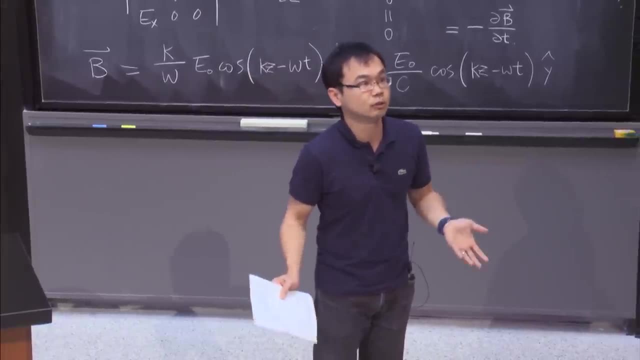 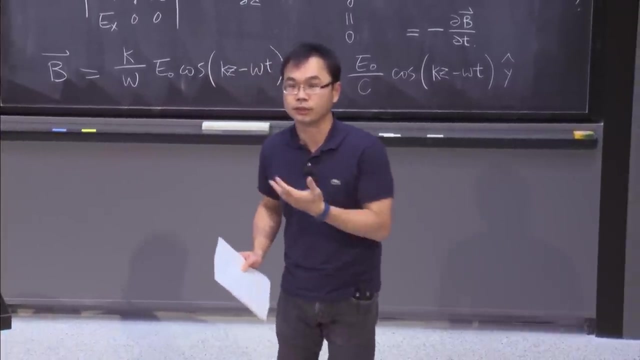 Right. So it will really fast react to this change in the electric field and really carefully arrange all the electrons so that the electric field is canceled. Otherwise all those electrons will continue to move around. OK, Until this happens, this cancellation happens. 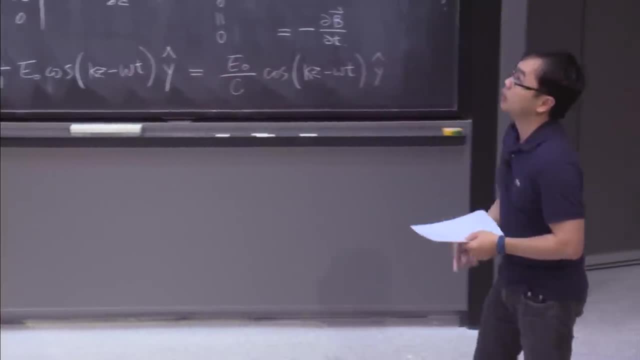 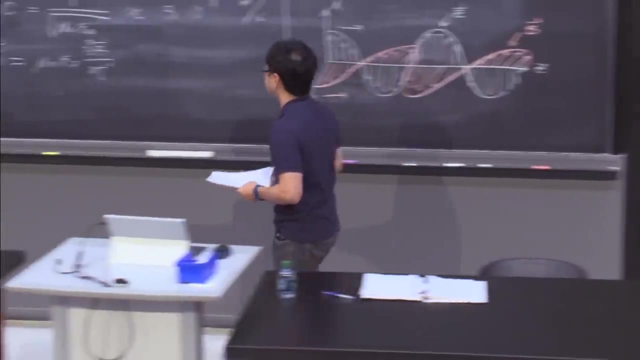 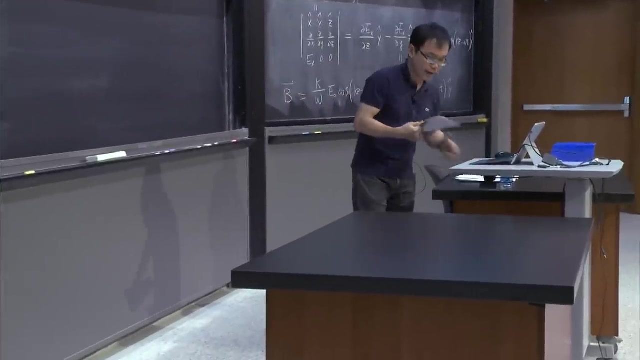 OK, So that's actually what I mean by a busy world and what I mean by a perfect conductor. OK, If I put this conductor into the game, what is going to happen? What is going to happen is that, if I consider a situation, 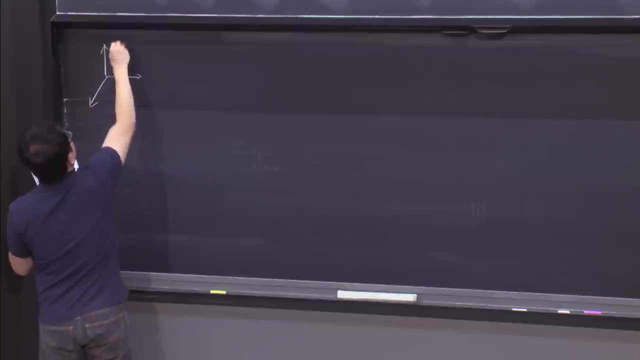 if I have my axis defined here, which is pointing up to be the x-axis, pointing to the right, to the z-axis pointing toward u is actually the y-axis. OK, So I can now again take the plane wave which I started with. 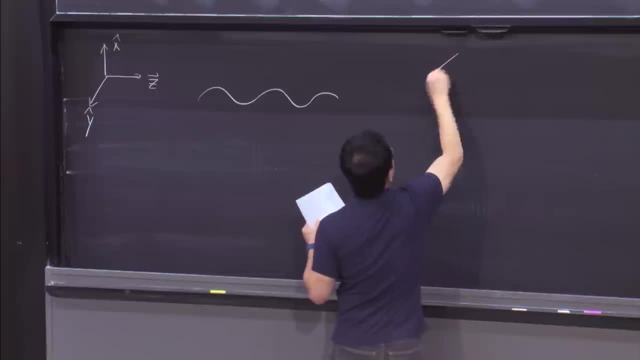 OK, There will be a plane wave like this And it's going to work a piece of a perfect conductor. What is going to happen is that, as I actually explained before, there are many charges over the place. They are going to quickly rearrange all those charges. 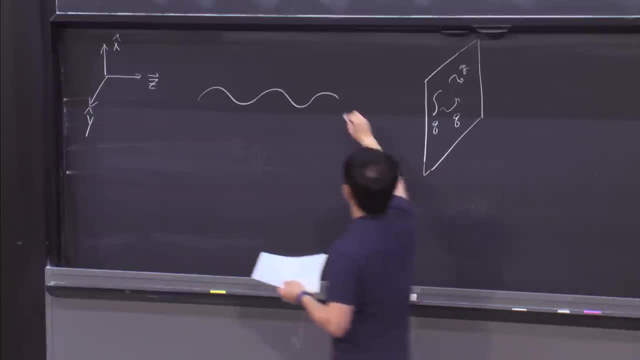 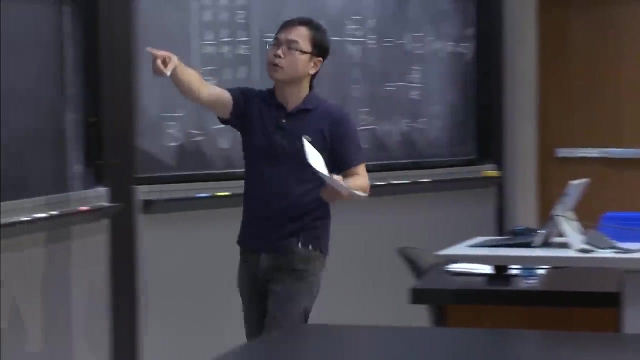 to cancel the electric field, Right? So if you have a plane wave going toward the perfect conductor and the surface of the perfect conductor, the electric field will become zero, Right, OK, So if I have one plane wave, it cannot be. 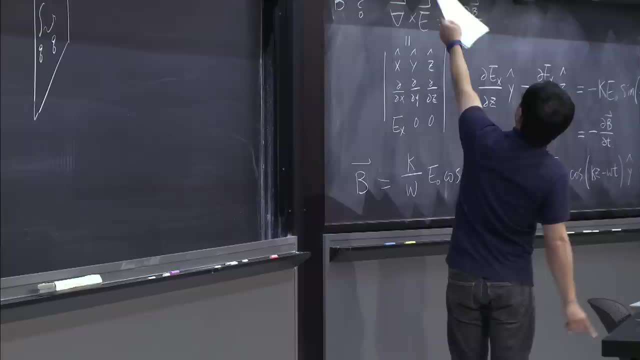 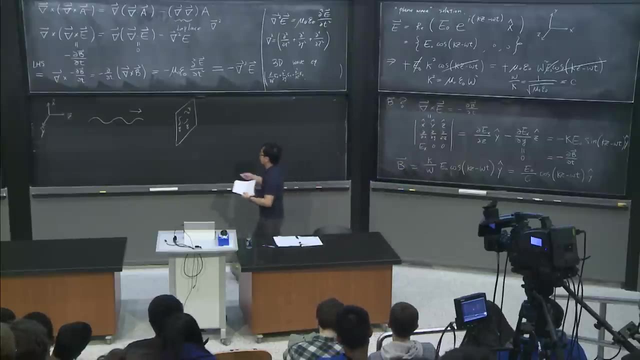 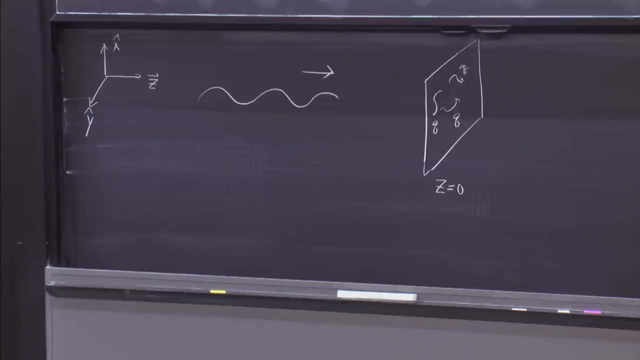 the magnitude cannot be equal to zero, Right, Because I know the functional form. I know that the functional form of the electric field is E0, cosine, kz minus omega t. Right, If I place this perfect conductor at z equal to zero, then I can evaluate the electric field. 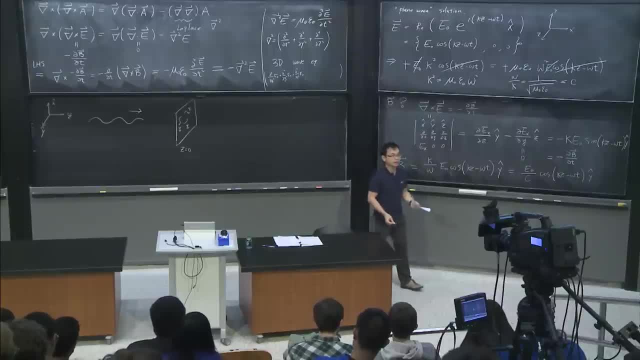 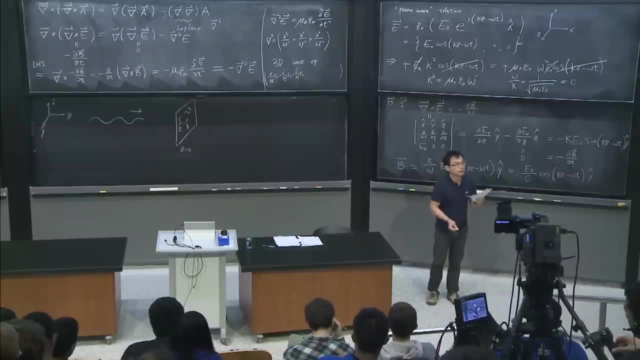 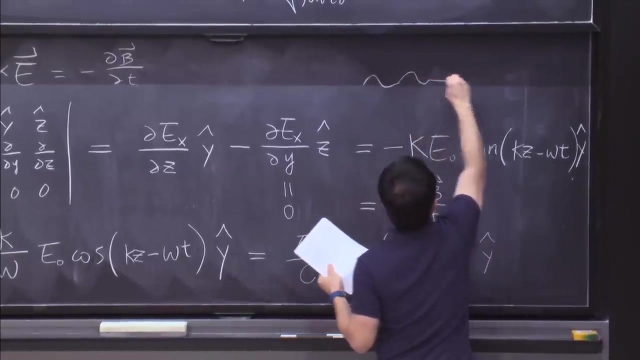 It's not equal to zero, Right, Because it's actually equal to E0 cosine minus omega t, Right? So what can I do to cancel the electric field? This is actually very similar to the situation when you have a progressing wave on the string hitting a wall. 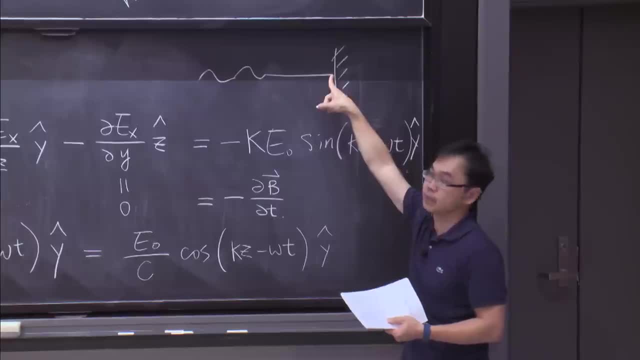 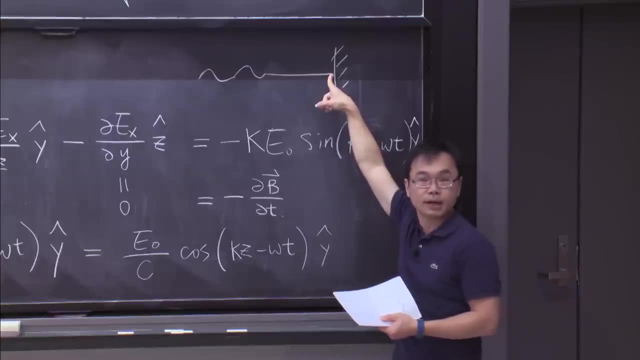 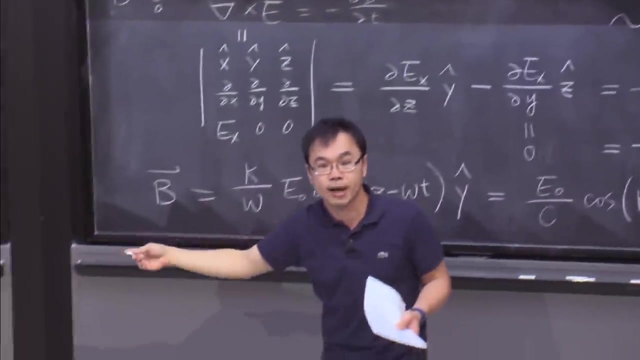 Right, Because the magnitude of the string- OK with respect to the equilibrium position, is actually equal to zero, Right? That's actually what we have learned in the last few lectures And this is actually exactly the same situation. Right, You have a progressing wave. 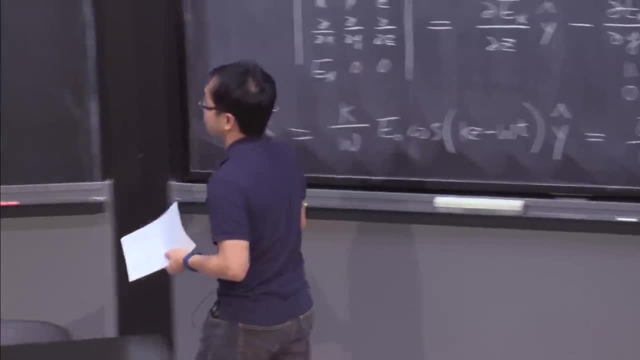 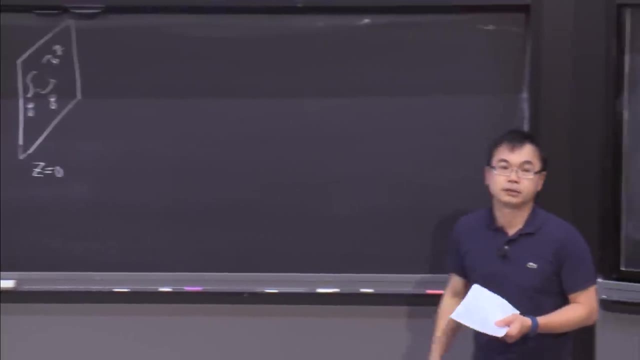 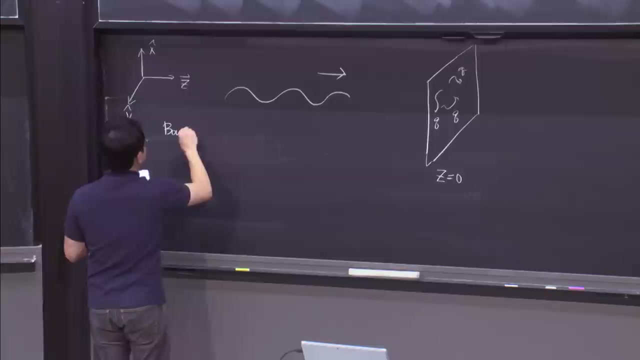 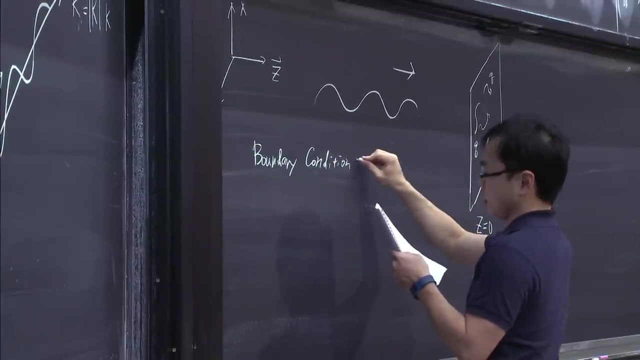 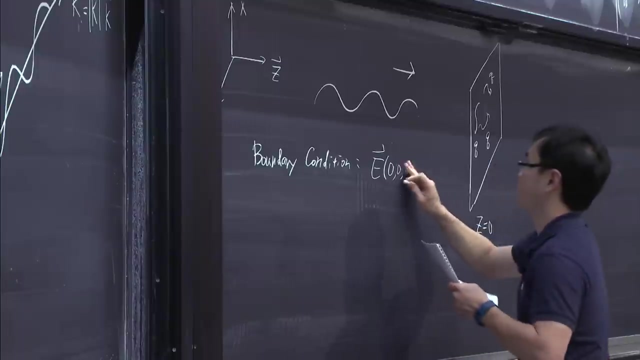 And there is some kind of boundary, which is actually when this progressing plane wave encounters this perfect conductor. There, the electric field, the boundary condition has to be. E, is actually 0, 0, 0,. sorry, Exy0,. 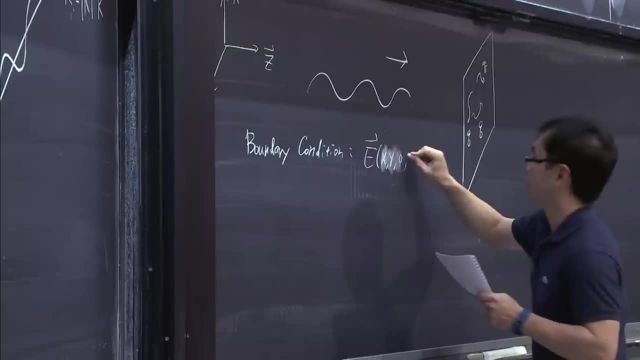 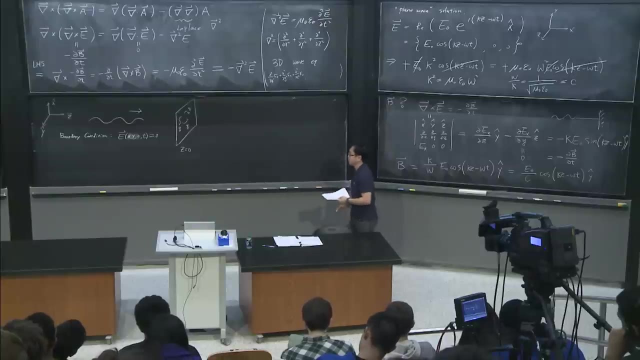 which is actually the position of the perfect conductor as a function of time, will be equal to 0.. OK, And then we have zero electric field. OK, So that means there must be what kind of wave? There must be a refractive wave, right. 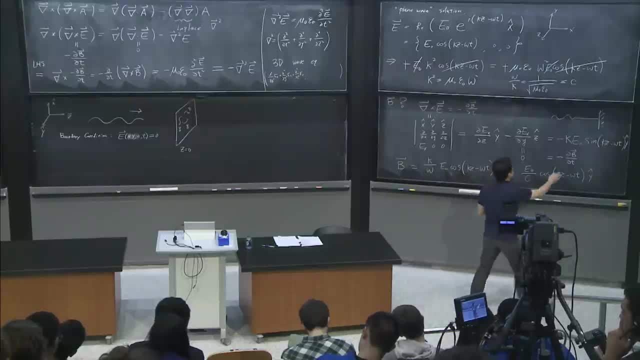 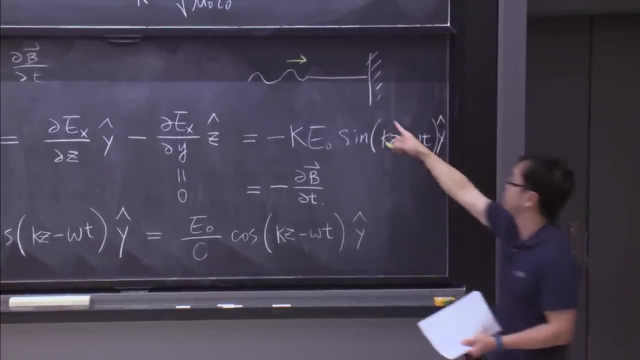 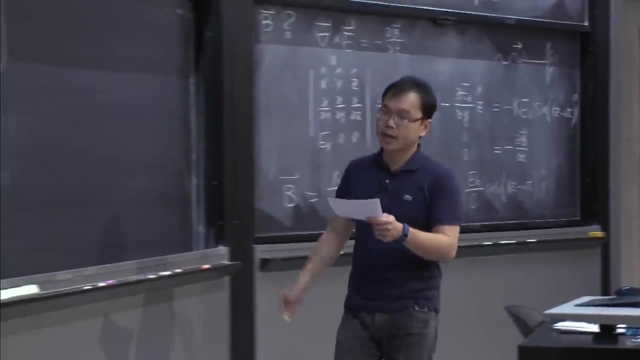 because of the presence of the perfect conductor Right. It's actually similar to the situation which we discussed: There is a progressing wave hitting the wall And, on this string wall system, there is a progressive wave coming out of it. OK, So therefore, what we are expecting. 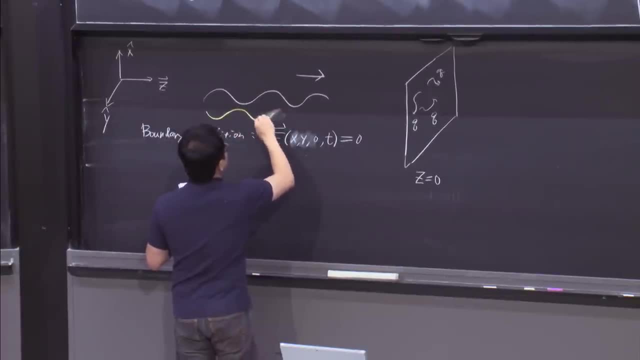 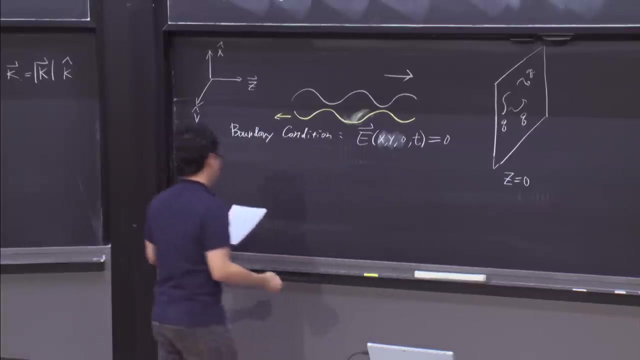 is some kind of refractive wave which actually cancel the magnitude of the electric field at z equal to 0.. OK, And this progressing wave is going to the left-hand side direction. OK, So now I can actually write down the incident wave. 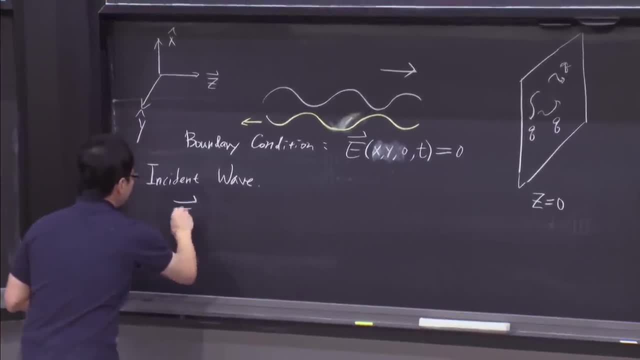 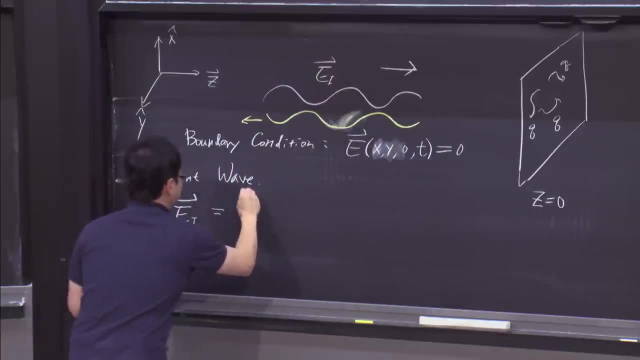 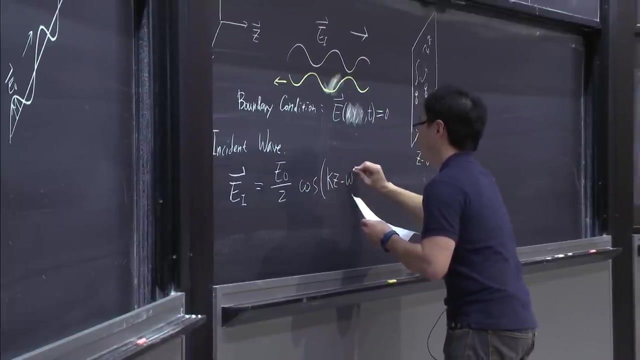 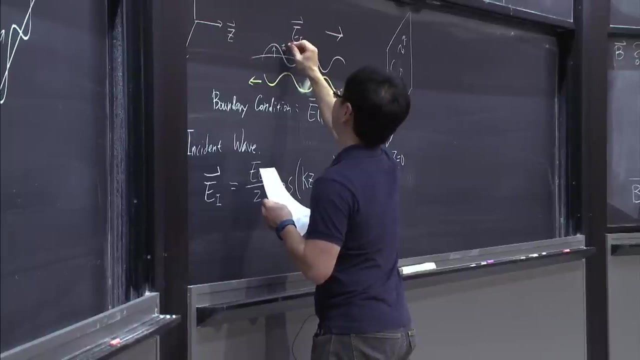 OK, This is an expression. The incident wave. I call it Ei. OK, This is Ei. It's expressed as E0 over 2 cosine kz minus omega t. This is actually what I put into the system. The magnitude is E0 over 2.. 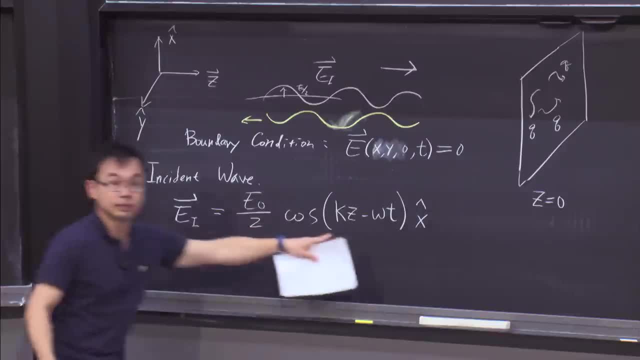 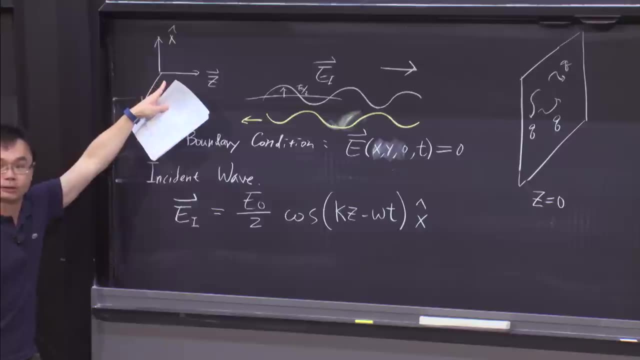 And it's actually propagating the z direction, as you can see from here, And the direction of the electric field is in the x direction. OK, And of course the E field will have a corresponding magnetic field, which is actually- you can actually write it down directly: 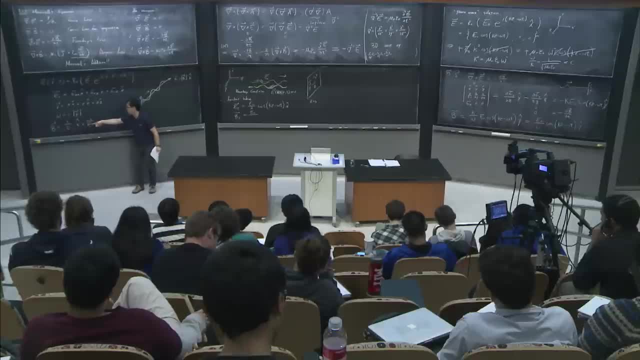 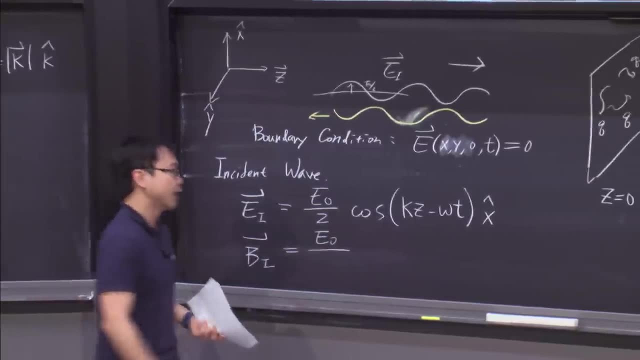 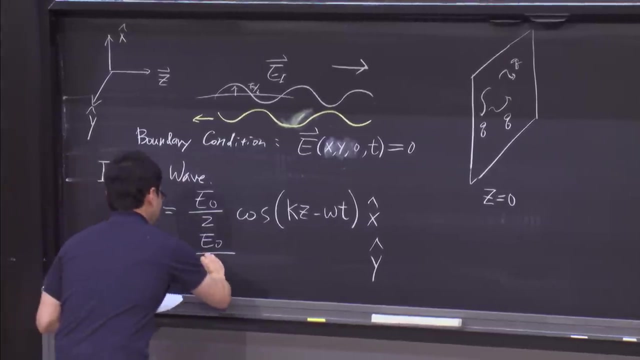 using this formula, Right, B equal to 1 over c, k equals E, k. here is z Right. Therefore, you can quickly evaluate and conclude that the magnetic field must be in the y direction And the magnitude of the magnetic field. 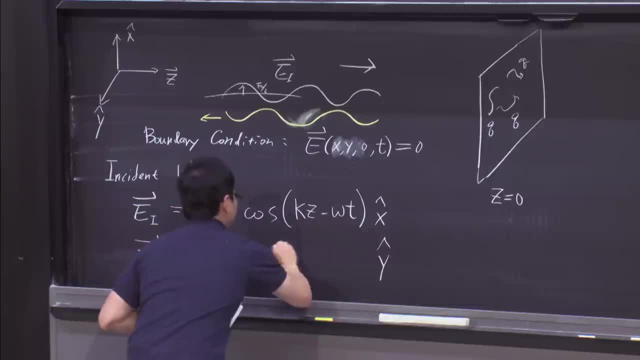 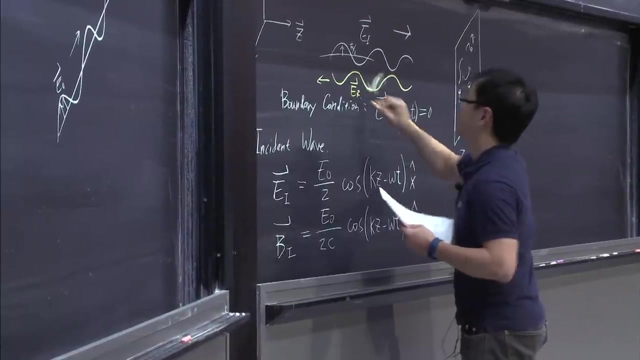 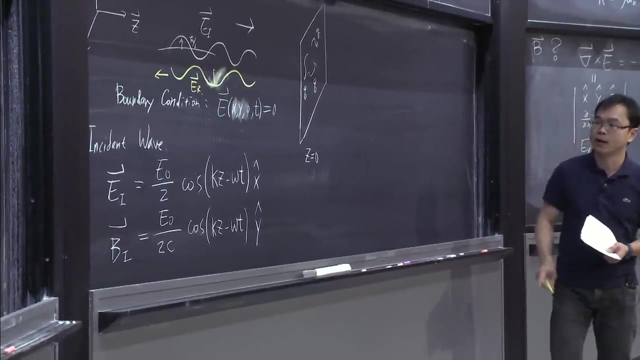 will be E0 divided by 2c, cosine kz minus omega t. OK, So that is actually the incident wave And of course I also need, as I discussed, there must be a refractive wave, And that is R, which actually cancels the electric field. 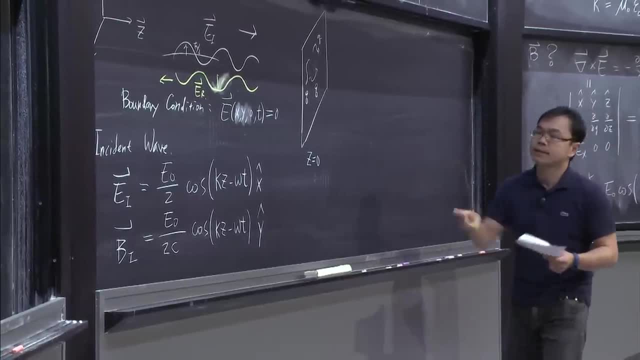 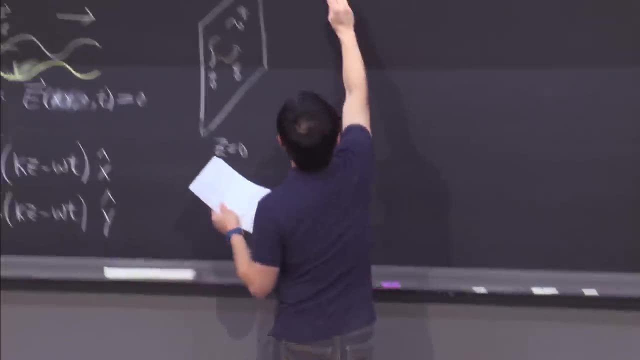 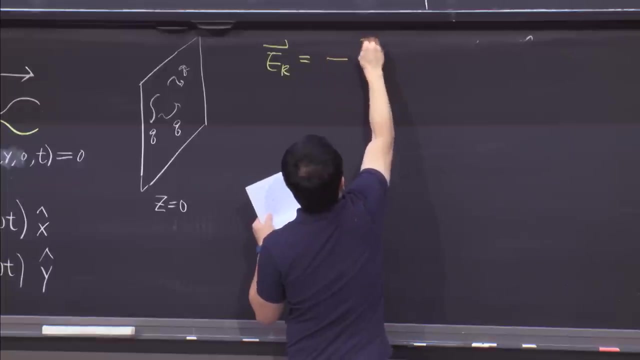 at z equal to 0.. OK, If that cancels the incident wave, that means the magnitude must be in the opposite direction of the incident wave, Right? Therefore I can quickly write down what will be the resulting refractive wave: that will be equal to minus E0 over 2 cosine. 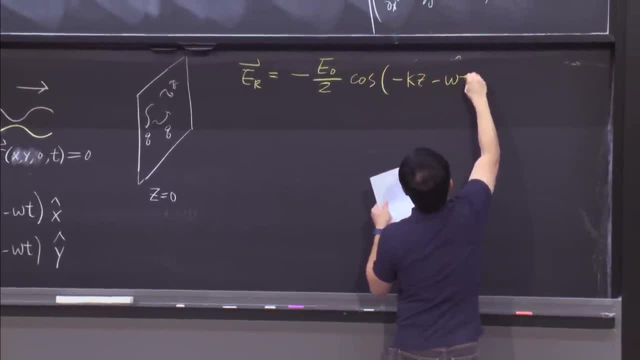 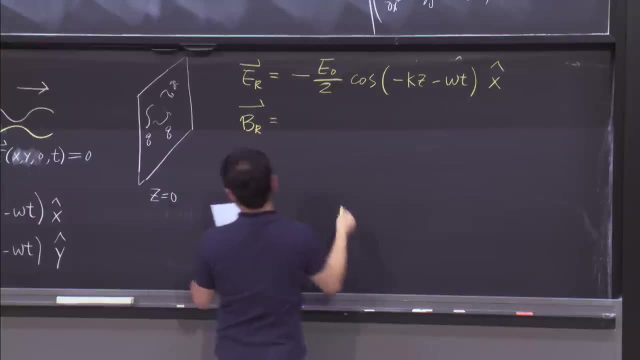 minus kz, minus omega t in the x direction, And then the corresponding B field. I can also write it down using exactly the same formula, Right? And basically what I conclude is that this will be equal to E0 over 2c, cosine minus kz. 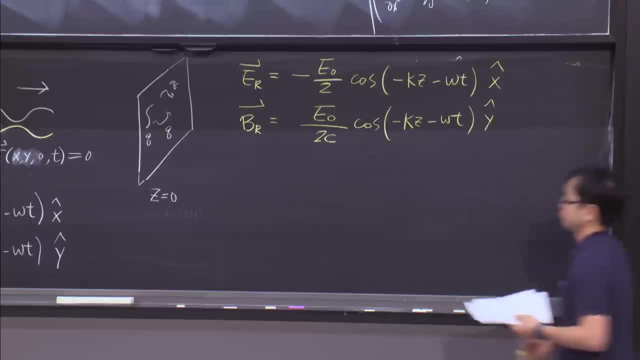 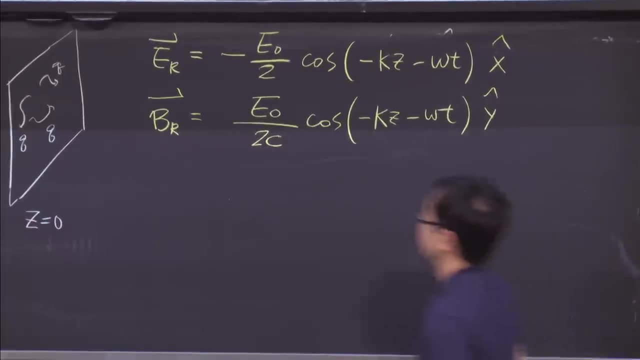 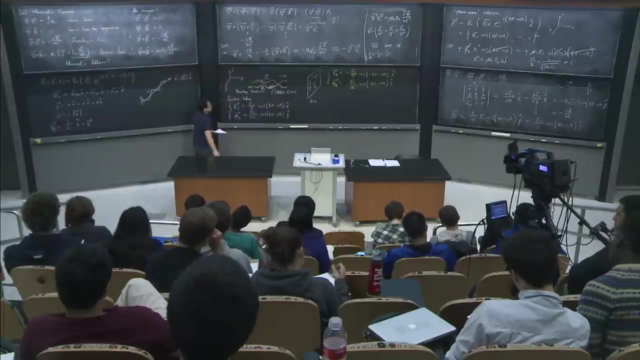 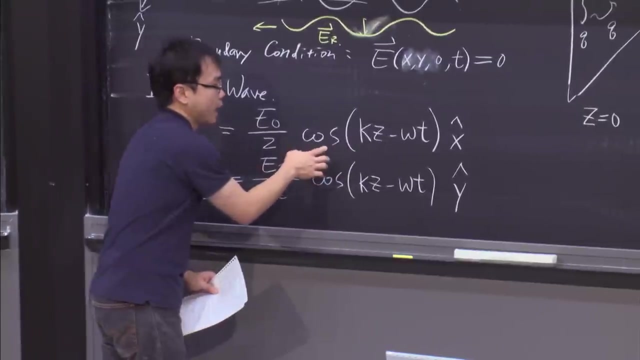 minus omega t in the y direction. OK, So you can actually check this expression after the lecture. So now I would like to check what will be the magnitude of the electric field at z equal to 0.. So basically, at z equal to 0, you. 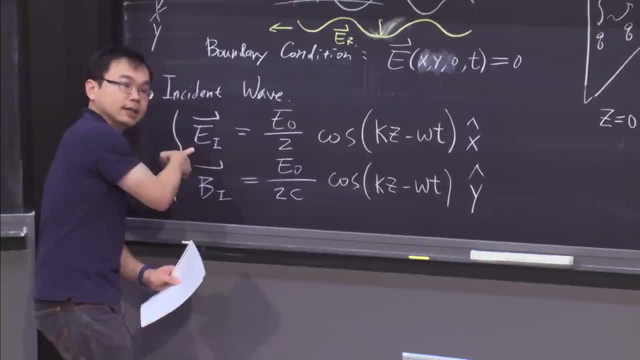 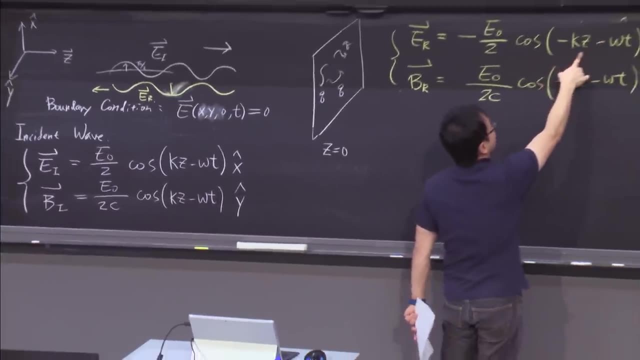 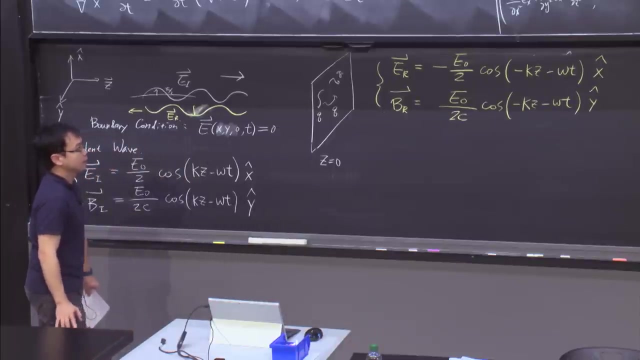 have something which is proportional to cosine minus omega t for the incident wave, And then the magnitude is E0 over 2.. And if you evaluate z equal to 0, basically you get minus E0 over 2, cosine minus omega t. Therefore, they really cancel and give you. 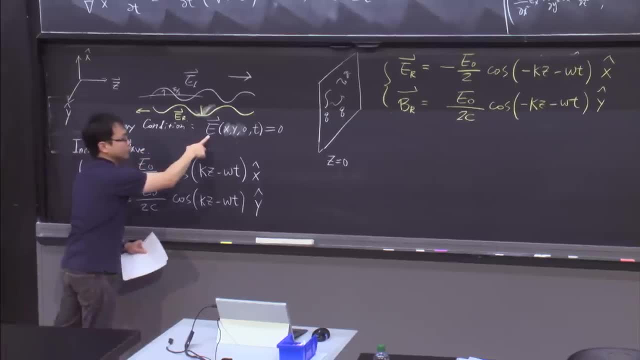 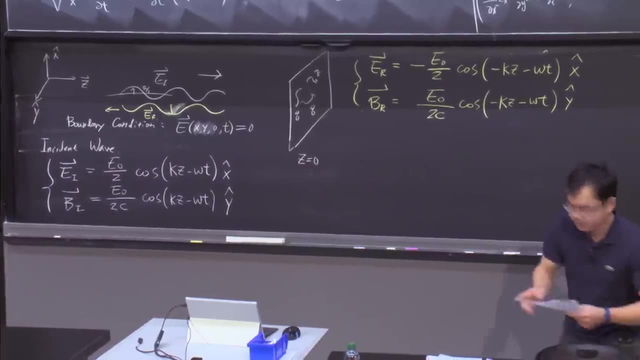 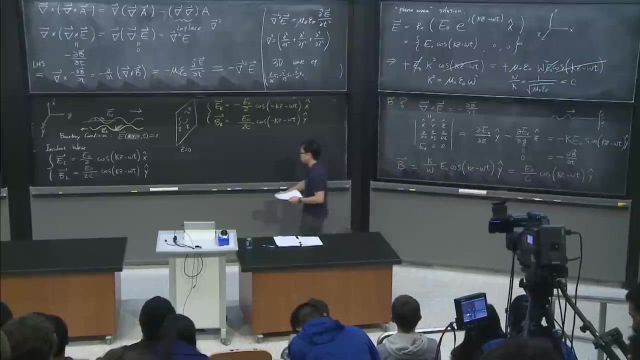 the desired boundary condition, which is actually E equal to 0 at the surface of the perfect conductor. OK, So that's very nice, And this is actually the physics which we already learned from this string wall system. OK, So what I can do now is to calculate. 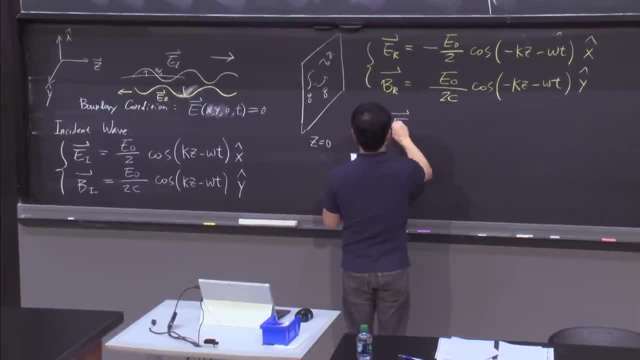 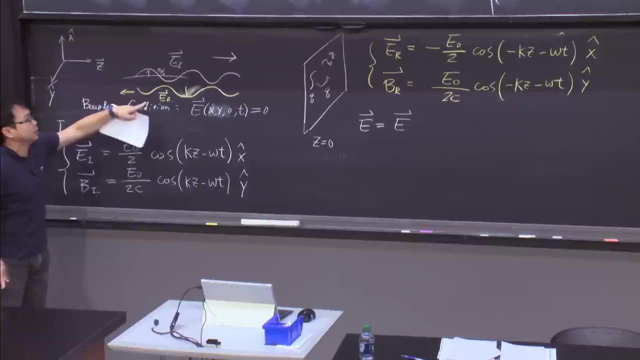 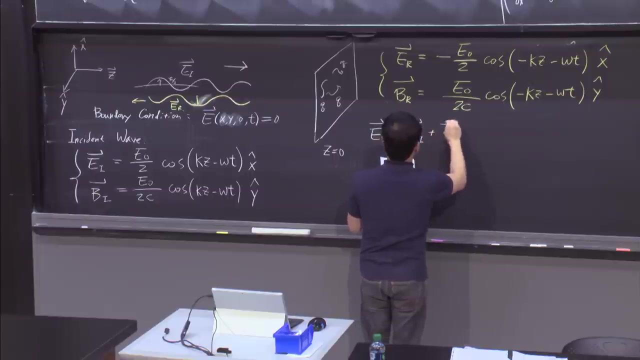 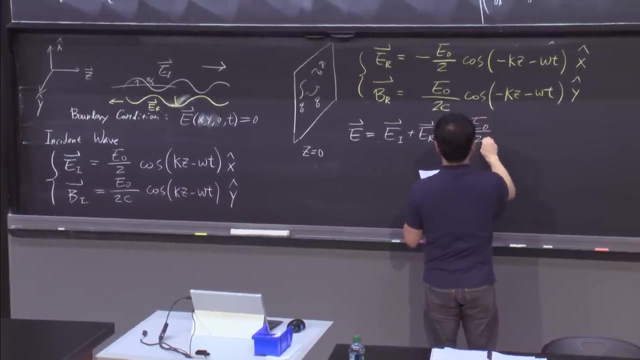 the total electric field. If I add them together, basically I will get E total electric field, which is actually overlapping the incident and the refractive wave. What I am going to get is Ei plus Er, OK, And basically what I get is E0 over 2.. 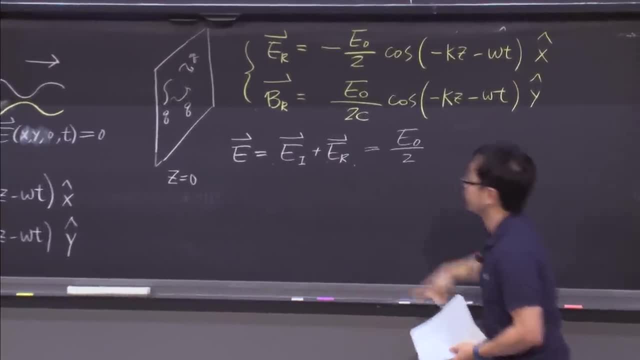 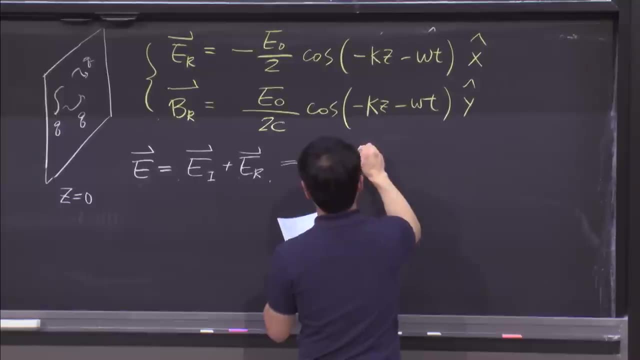 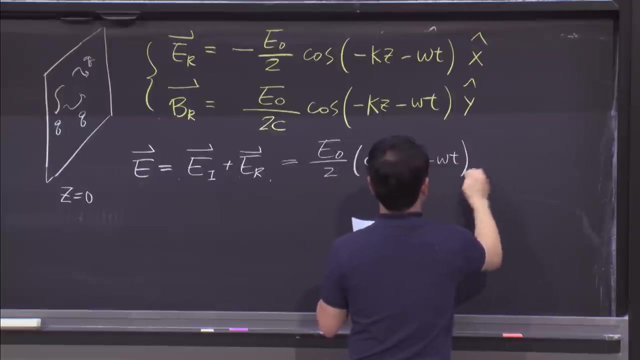 OK, Because the incident wave and the refractive wave, the electric field, is always in the x direction. Therefore, I only need to take care of the x direction. So basically, I have cosine kz minus omega t minus, because there's a minus sign here- minus cosine minus kz. 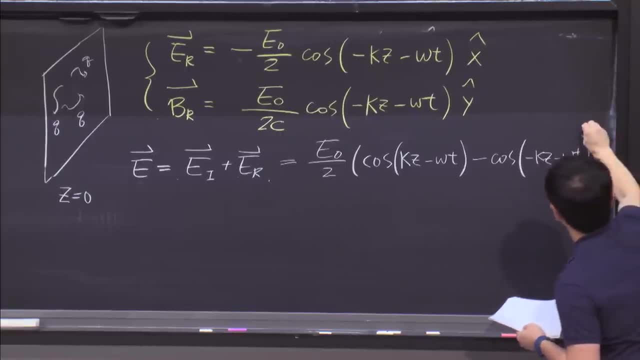 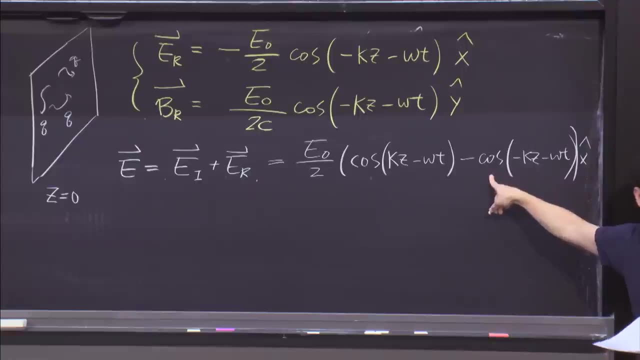 minus omega t in the x direction, And this should be here. And of course, this is a cosine minus cosine, right? So we have all the formulas I want from, for example, Wikipedia or from your textbook, right? So you can actually calculate this. 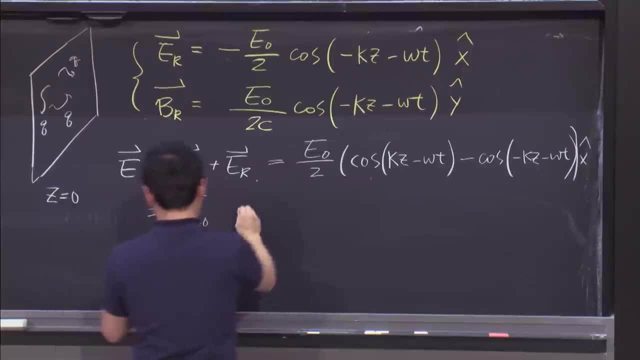 rewrite this expression to be E0 sine omega, t sine kz, And this is actually in the x direction. OK, Everybody is following. I hope it's not too fast, All right, And of course I can also calculate the corresponding B field, right. 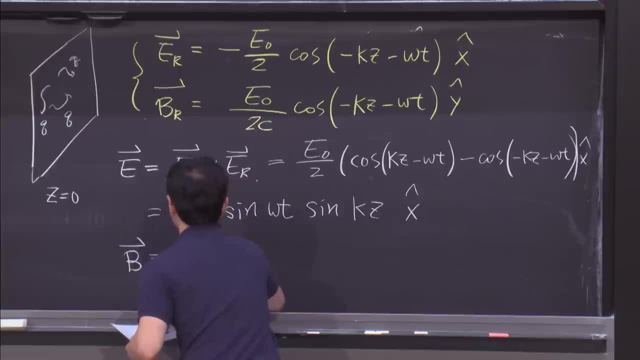 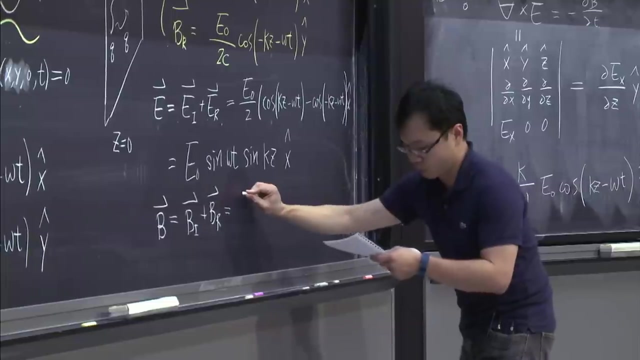 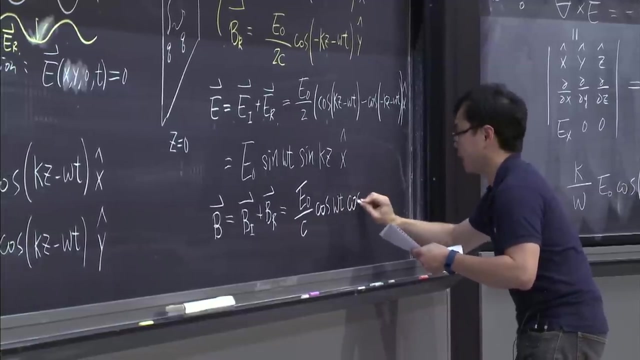 So essentially again exactly the same thing, Vi plus Br, And basically I will skip the step. Basically, you can add this term and that term, OK, And you can conclude that the B field will be equal to E0. over C cosine, omega t, cosine kz. 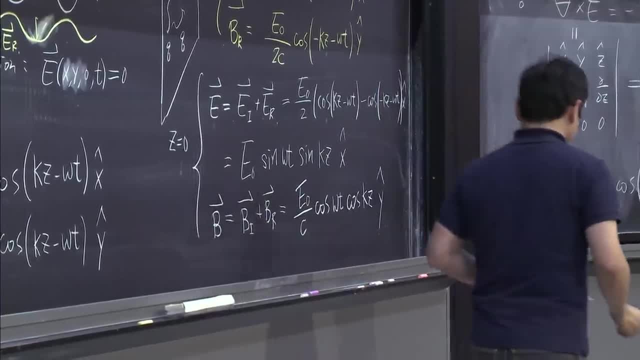 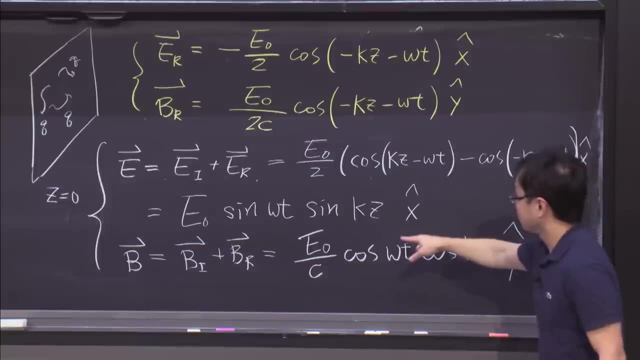 in the y direction. This is actually pretty interesting If you look at this, if you look at this result. I have an electric field which is proportional to E0, sine omega t, sine omega t and sine kz. OK, What does that mean? 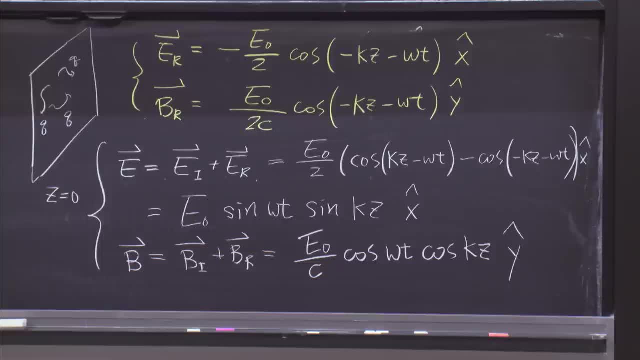 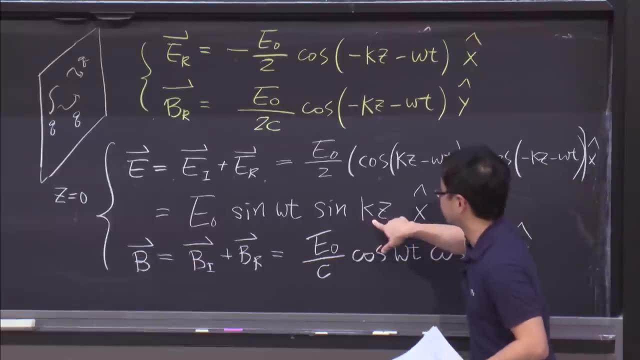 This is a special kind of wave which we learned before. What kind of wave is this? It's a standing wave, right? Because the shape is actually fixed, It's sine kz And the magnitude is actually changing up and down at the angular frequency omega t. 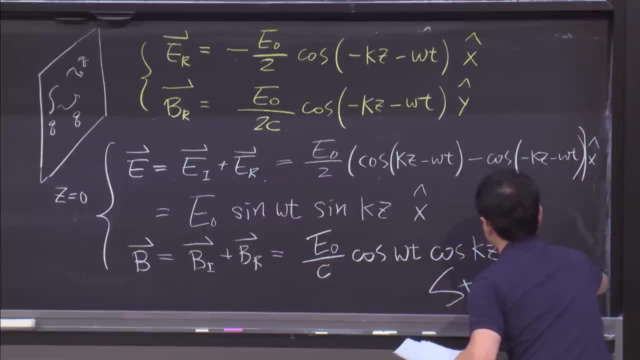 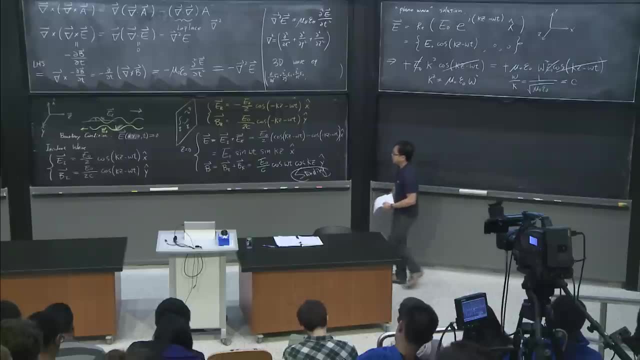 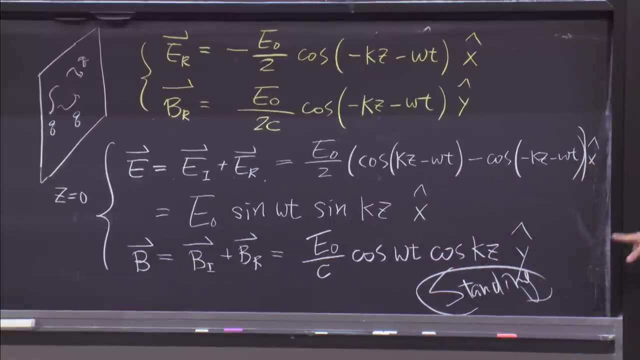 It's a standing wave. Another thing which is really interesting is that if you look at the expression of electric field and the magnetic field, if you compare that one is actually sine sine, The other one is cosine, cosine. OK, That's kind of interesting. 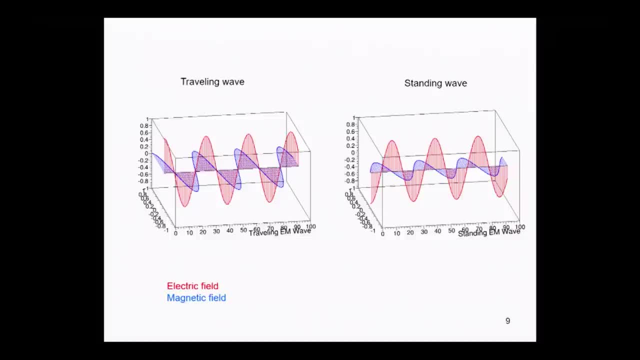 Because this is actually different from what we actually usually learn from the progressing wave solution or traveling wave solution, where the electric field and the magnetic field are in phase Right. There is no phase difference In the case of the superposition of the incident. 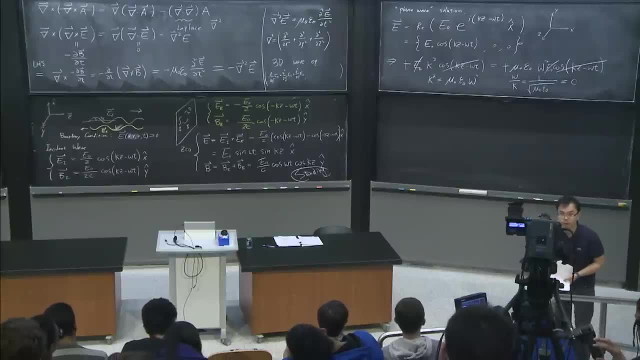 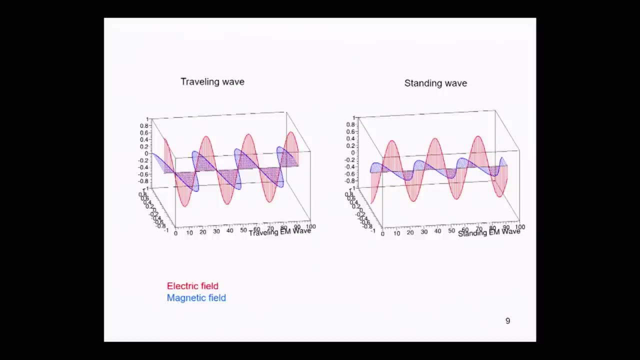 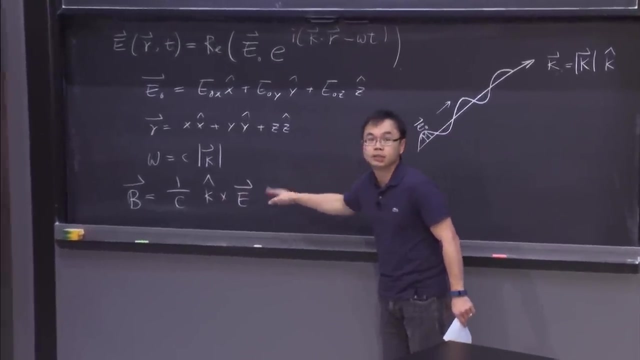 and the refractive wave, the solution of a standing wave. actually, you can see that the phase of the B field and the E field are different. OK, Finally, very important, you see that Look at this expression: B equal to 1 over C, k cross E. This only work. 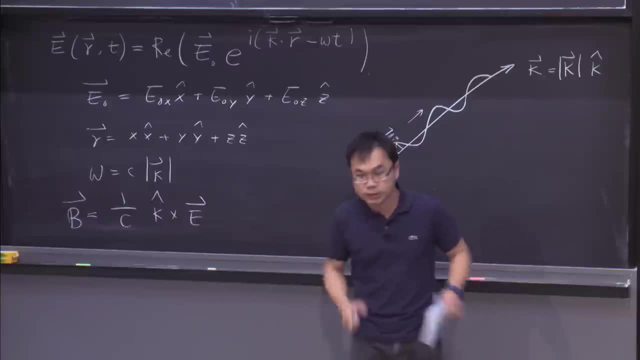 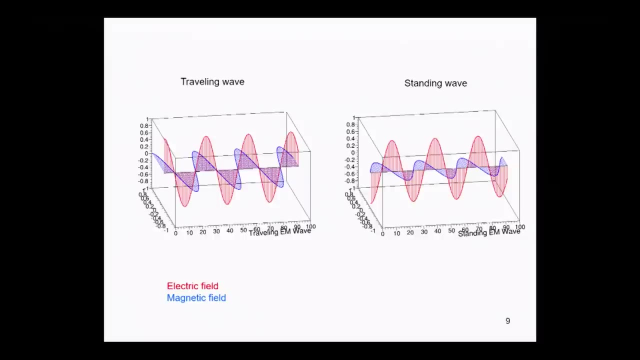 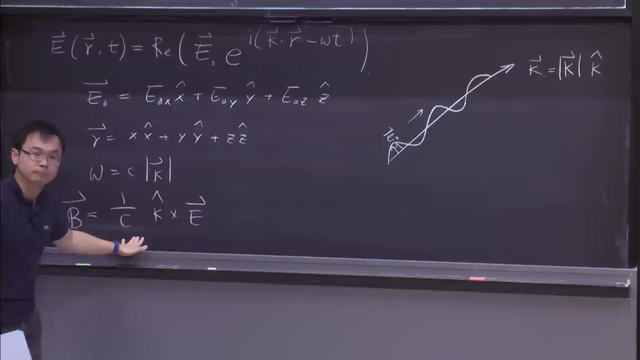 That means this only work for traveling wave Right. Clearly this doesn't work for standing waves. OK, Very important. So don't blindly apply this expression. This is only useful for the traveling wave solution, And you can see a very concrete example here. 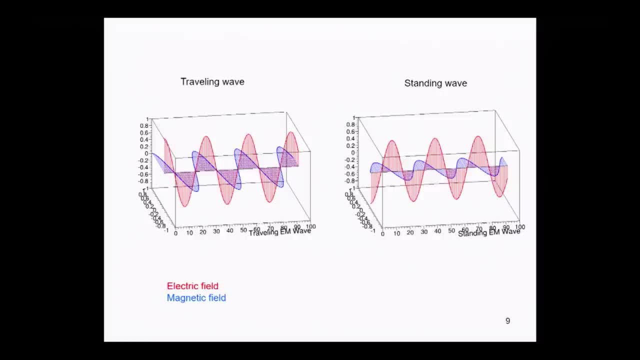 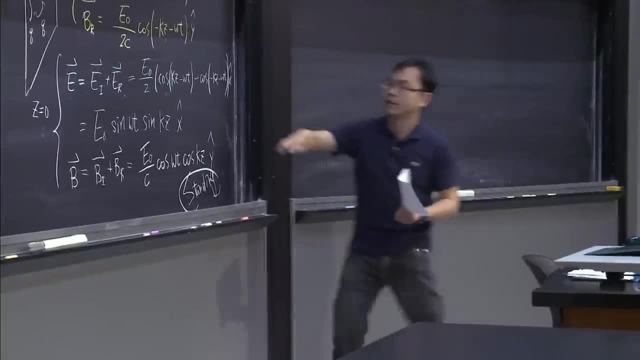 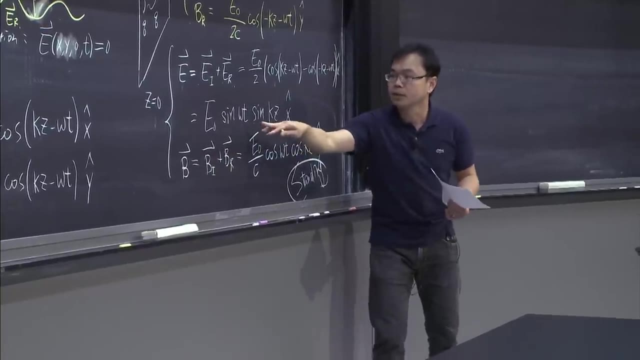 This doesn't work for standing waves, OK. OK, That's kind of interesting. And if you look at this result, you will see that if I don't have magnetic field, OK, I only have the electric field. there will be an instant of time. for example, t equal to 0. 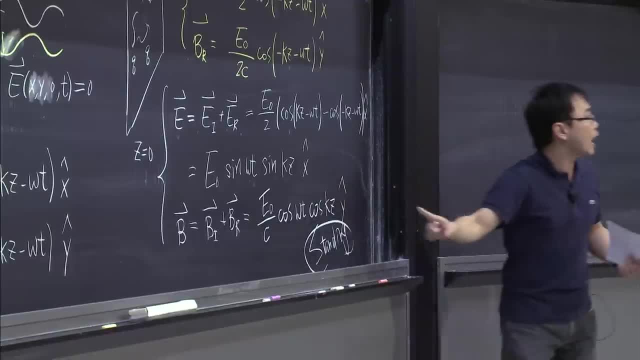 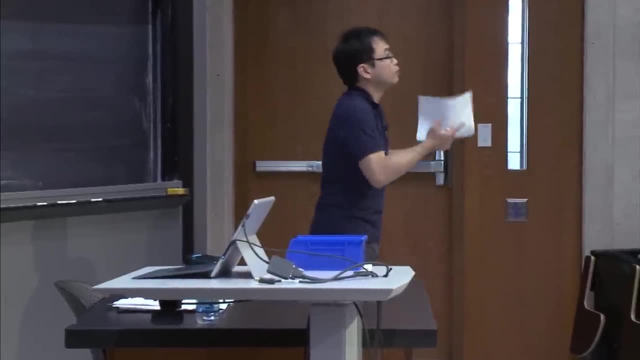 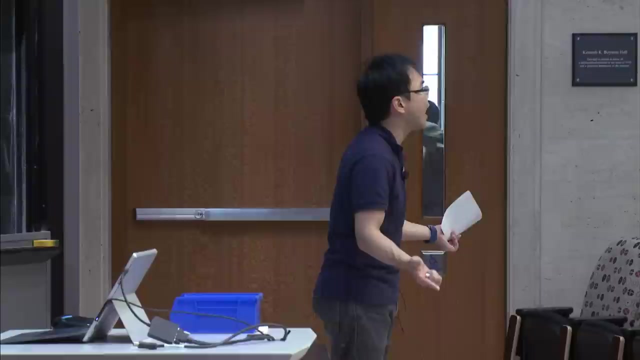 When t is equal to 0, sine is equal to 0. What is going to happen? You will have no electric field. OK, That means electric field completely disappear. Right, Because we are operating this system in vacuum. Right, There's nowhere to hide. 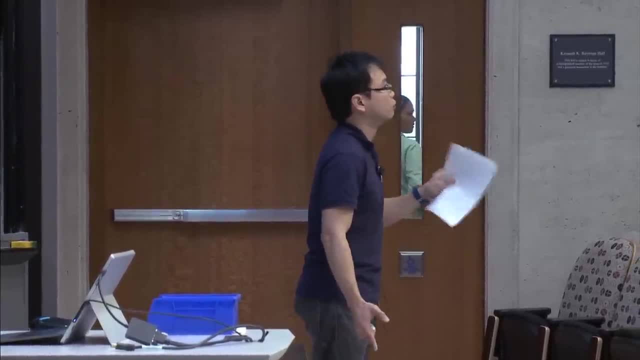 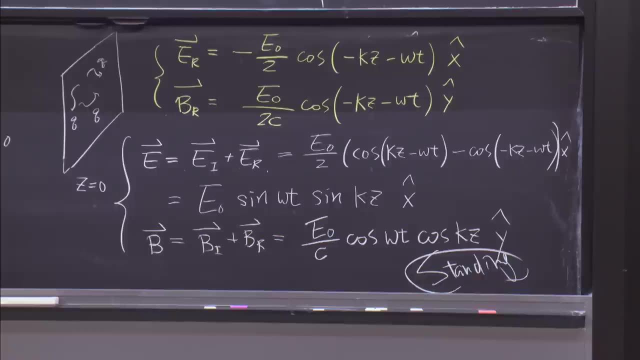 Where is the energy? Right, The energy. Unfortunately, electric field have a very good partner, which is actually B field. OK, All the energy is actually stored in the form of magnetic field. Right, You can see that now magnetic field is reaching the maximum. 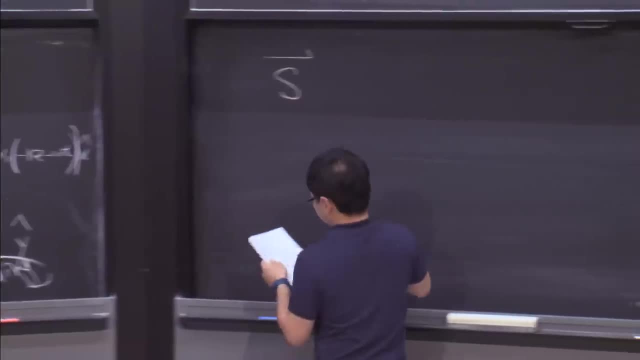 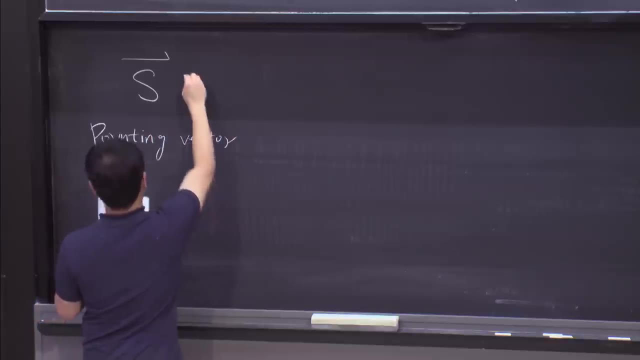 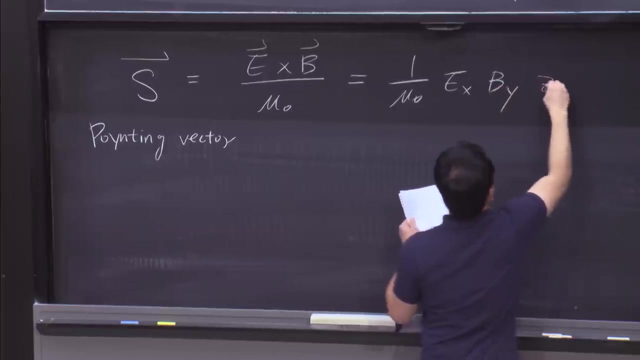 OK, So of course I can now calculate the pointing vector. OK, Pointing vector is E cross B divided by mu 0. And this will be equal to 1 over mu 0, EX BY in the z direction. There is only one term which survives. 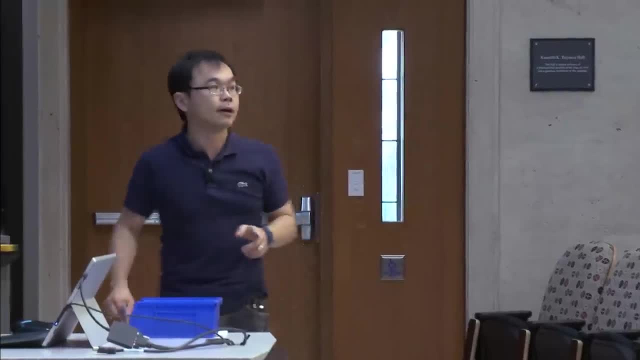 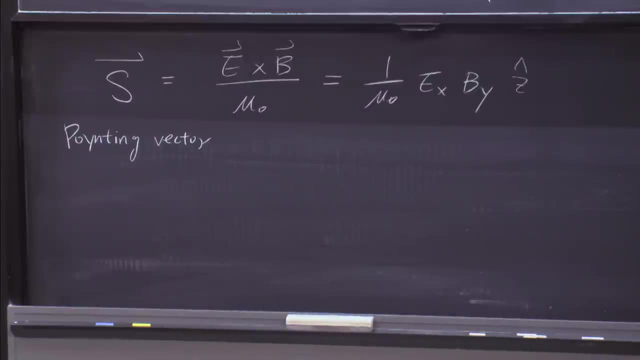 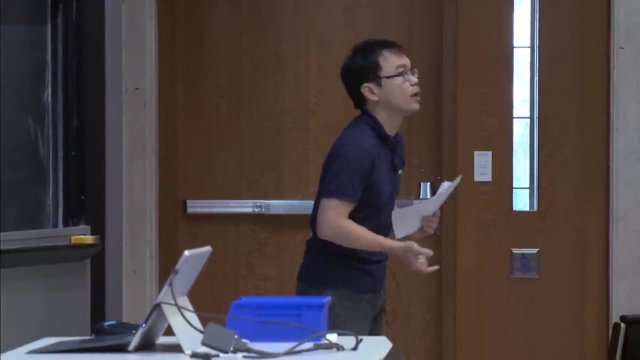 So pointing vector is not pointing vector. OK, It's not pointing around. OK, There's a gentleman who is called Pointing And he has a vector. Pointing vector is a directional energy flux. It's a directional energy flux or the rate. 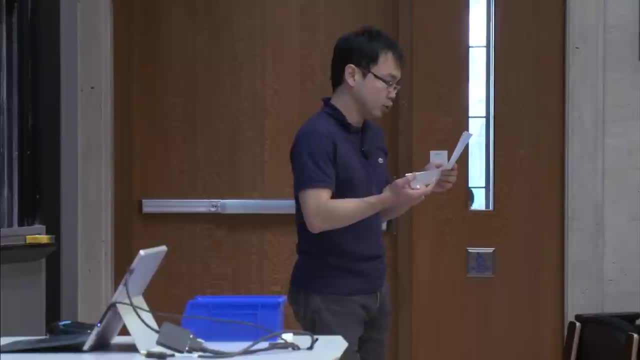 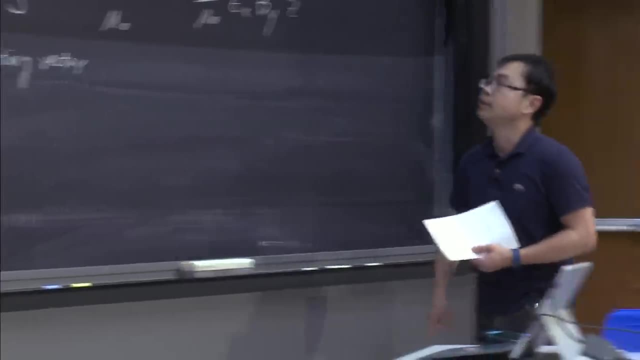 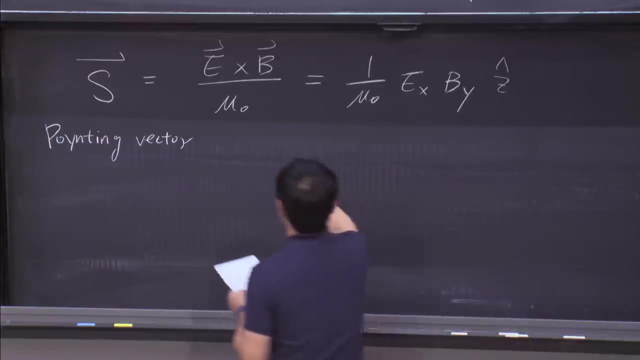 of energy transfer per unit area. OK, So that is actually the meaning of pointing vector And its magnitude is proportional to E cross B divided by mu 0.. OK, So now I can calculate that If I have the EX and BY, then I can calculate. 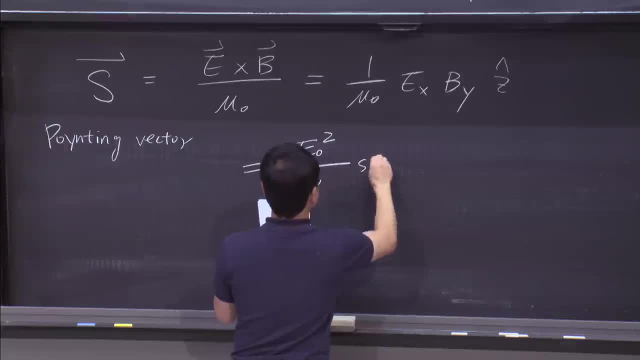 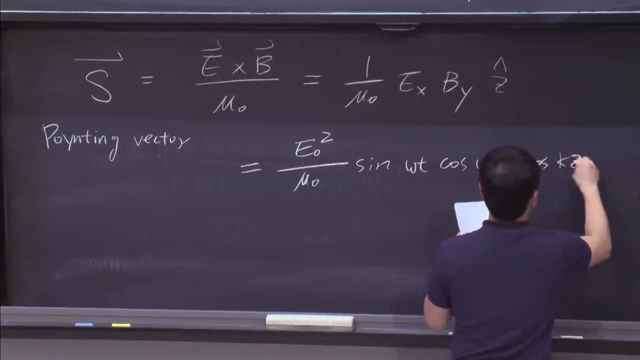 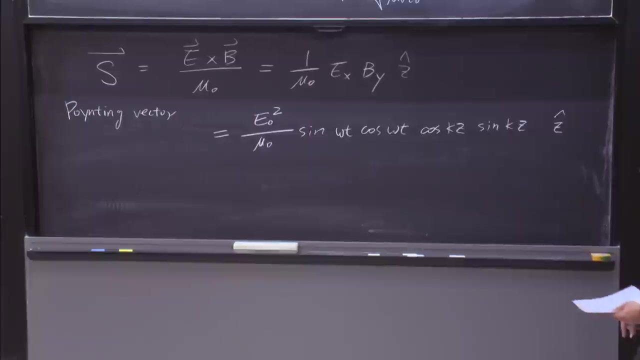 that would be equal to E0 squared over mu 0 sine omega t cosine, omega t cosine kz sine kz in the z direction Right, Because I have x cross y And I'm going to get the z direction Right, OK, And I can simplify this. 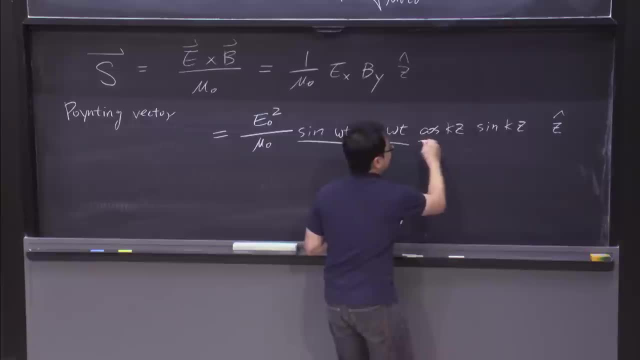 So I have sine cosine and I also have cosine sine. Basically you can simplify this expression and get E0 squared, divided by 4, mu, 0, c sine 2 omega, t sine 2 kz in the z direction. OK, So you can see that the directional energy flux. 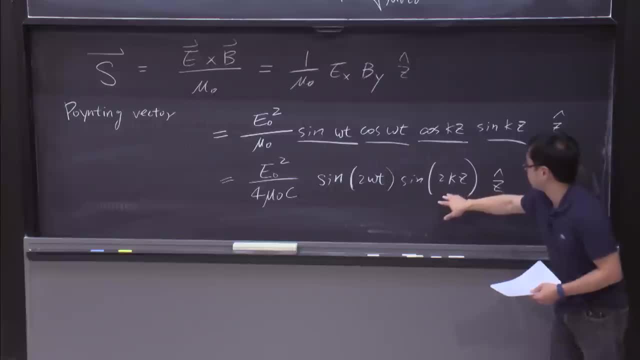 it's in the z direction, OK, And it has a vector. It has a wave number, two times of the original wave number, And it's actually going up and down two times of the speed of the oscillation of the original electromagnetic wave. 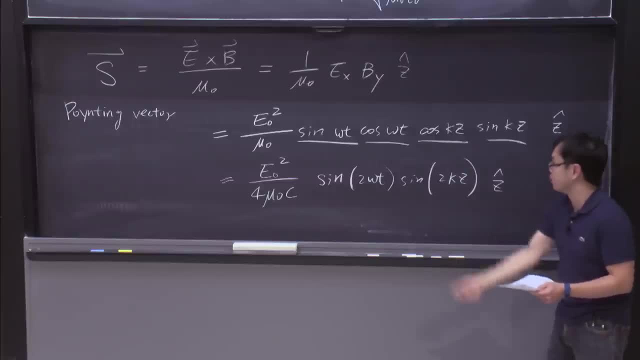 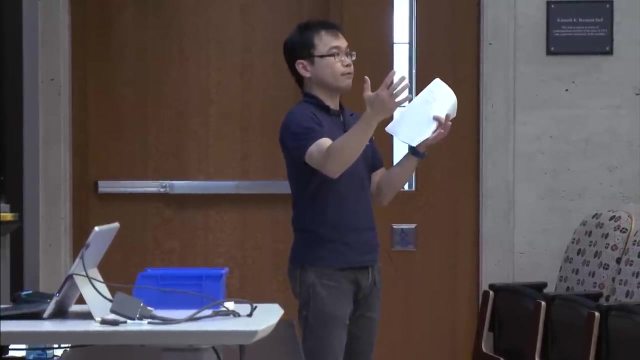 OK, And this energy is actually vibrating up and down And the shape of this energy transfer pointing vector is actually a sine wave. OK, So that is actually exactly how the microwave actually works, Right? So basically, what we are doing is to generate microwave inside your device. 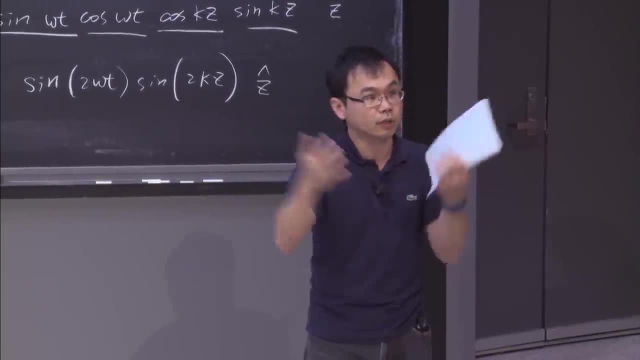 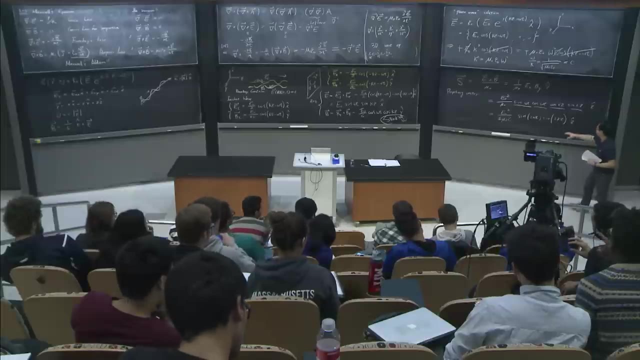 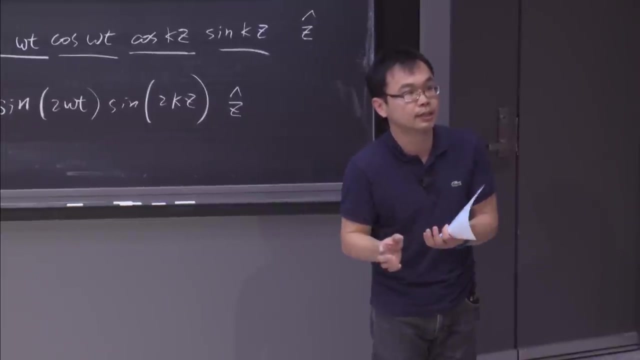 And in the oven. this microwave is actually bouncing back and forth because you have metal walls which, as you can see, bounce the electromagnetic field back and forth And it really can cook the food by vibrating the molecules inside the food back and forth. 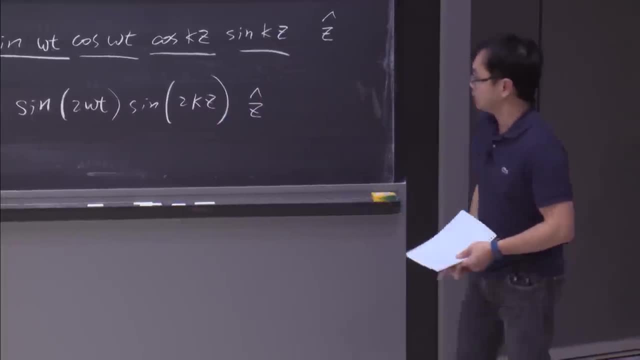 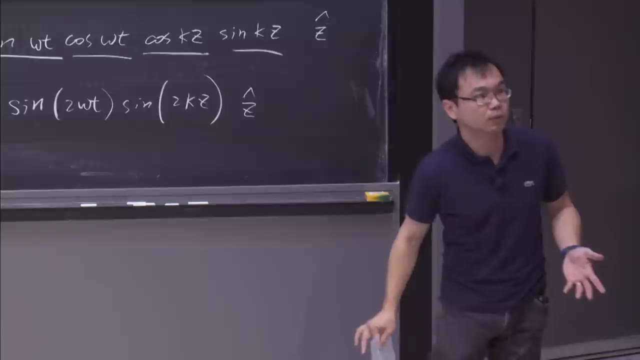 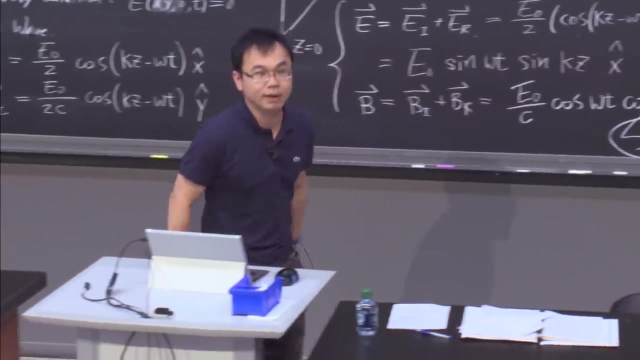 Right. So, as you can see, the magnitude of the pointing vector is actually oscillating up and down. That actually causes additional vibration And that heats up the food. So after this lecture, you will be able to say proudly that you understand the physics of microwave oven.